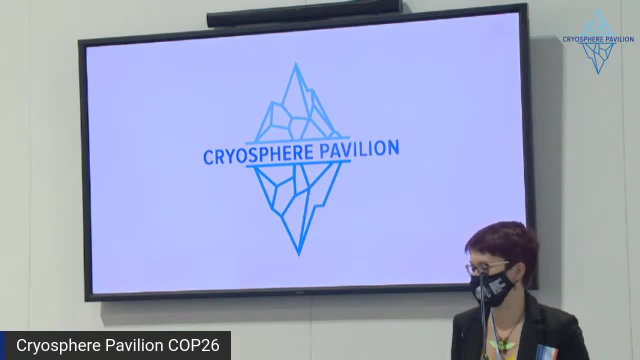 to the Cryosphere Pavilion and to Permaprost Day at the Cryosphere Pavilion. We've got a fantastic session ahead of us looking at committed emissions and intergenerational justice, with a fantastic set of speakers, And I'd like to welcome you to that session. 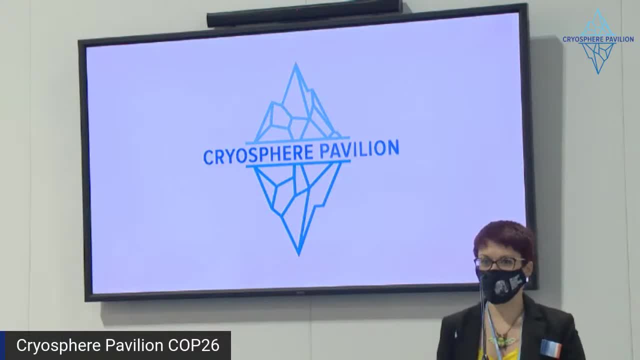 Of course, all of you here in front of me, as well as all of you at our Cryosphere hubs in Stockholm and in Geneva, and, of course, all of you joining online as well, And wherever you're joining from. do feel free to pop your questions into the chat. 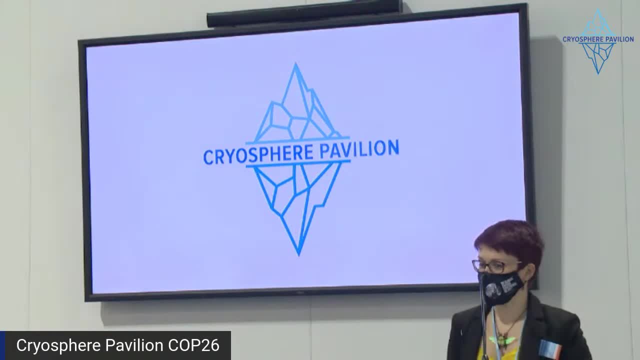 And I'll be happy to answer them online as we go along, and we can come back to those at the end. So, without further ado, I will hand over to our first speaker, Gustav Hugilius, from the Boland Center at Stockholm University. 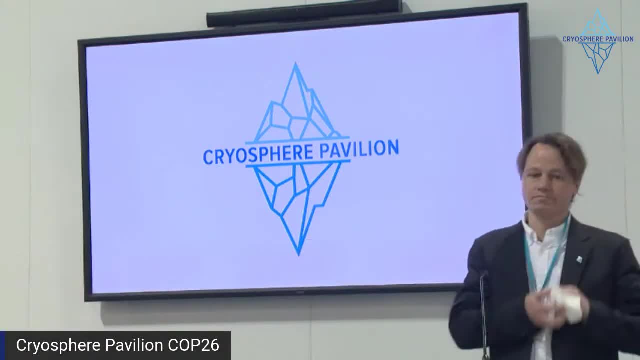 Thank you. Thank you very much, Rachel. So I will wait for my slides to come up. I can start by just giving an overview of the session in general. Thank you very much, Rachel. I will wait for my slides to come up. I can start by just giving an overview of the session in general. 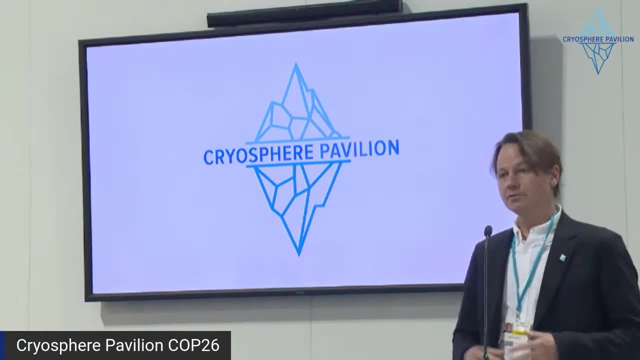 I can start by just giving an overview of the session in general. We will have three talks. I will start with an introduction to permafrost thaw, also linking it quite a lot to the most recent report from the IPCC, the Working Group, One report from the Sixth Assessment Report. 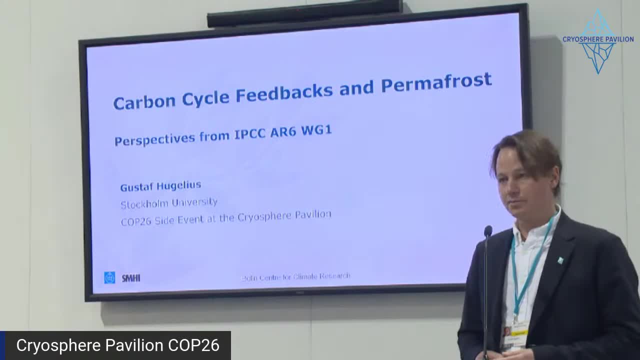 And then after that we have talks from Jens Strauss and Sarah Chadburn, Then we go into a panel and after that we'll take questions. Okay, but I will start with my first talk, which is on carbon cycle formation. We will take questions from innovation. 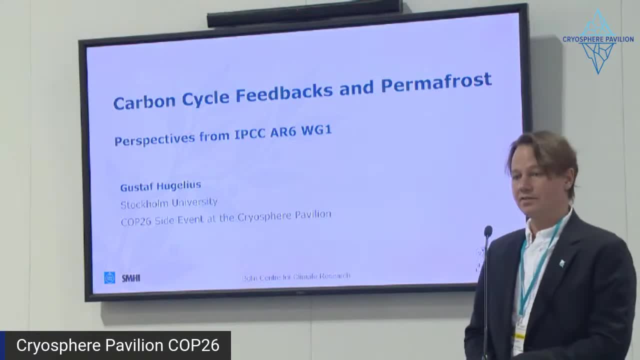 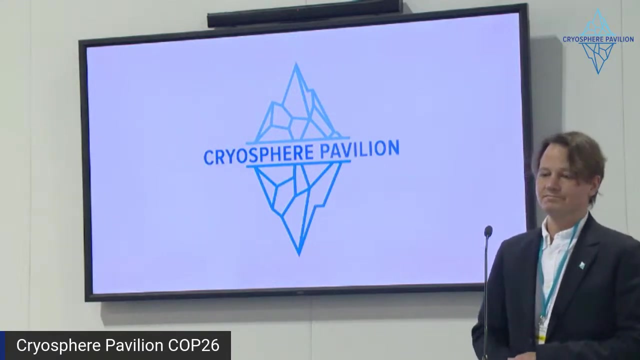 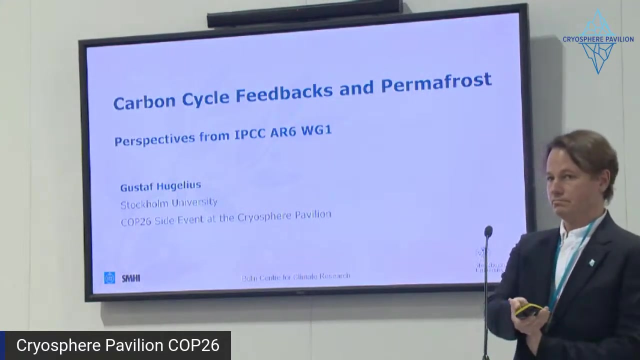 general overview with perspectives from the Working Group One of the IPCC. There's some technical issues with changing the slides. I think they turned off the slideshow. Yeah, please bear with us while we're working through the technical difficulties. Oh, now we're here again. 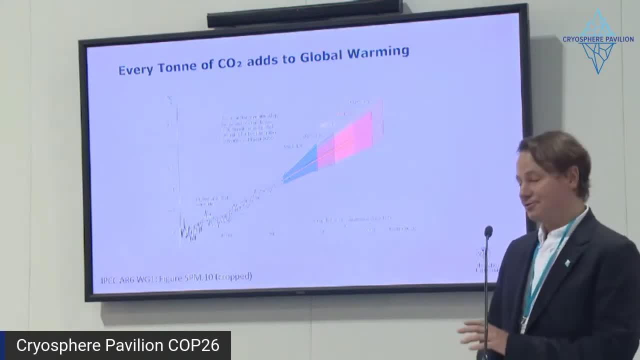 Okay, great. So now we're rolling. So the first slide of my talk is from From the IPCC report. For all of the slides you'll find the sources to the bottom left. so if you want to dig in more in the report to sort of where the material comes from, 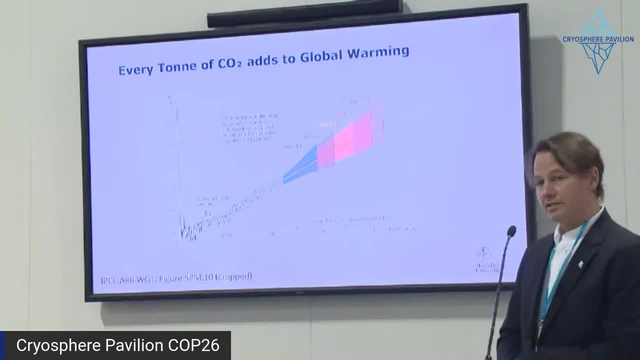 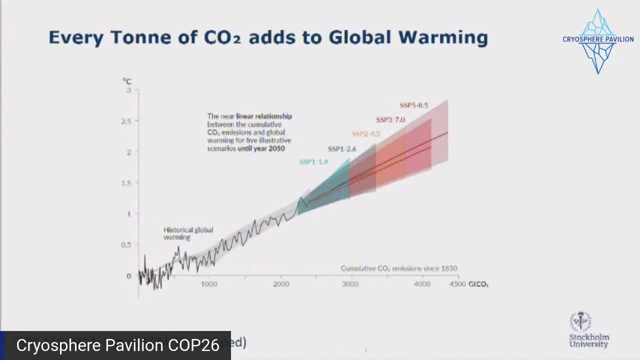 This is a graph that shows you, on the x-axis, cumulative human emissions since 1850, plotted against temperature increases And it's historical global warming, and then you go on to different emission trajectories And one of the take-home messages is that we see basically a linear relationship where 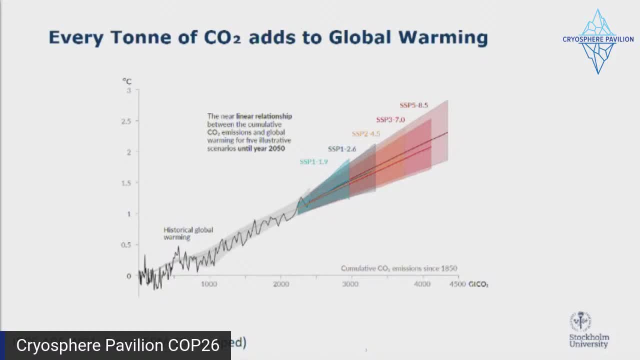 every ton of added CO2 to the atmosphere adds to global warming, So there are no sort of safe thresholds to hide beneath or anything like that. Every added ton adds to the warming. But another important thing here is to think about what the warming trajectory would have. 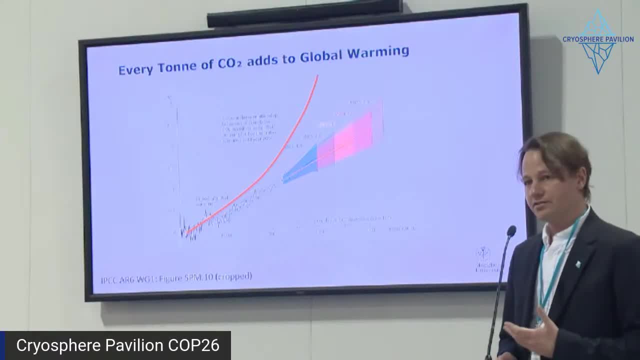 been if we wouldn't have had natural sinks in the Earth's system that actually buffered the emissions for us. So this orange line roughly outlines what the warming trajectory would have been if we wouldn't have had natural sinks in the Earth's system that actually buffered the 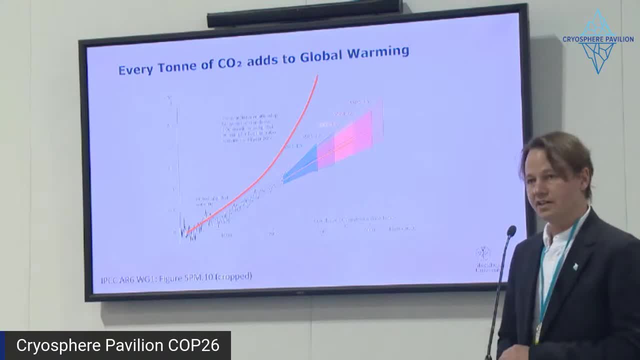 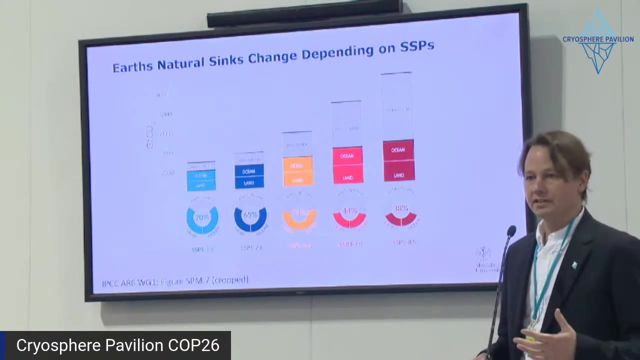 emissions for us And what warming would actually be unless we had natural sinks in the Earth's system that actually dampen the emissions and take up some of the carbon dioxide that we add to the atmosphere. So basically, the terrestrial biosphere and the oceans take up roughly half of the CO2. 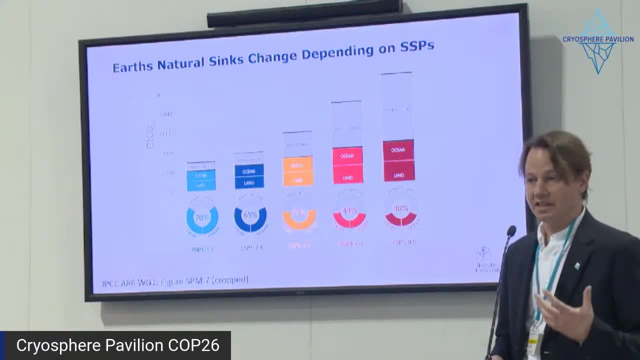 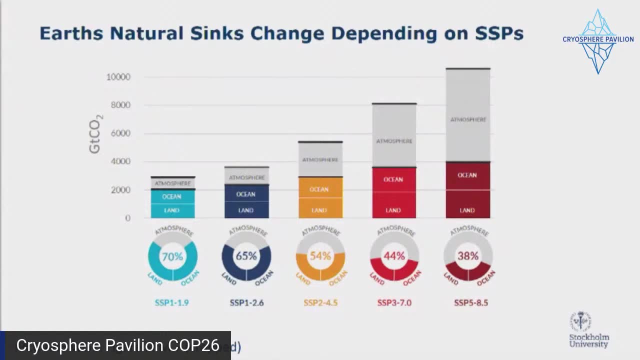 that humans emit and we actually only see half of the CO2 staying in the atmosphere and actually warming the climate. One thing that is emerging is that these natural sinks are actually weakening And they are changing depending on which scenario we are going to follow. 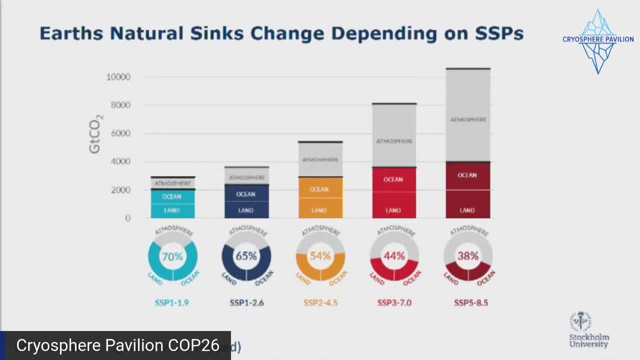 So this is another figure from the IPCC report that shows you from starting in the light blue color in the left and going toward the redder colors, show you the different scenarios or pathways of emissions, ranging from the really low 1.5 consistent scenario to a very 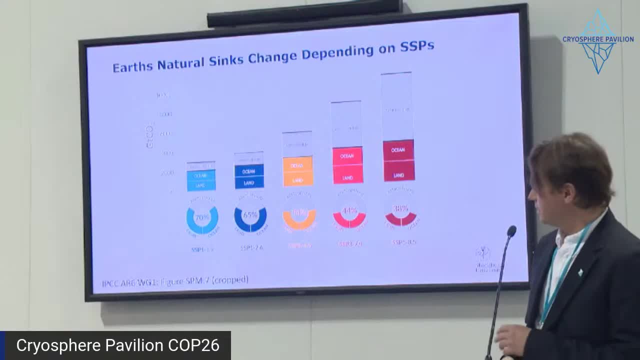 high scenario at the end And what you see- you see the upper bar charts- are the cumulative emissions And then you see how much of those emissions will actually be reabsorbed into the Earth's system, either ocean or land. And, in the optimistic scenario where we actually stick to a low-emission scenario, the natural 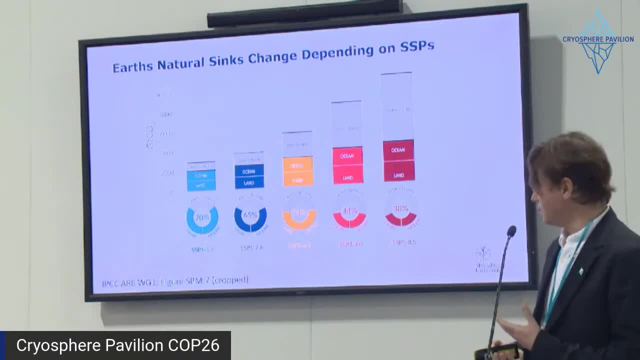 sinks are going to take up 70% of the emissions, But these saturate And if you go to the far right you see that the Earth's sink capacity to actually absorb CO2 is weakening. So this is a very interesting scenario. 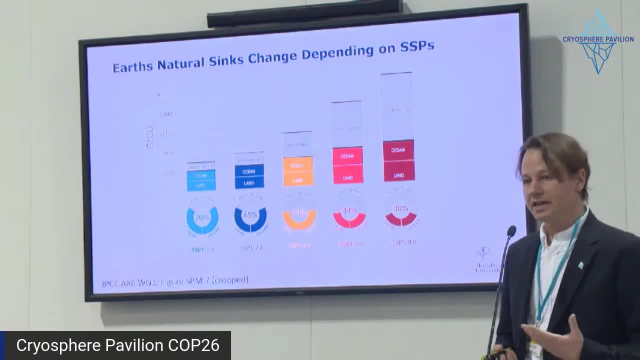 And then you see how much of those emissions will actually be reabsorbed into the Earth's system, either ocean or land. And I think the reality is actually even more dire, because some of the natural feedbacks that would add more CO2 to the atmosphere are not fully included in the models that 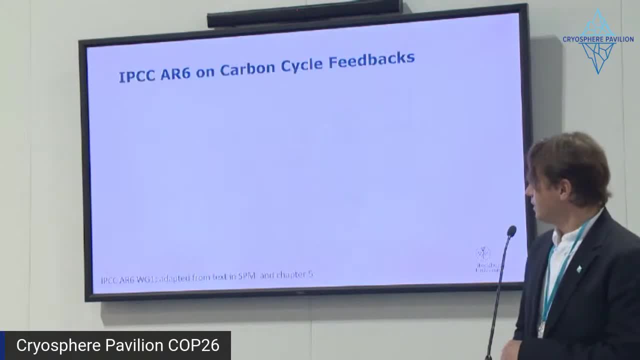 are behind these graphs. So here I list some of the take-home message for the summary for policymakers on carbon cycle feedbacks as outlined in AR6.. So they note that the carbon climate feedbacks increase with warming and become more uncertain. So any feedbacks in the Earth's system that would release more CO2 as climate gets warmer. 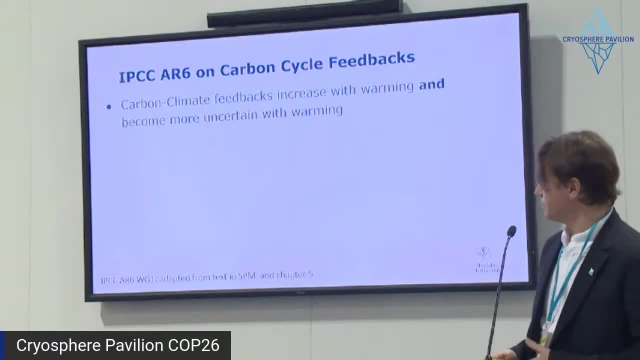 and be a positive runaway effect. not runaway effect, but a positive increasing effect. they are increasing with warming and becoming more uncertain. But they also note that the different scenarios, the different human scenarios, the SSP, still really dominate the uncertainty in future atmospheric CO2 concentrations. 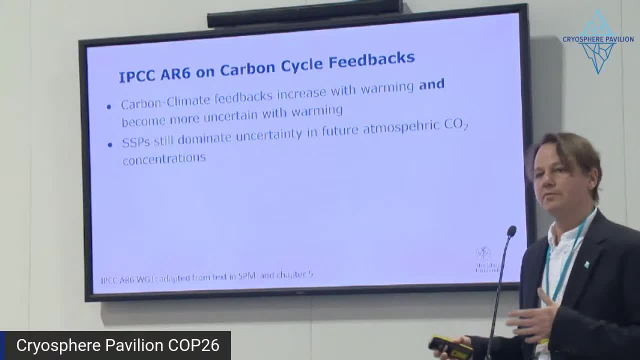 So most of the uncertainty in our projections come from the underlying CO2 emissions. So they also note that the different human scenarios, the SSP, still really dominate the uncertainty in future atmospheric CO2 concentrations. So most of the uncertainty in our projections come from the underlying CO2 emissions. 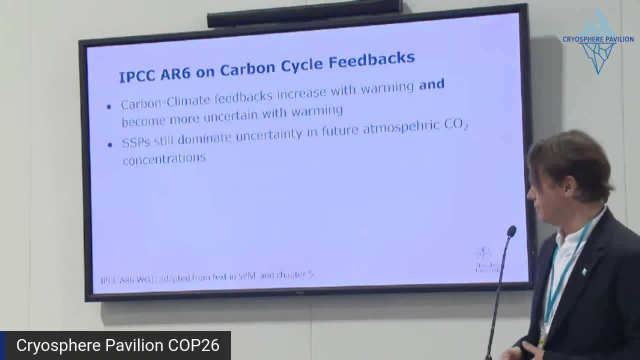 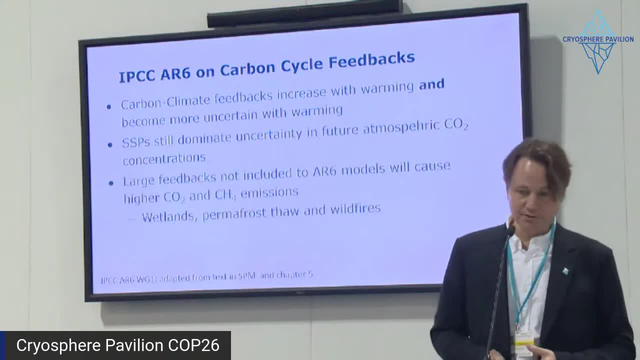 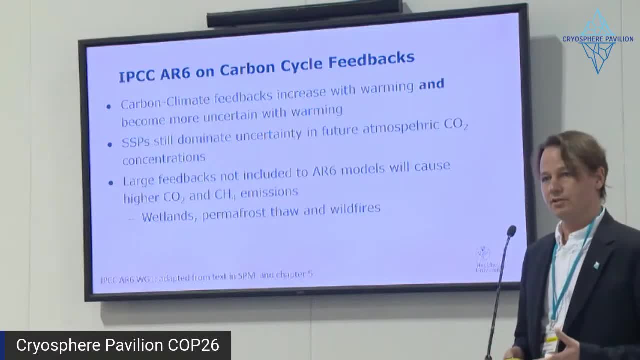 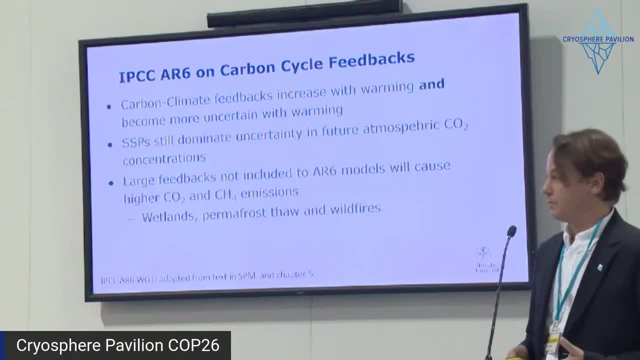 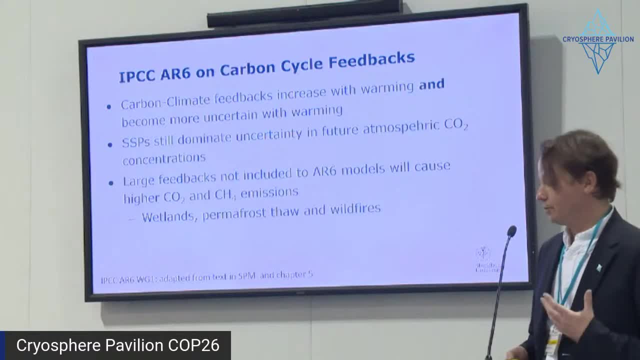 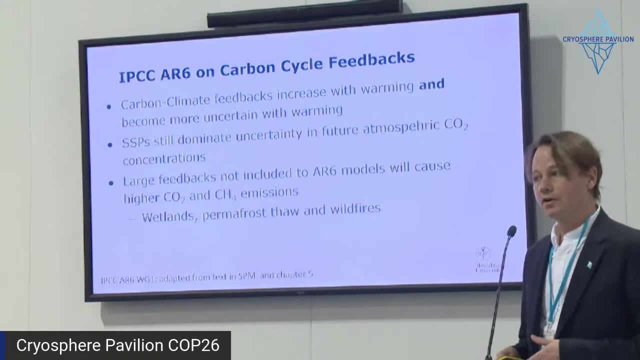 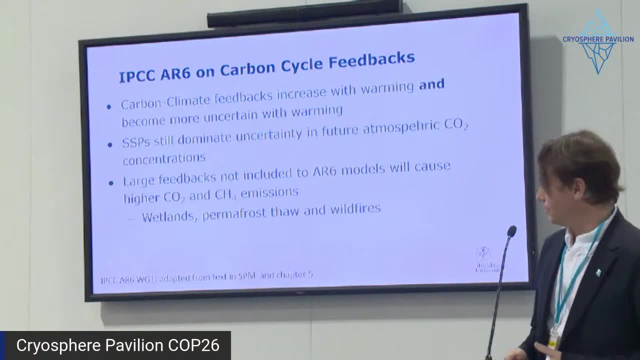 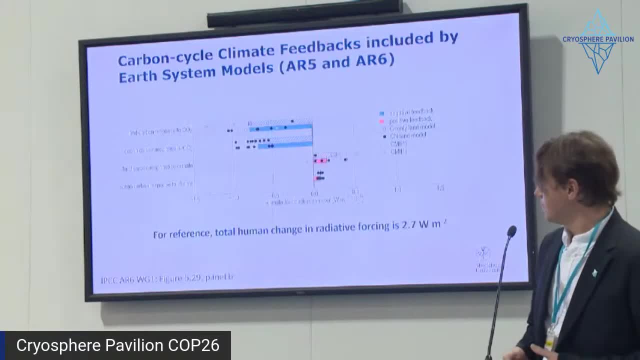 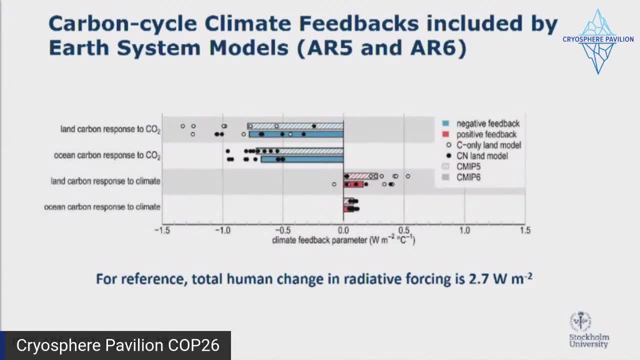 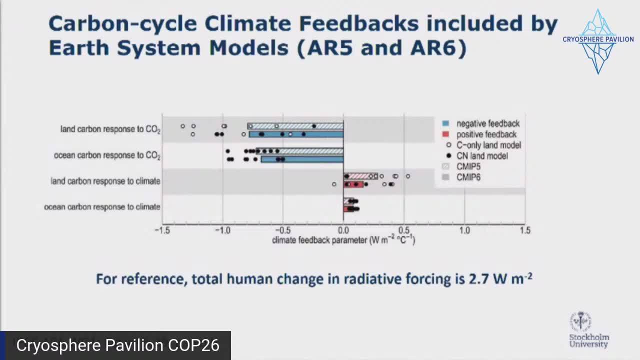 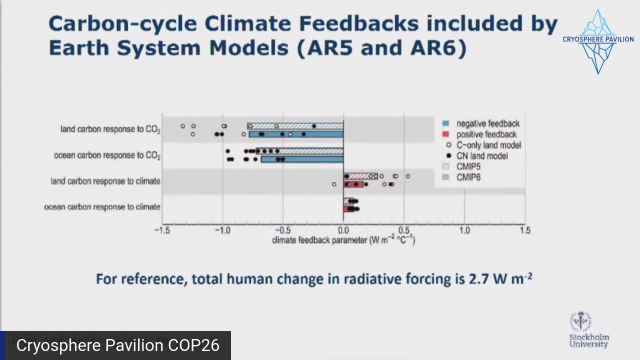 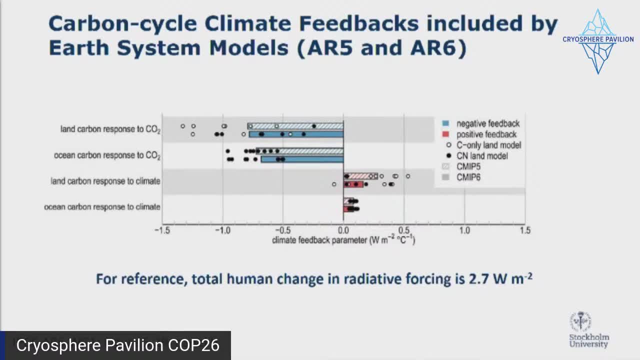 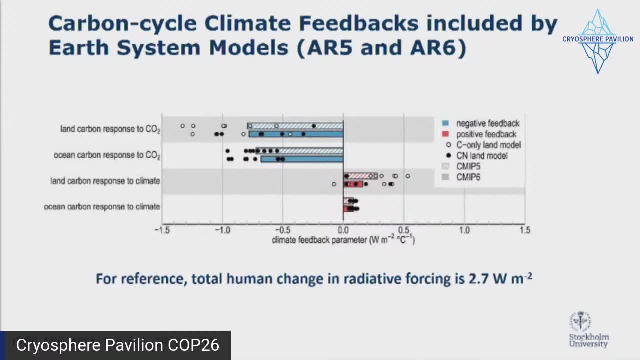 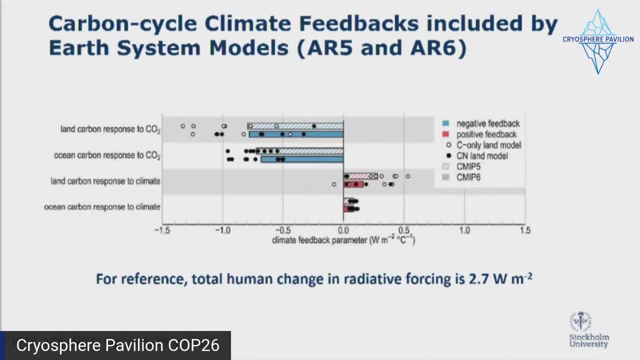 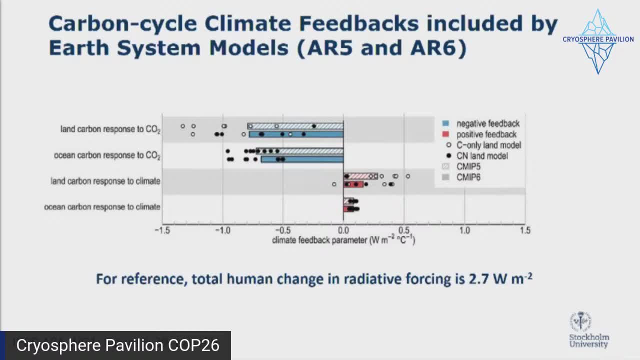 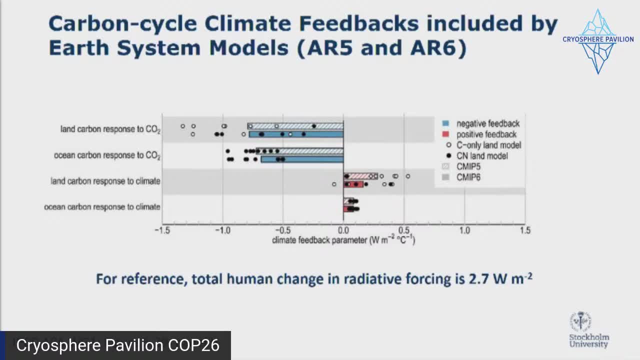 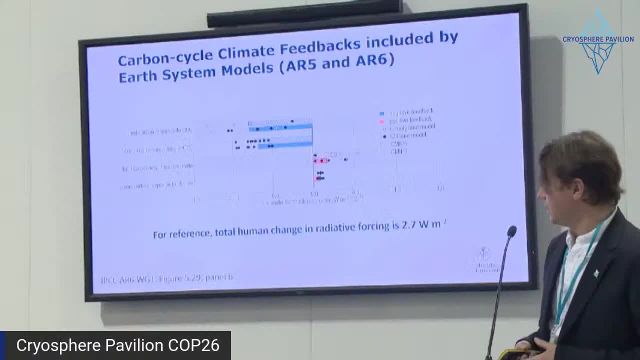 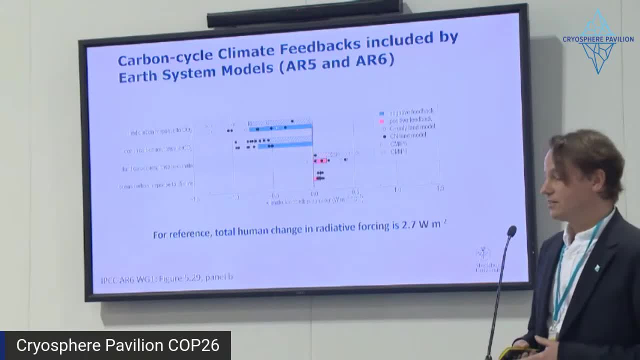 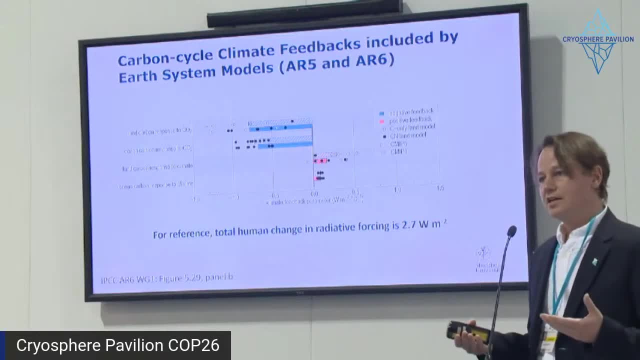 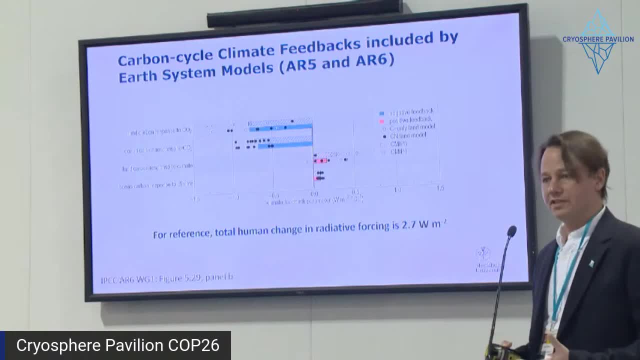 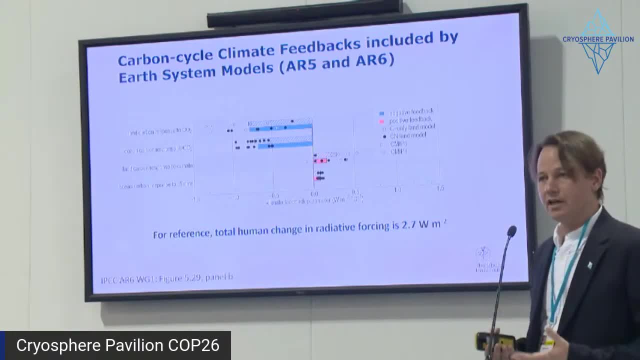 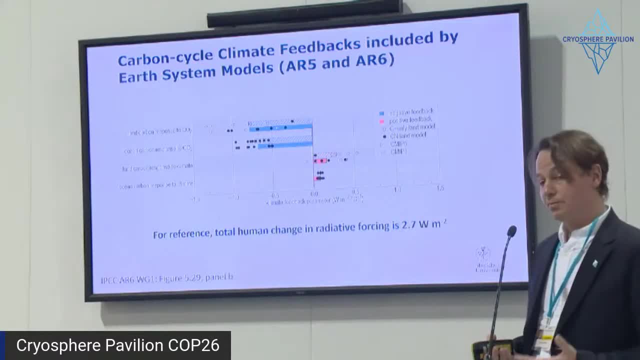 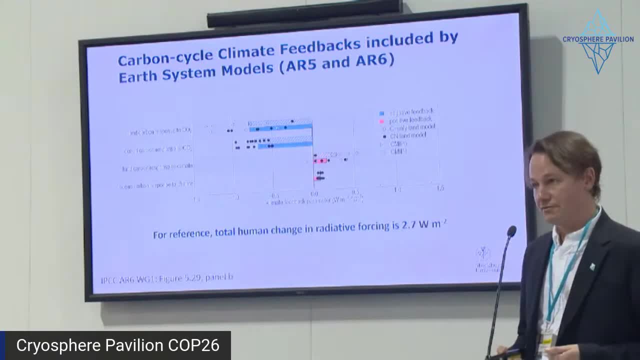 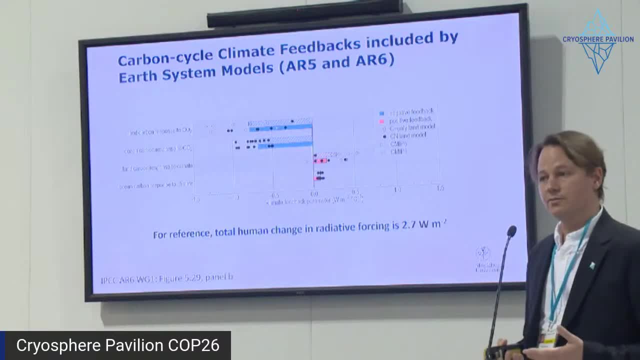 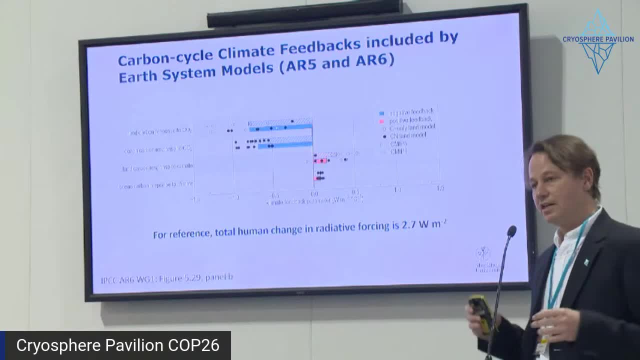 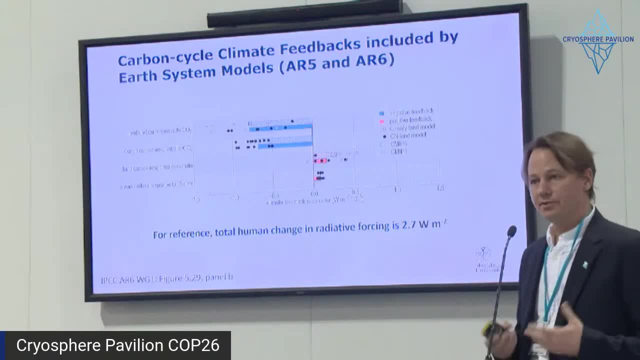 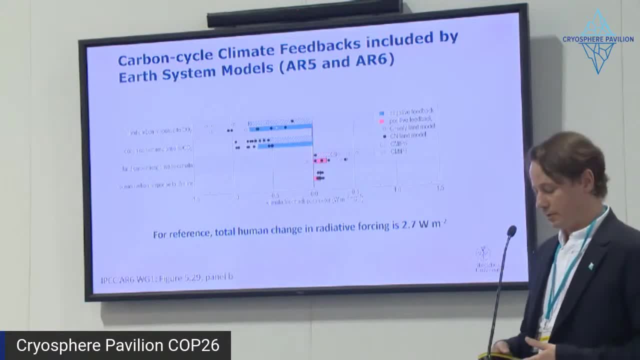 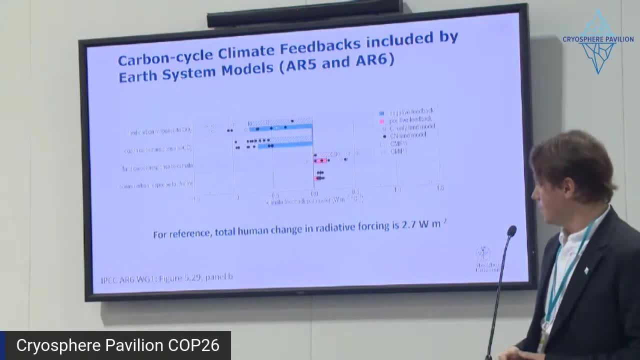 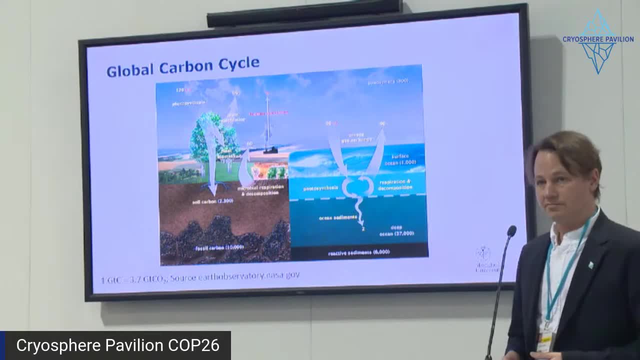 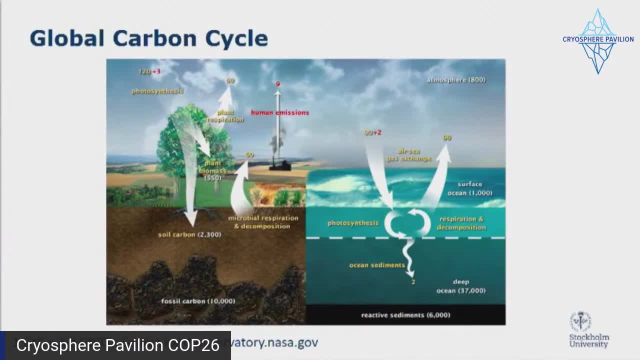 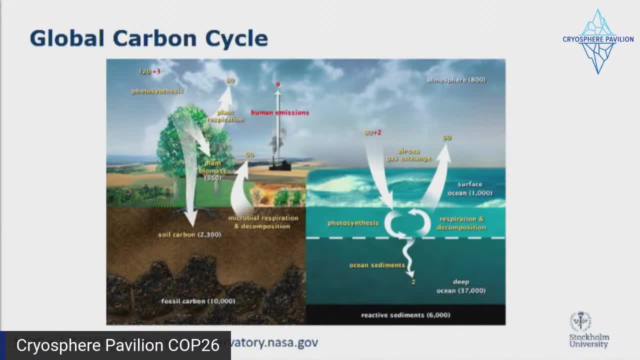 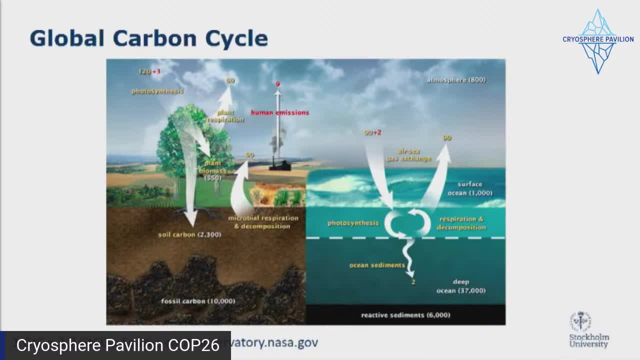 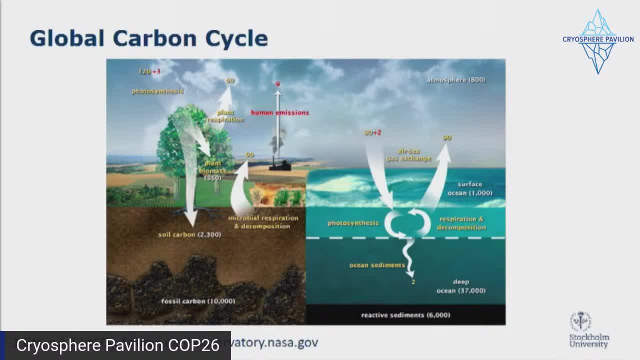 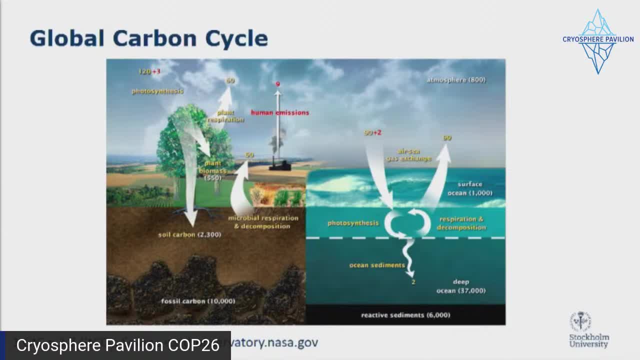 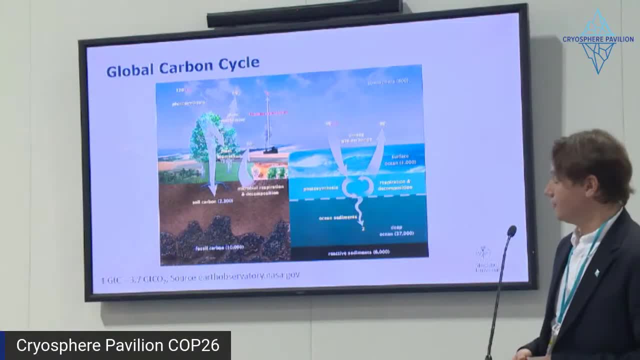 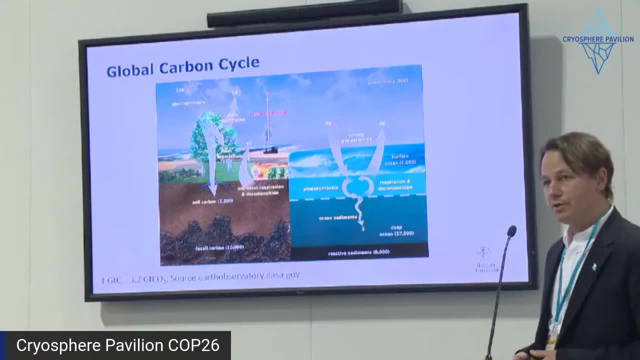 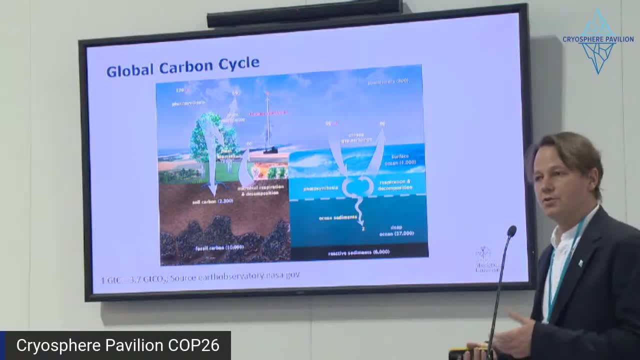 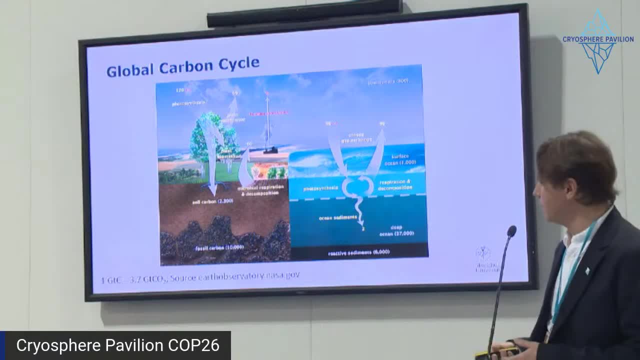 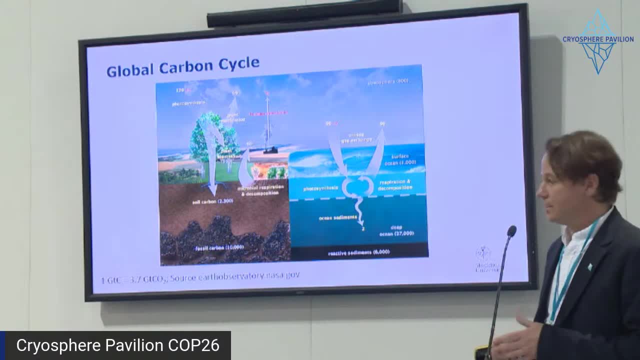 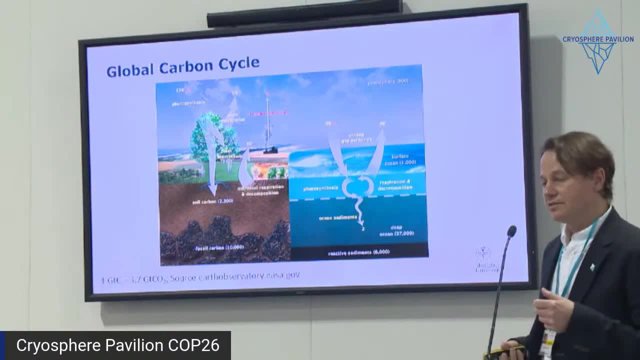 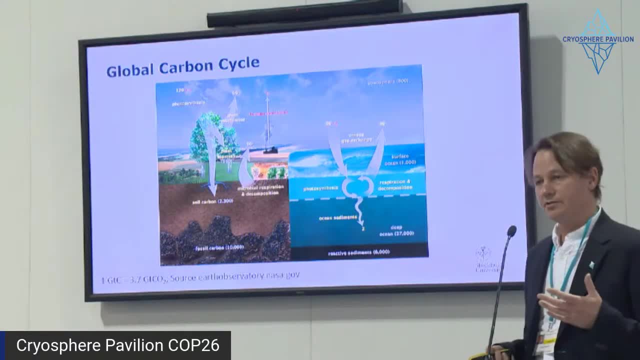 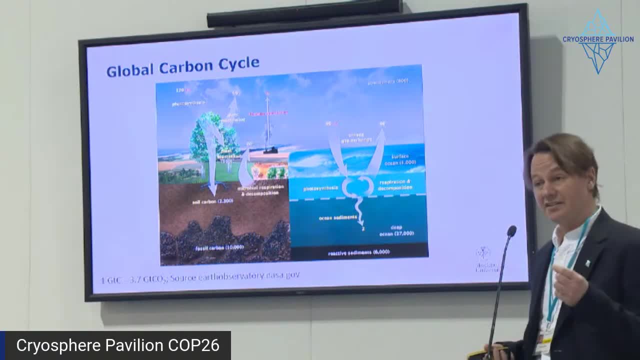 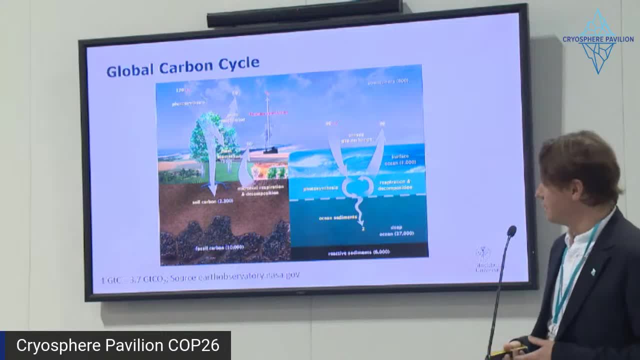 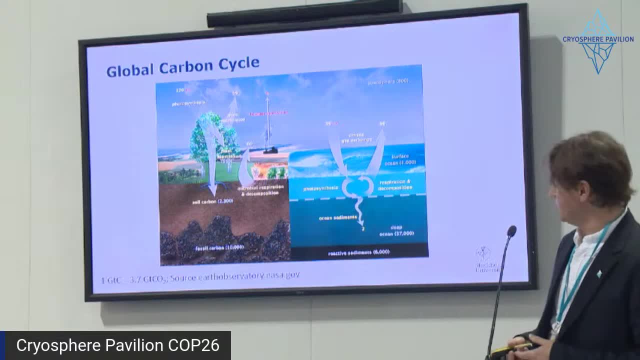 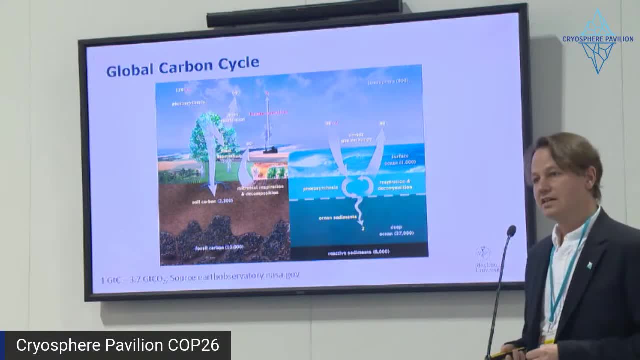 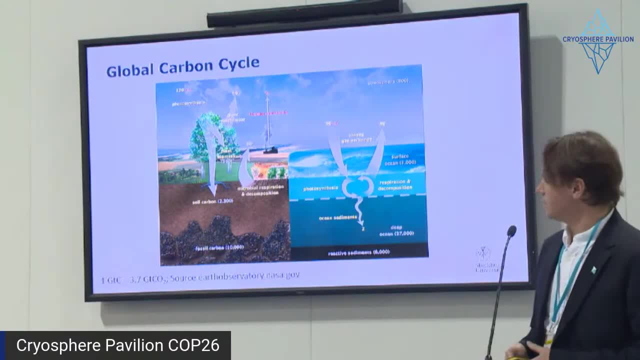 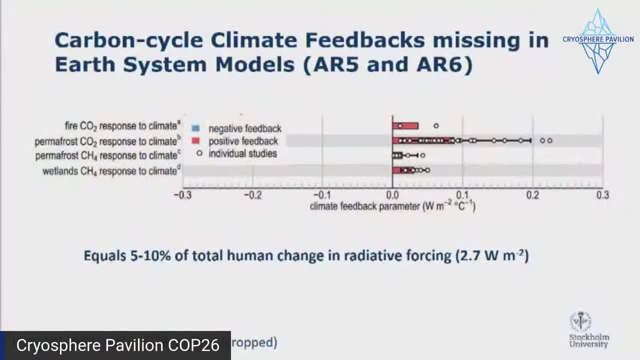 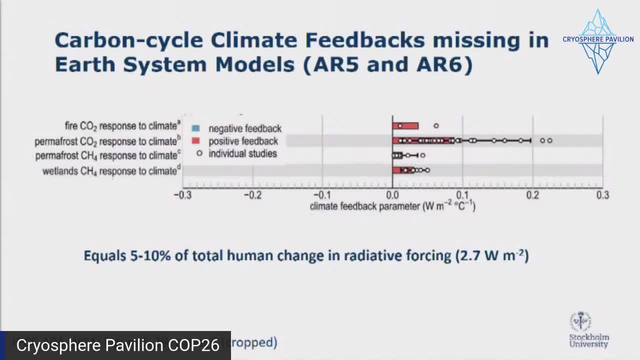 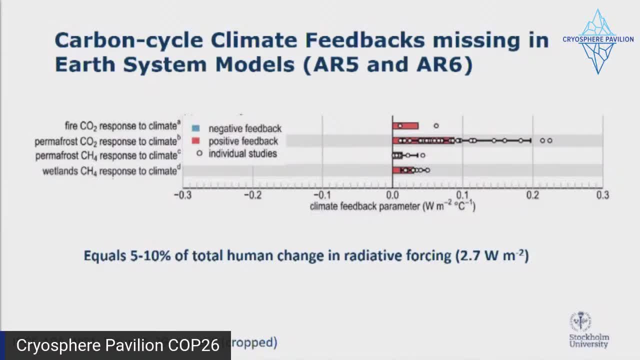 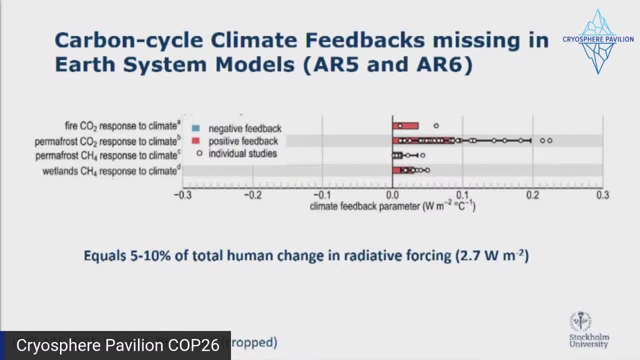 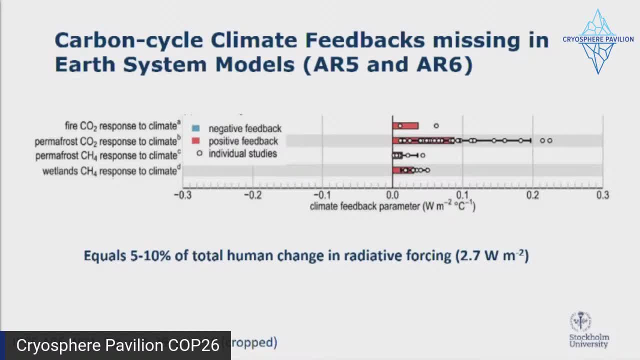 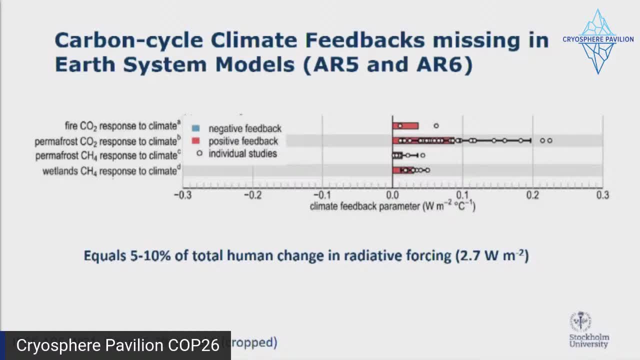 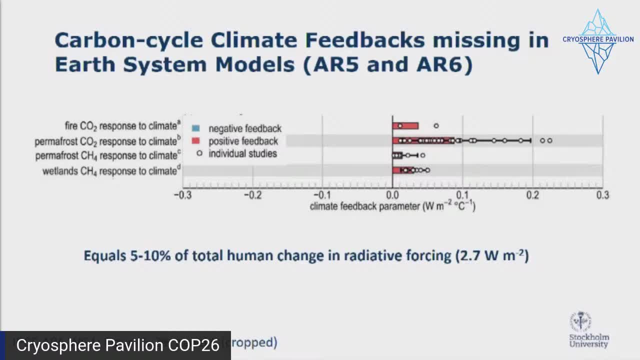 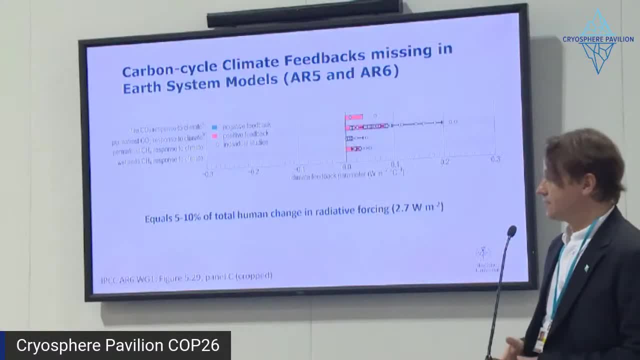 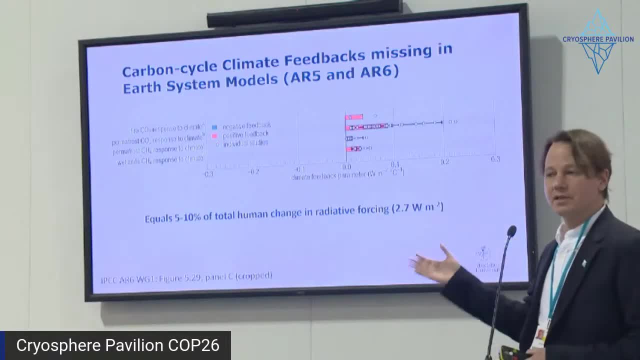 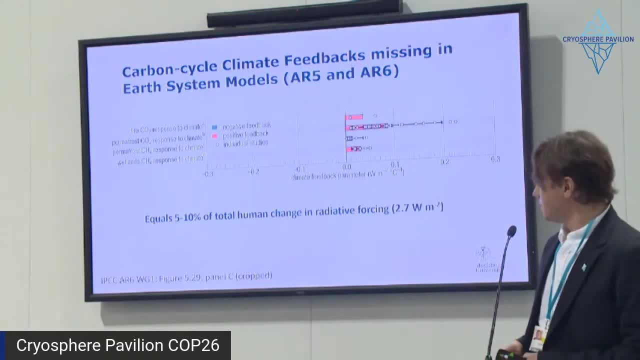 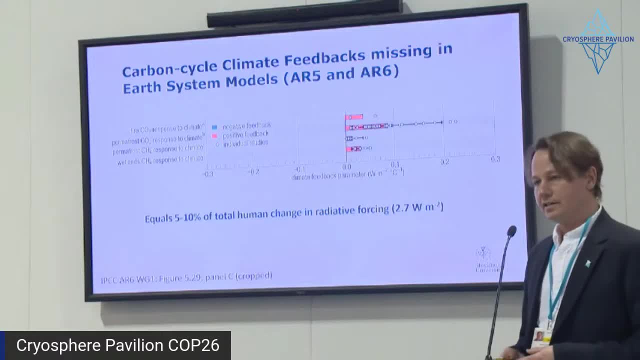 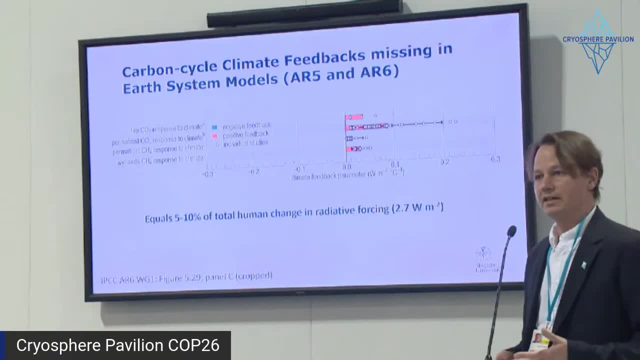 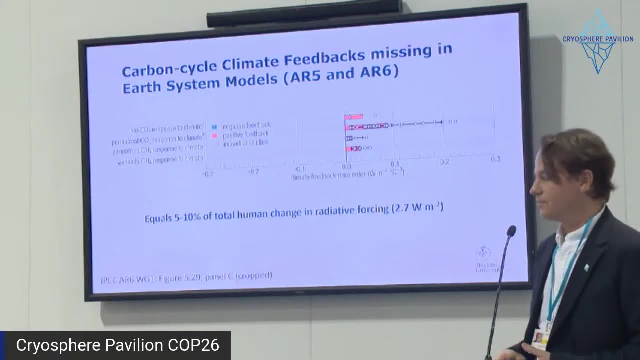 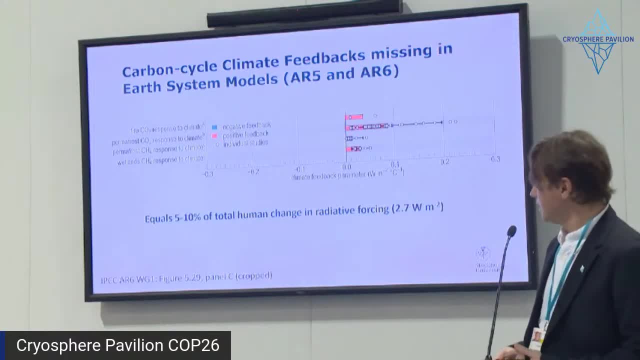 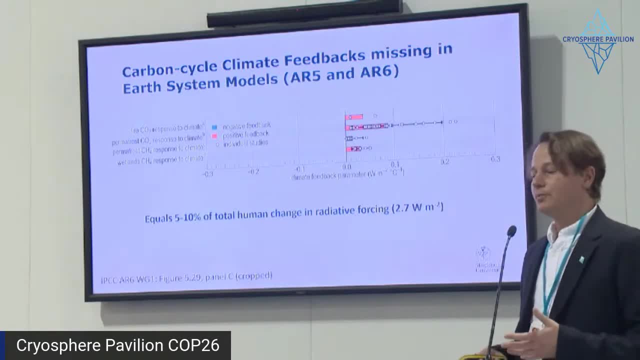 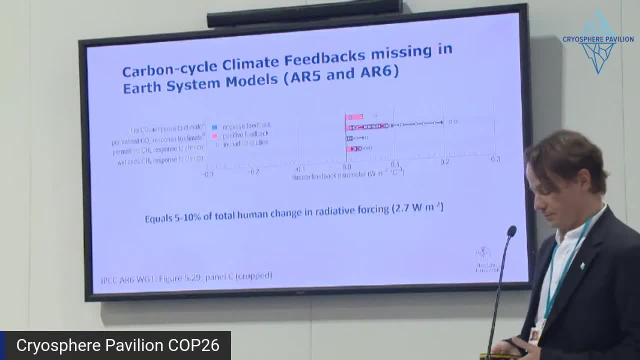 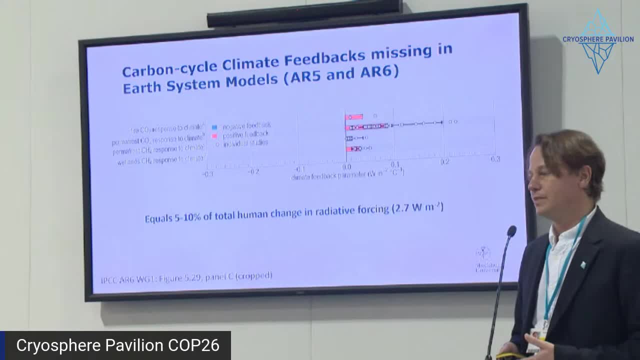 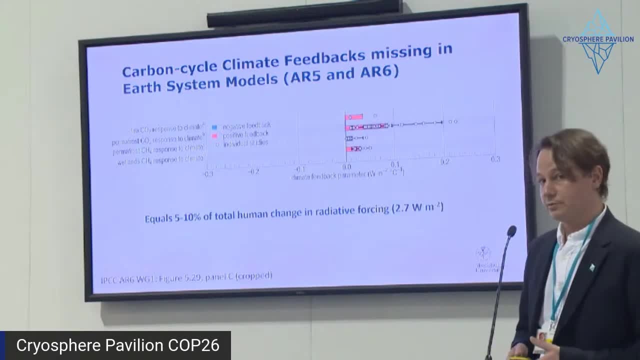 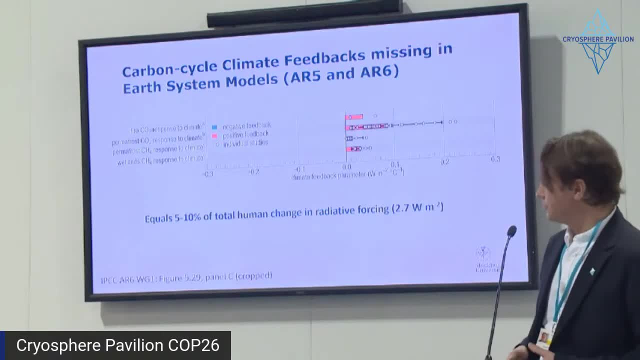 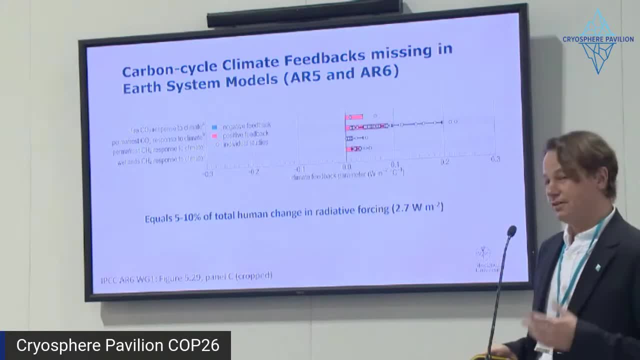 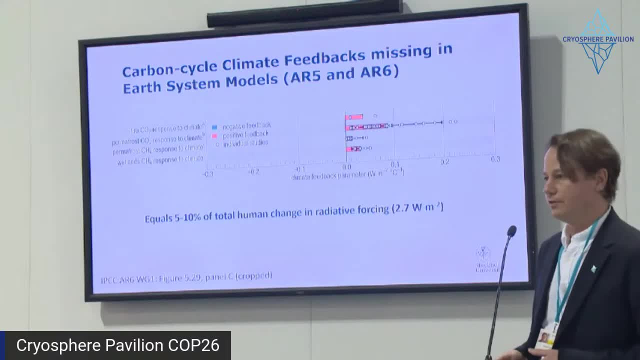 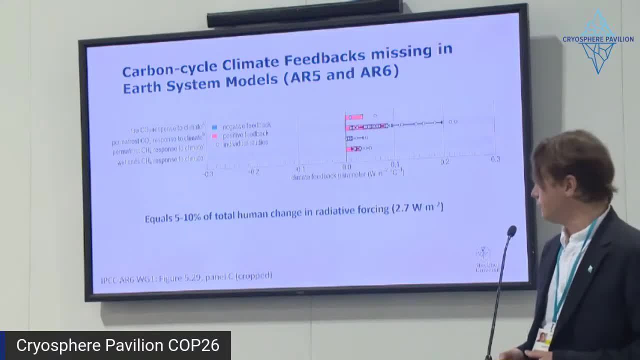 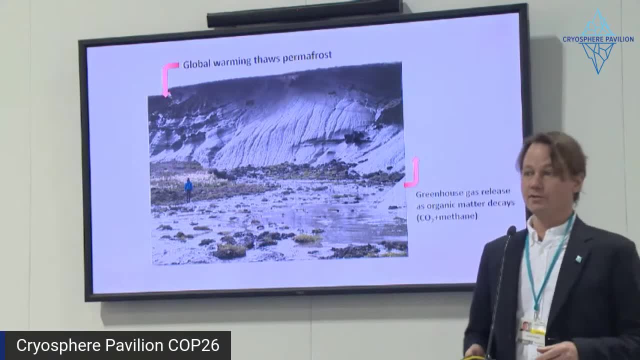 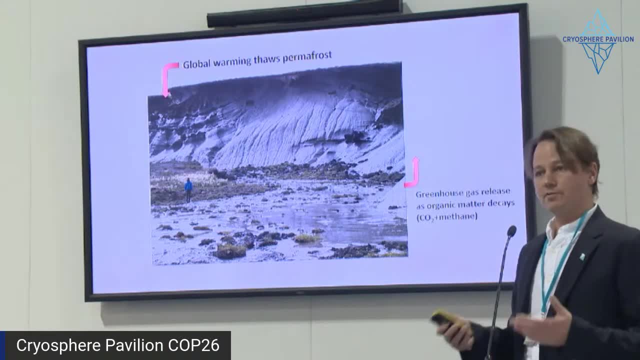 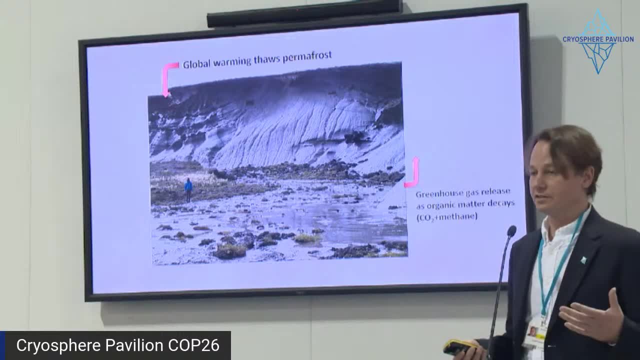 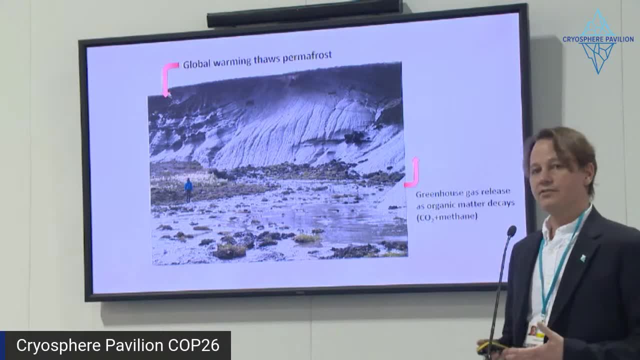 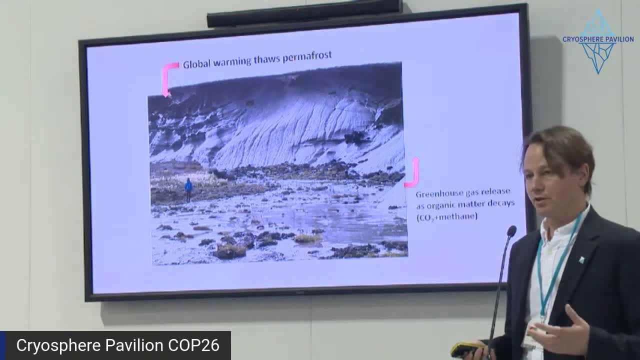 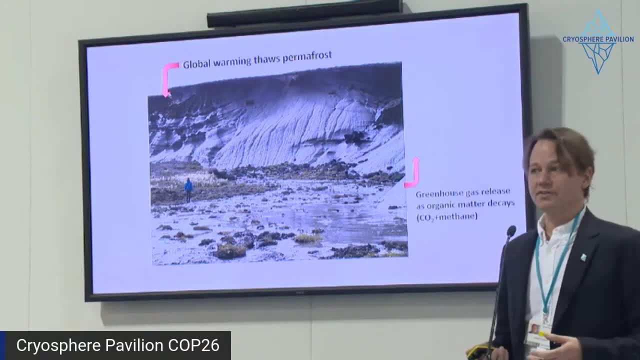 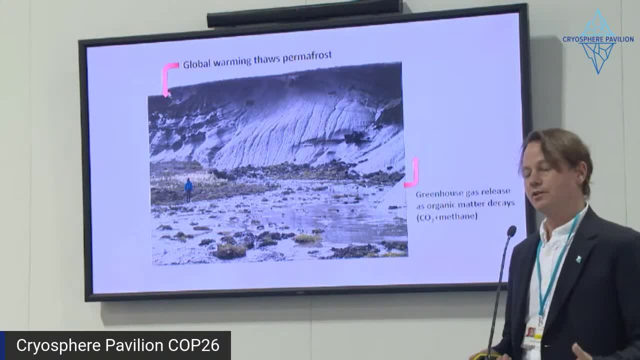 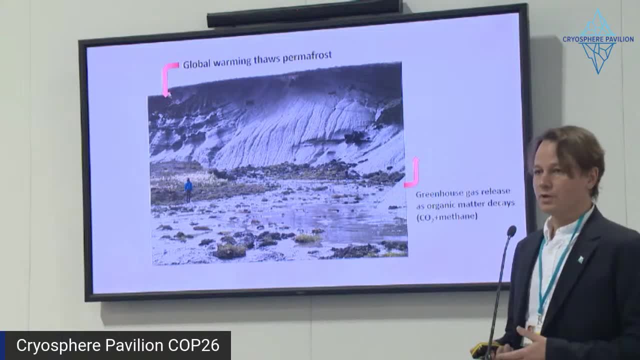 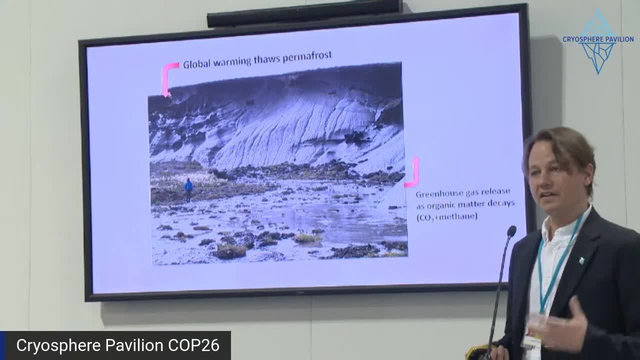 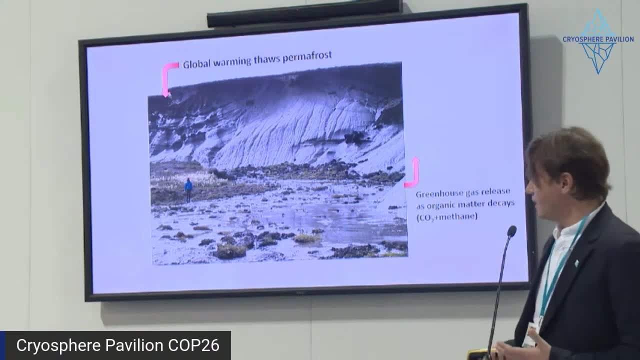 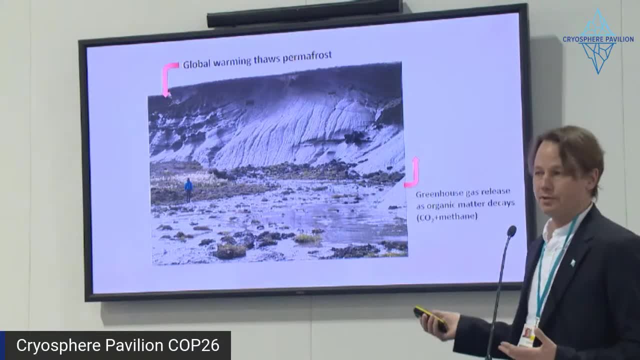 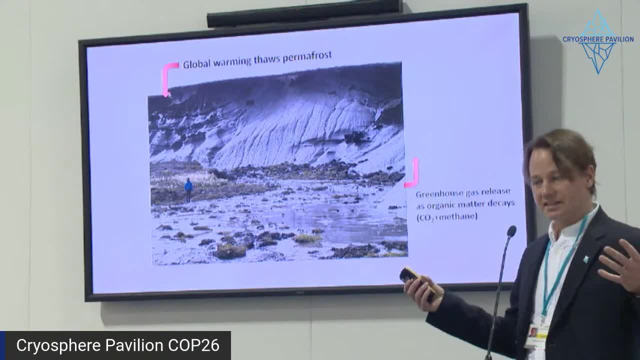 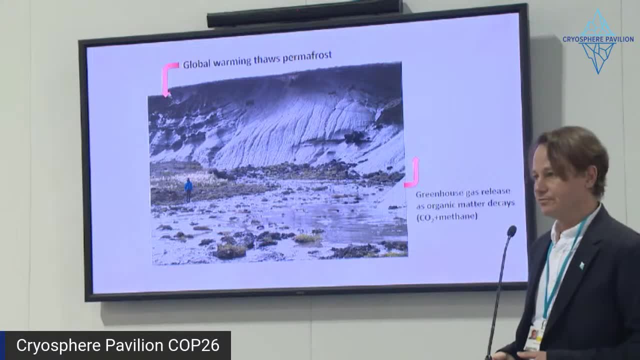 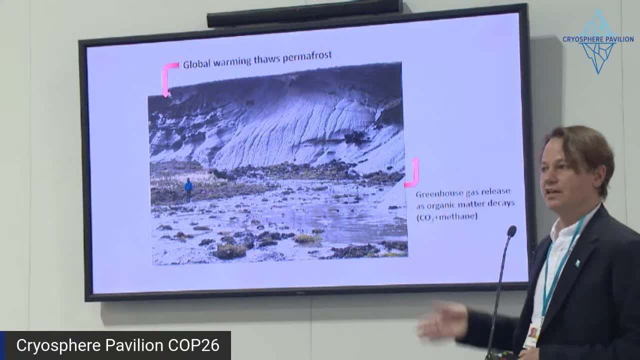 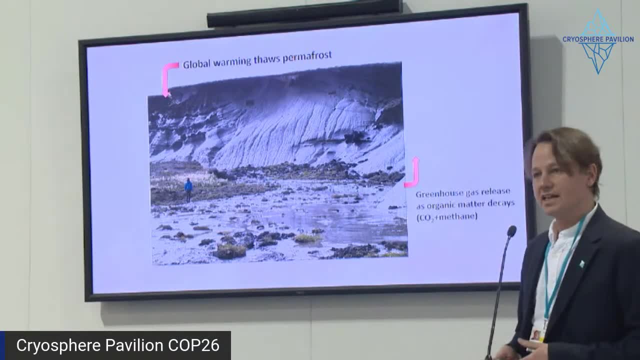 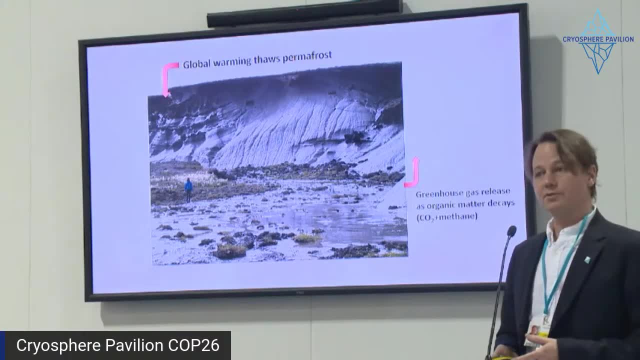 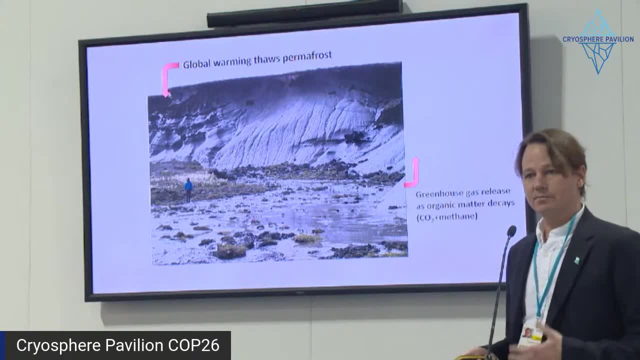 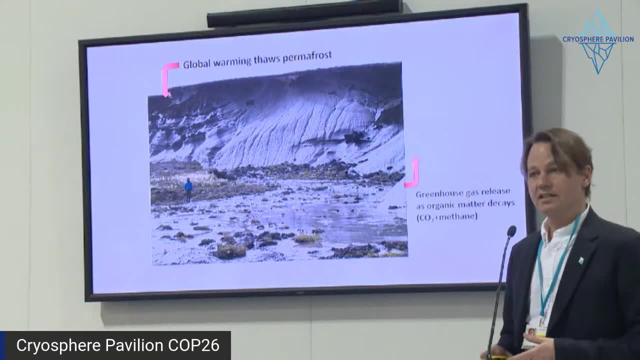 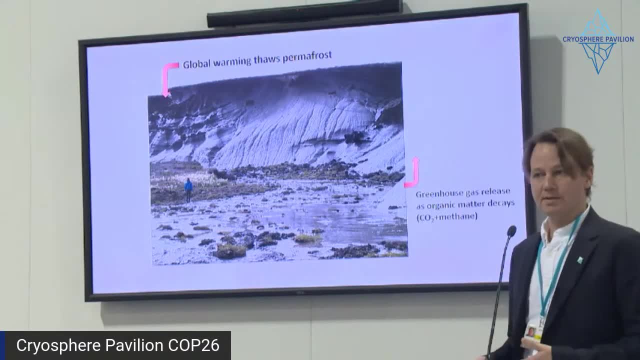 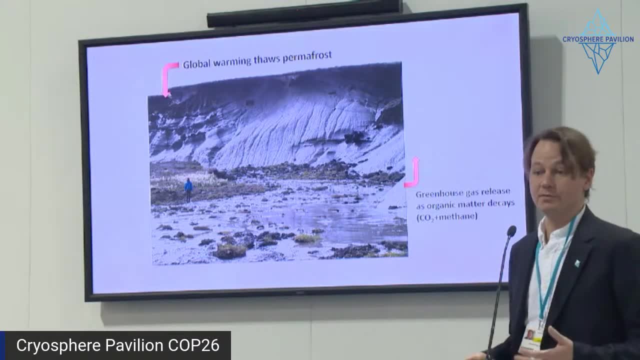 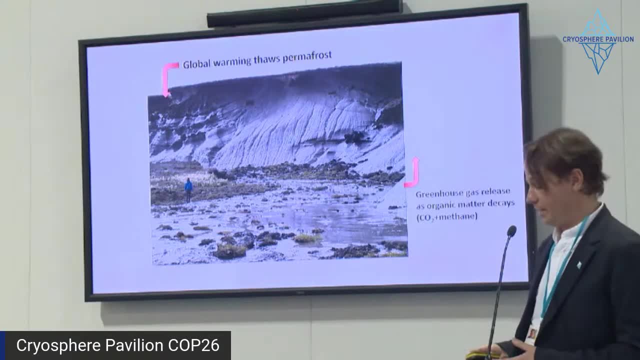 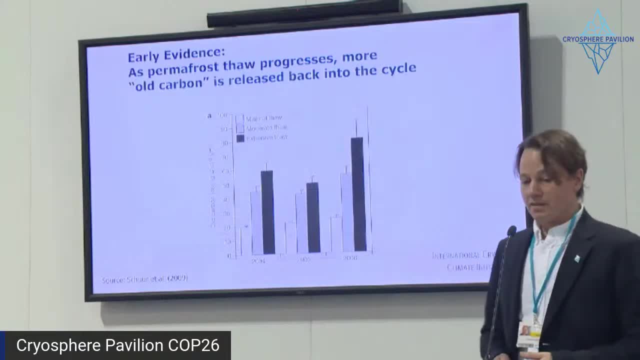 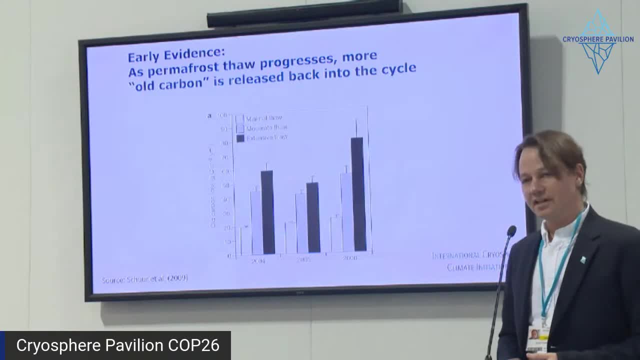 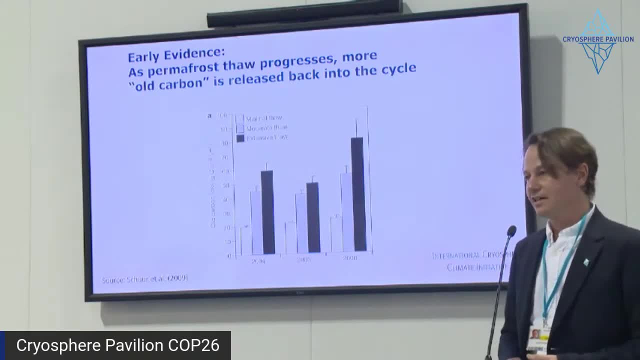 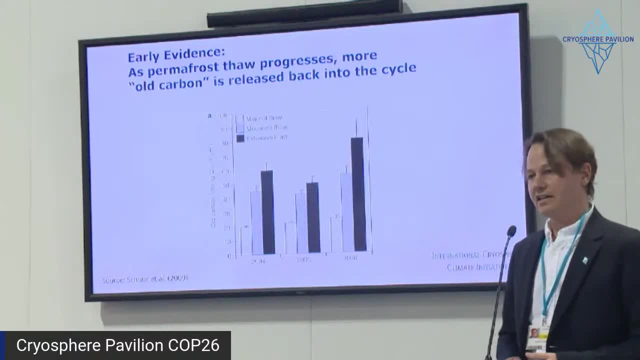 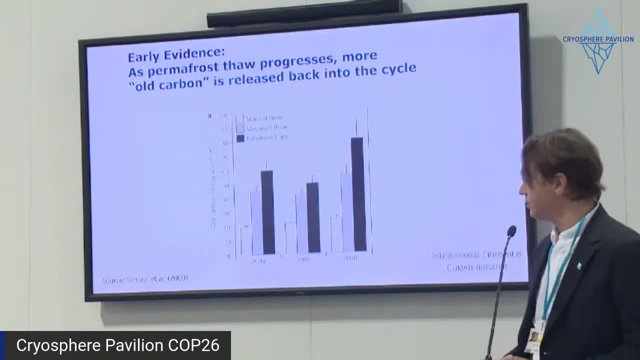 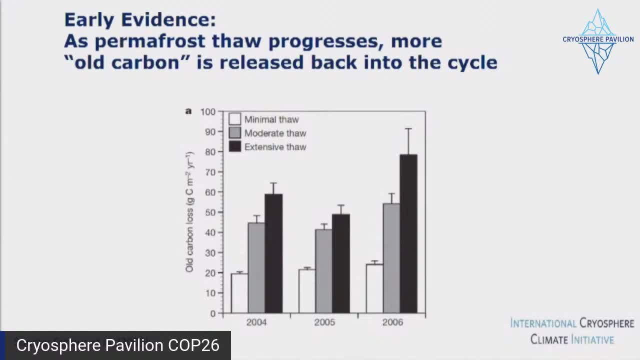 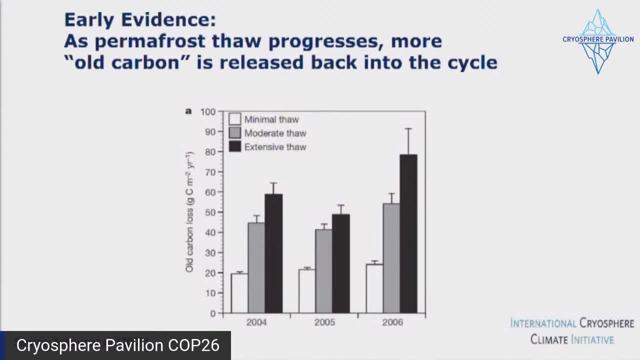 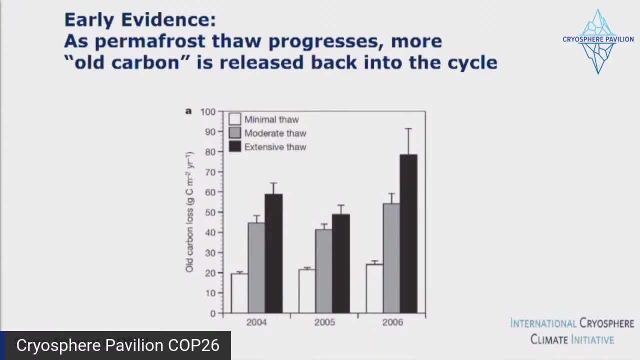 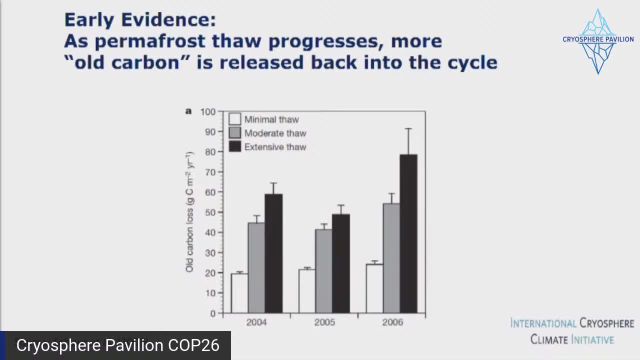 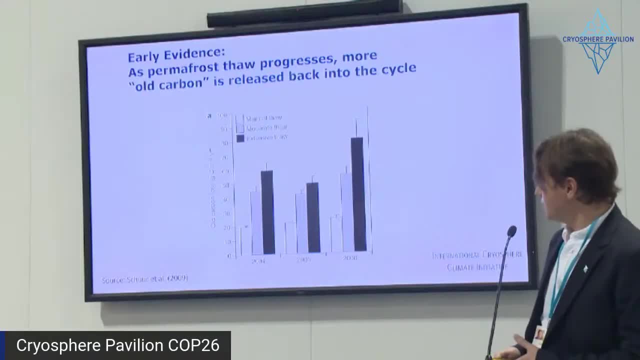 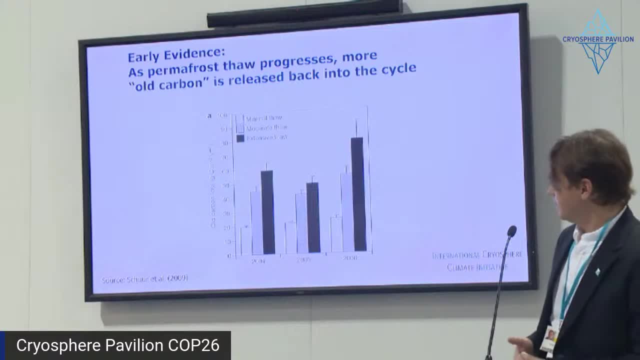 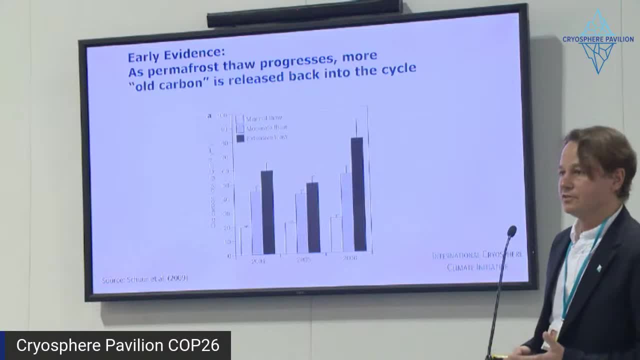 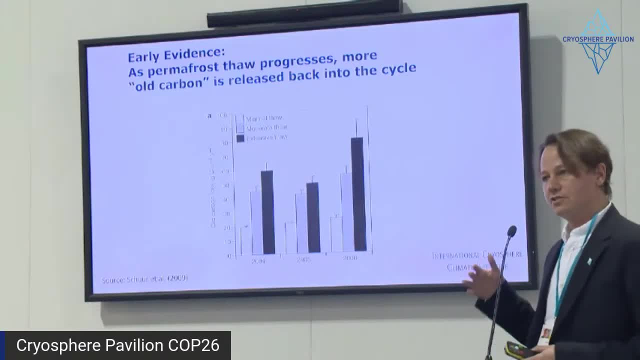 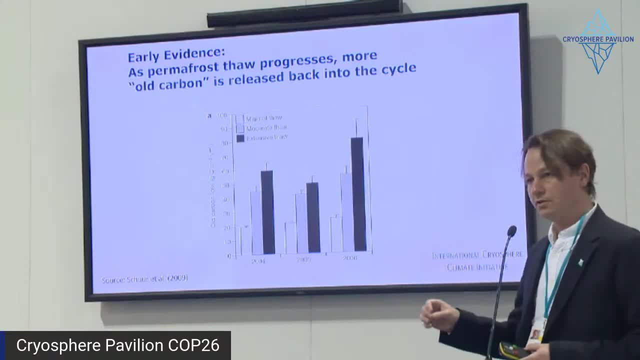 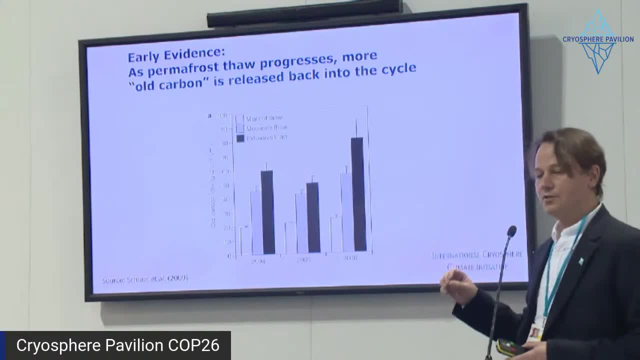 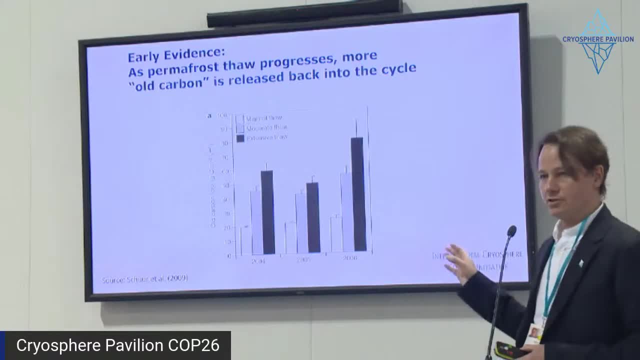 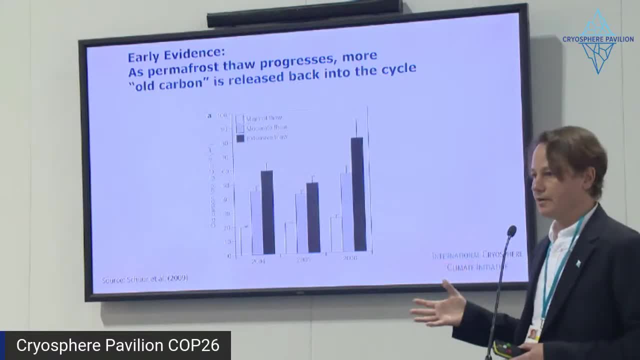 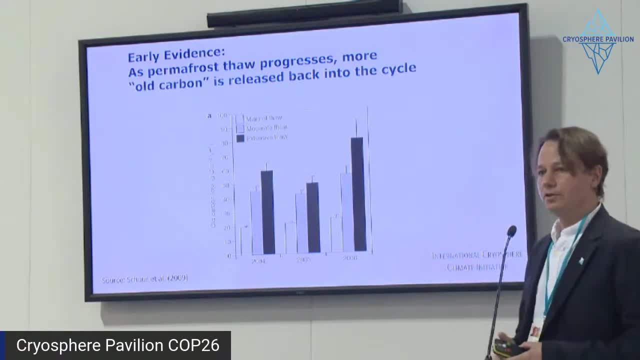 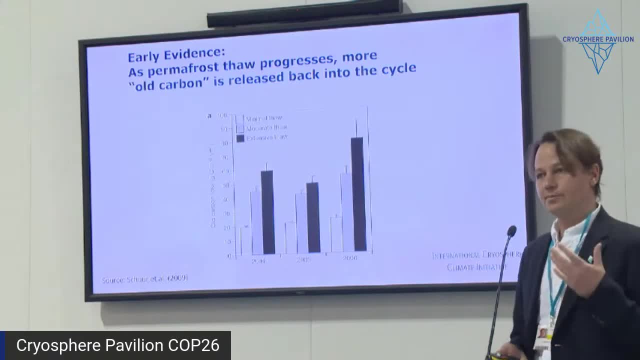 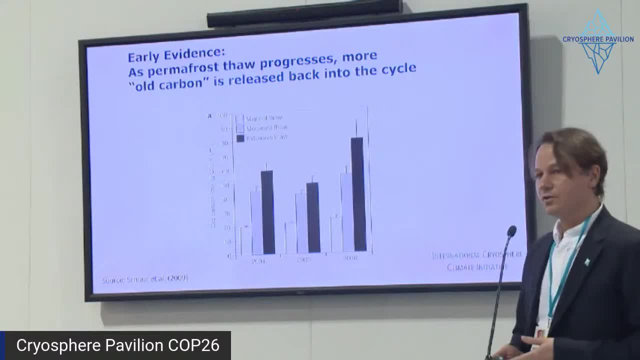 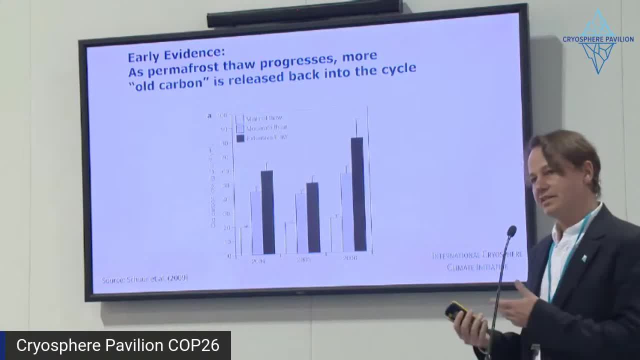 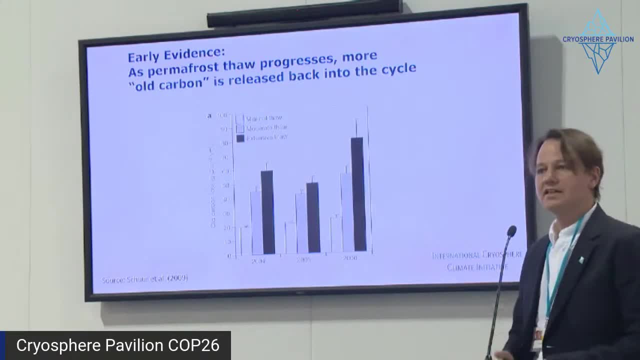 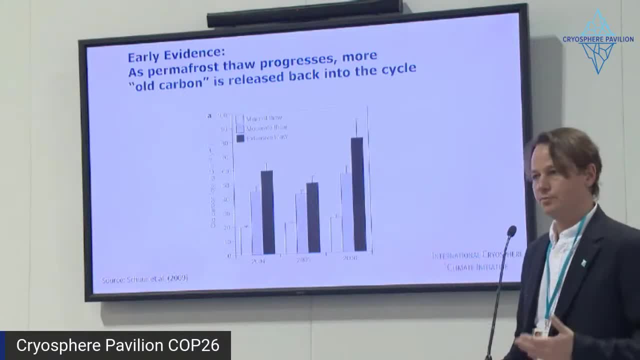 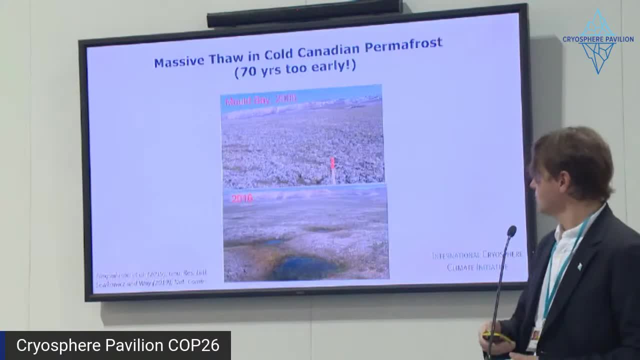 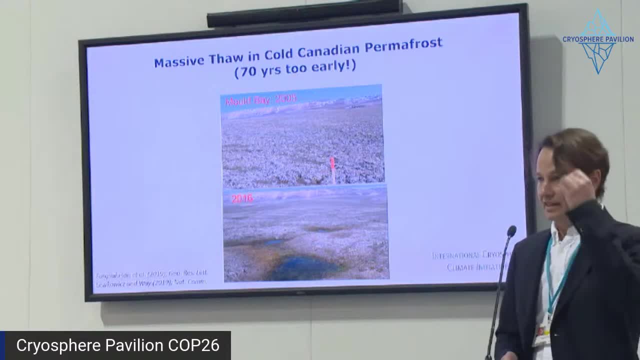 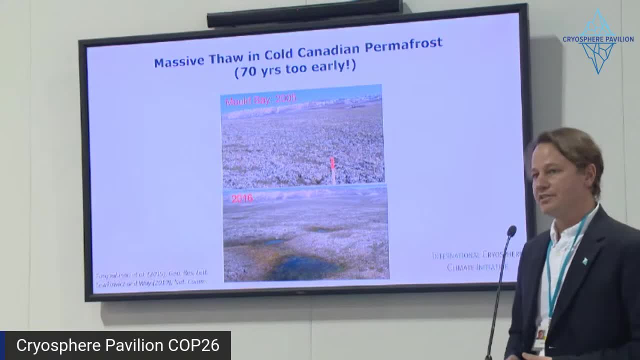 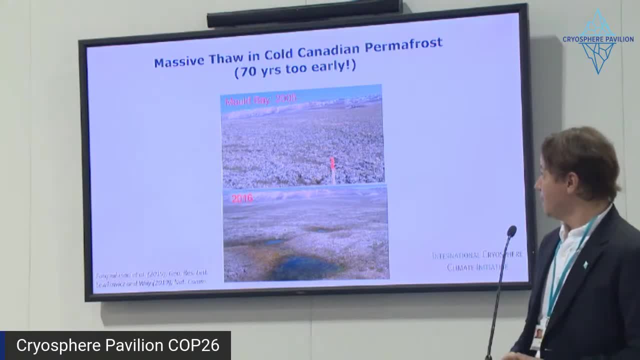 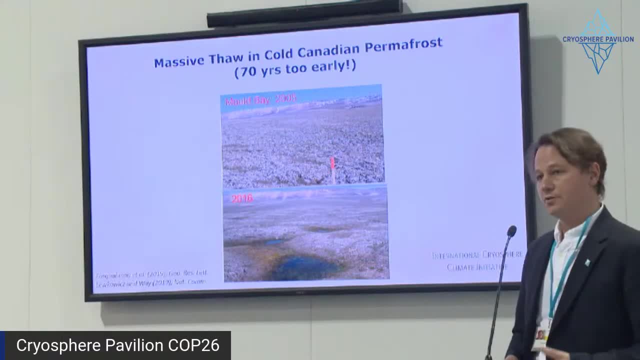 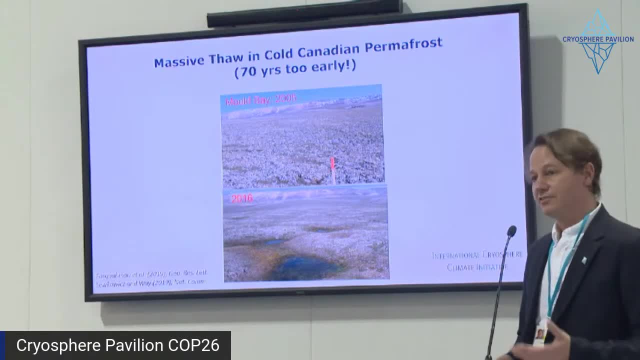 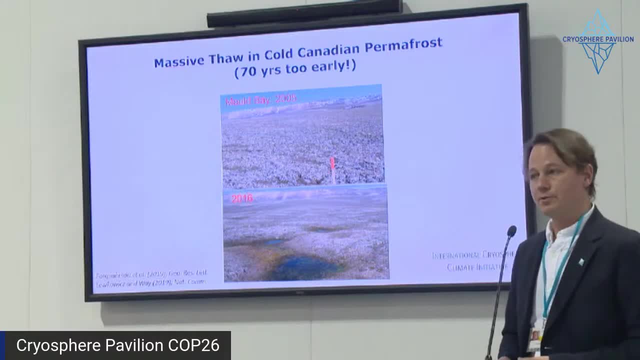 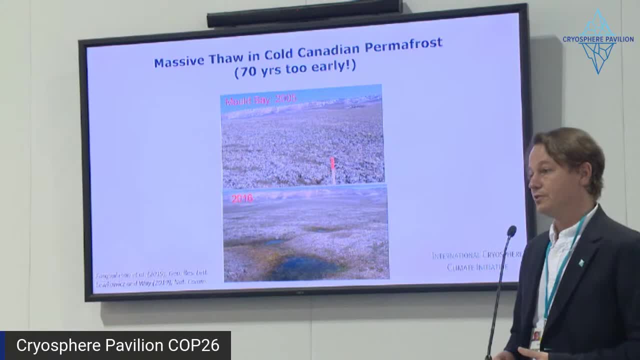 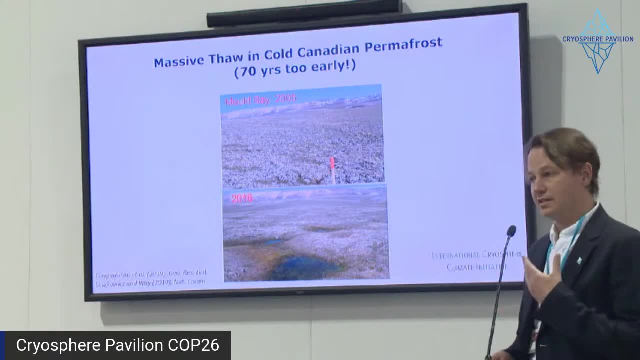 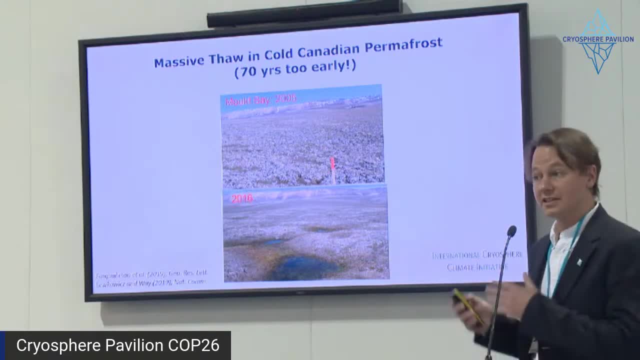 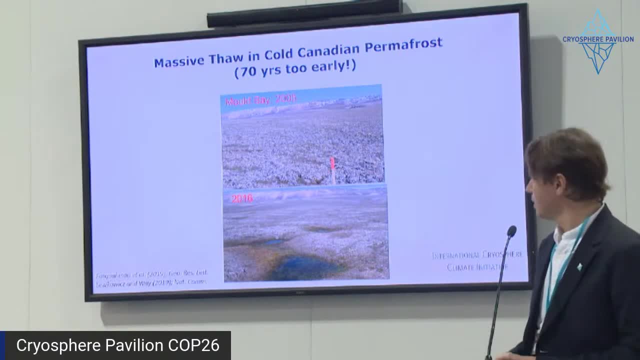 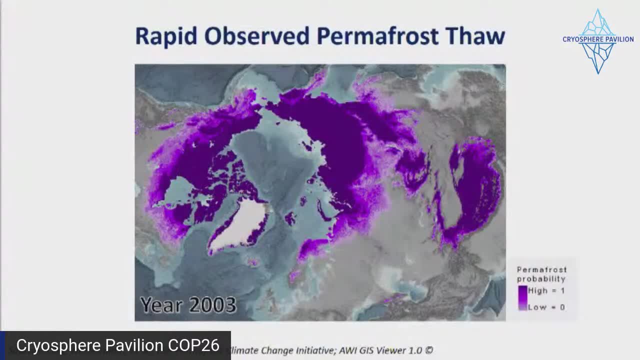 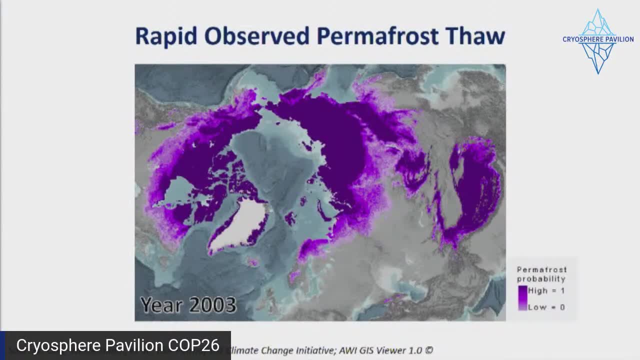 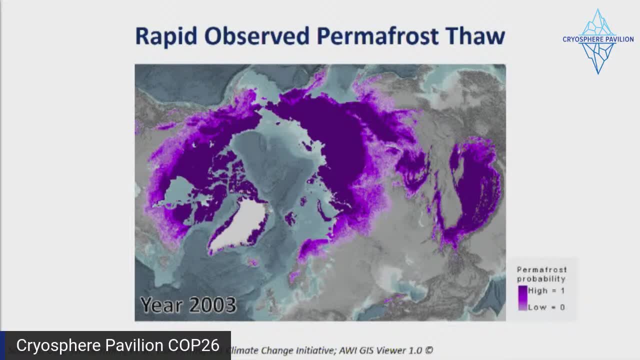 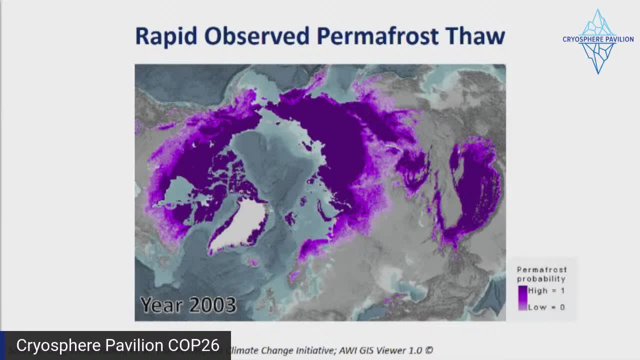 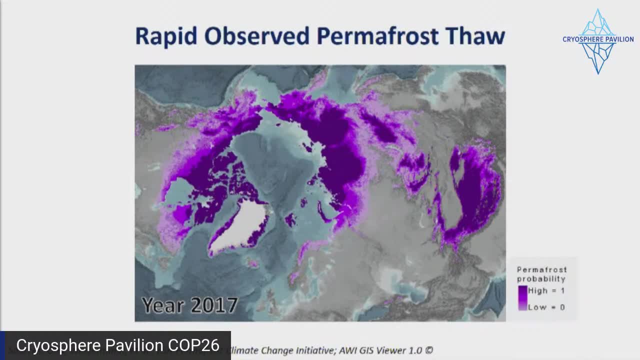 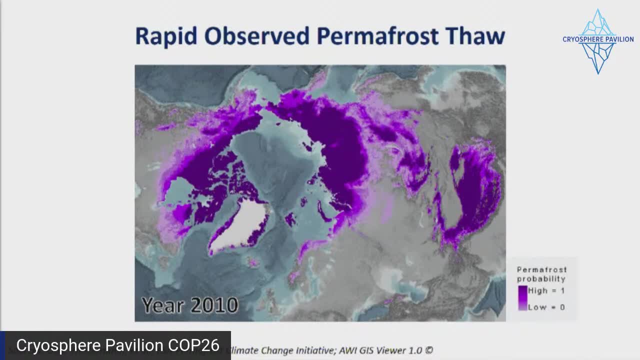 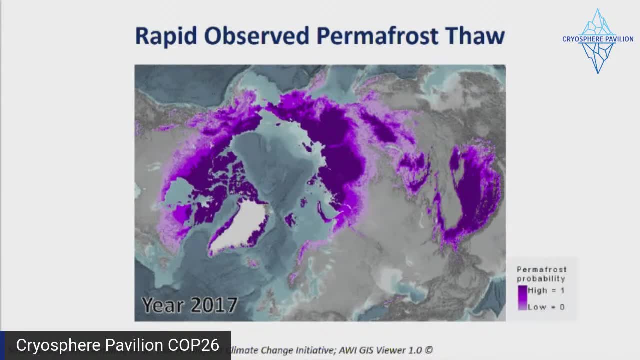 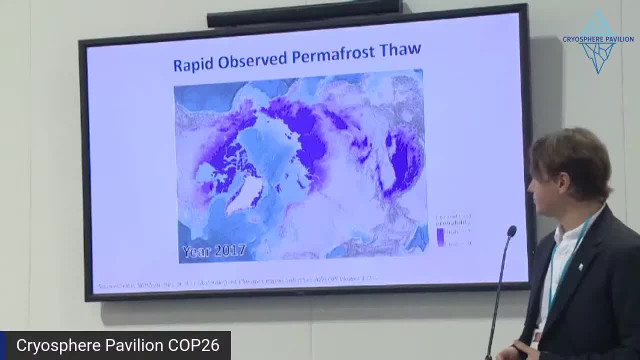 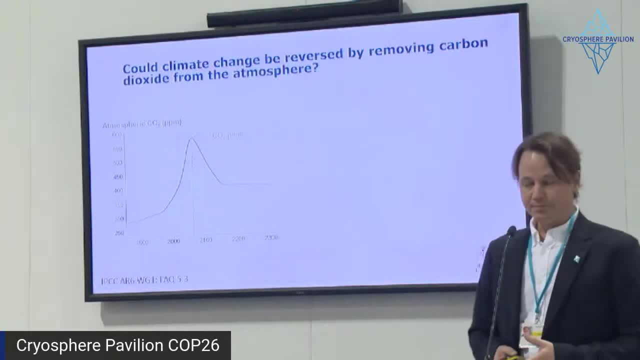 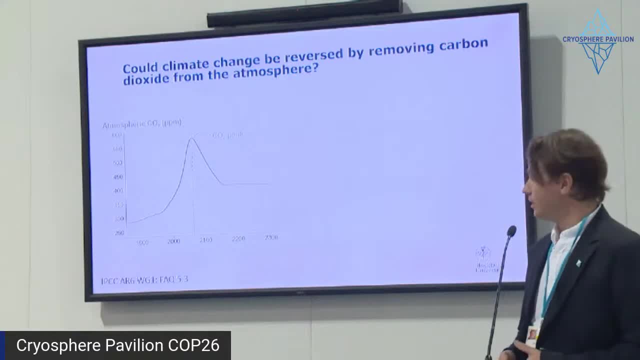 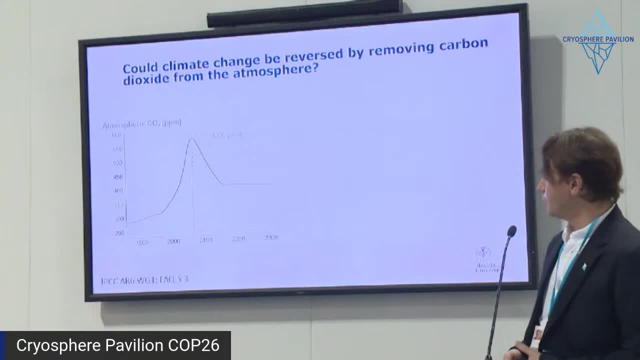 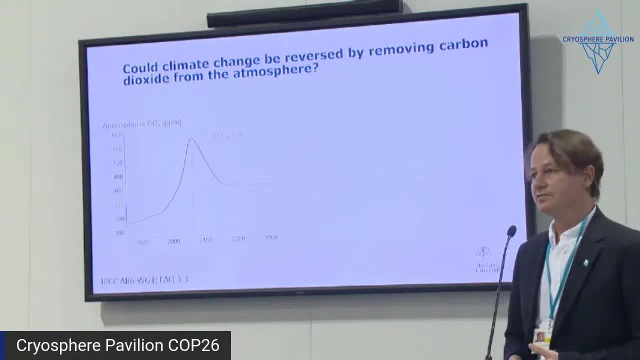 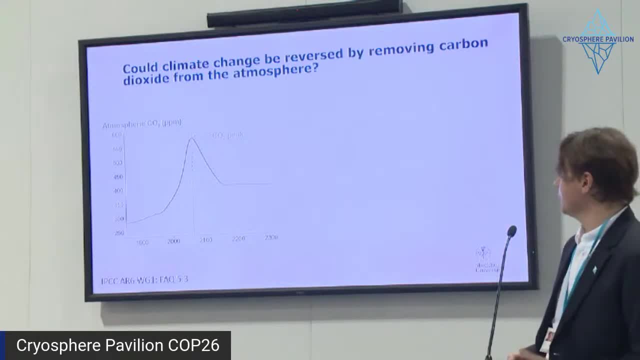 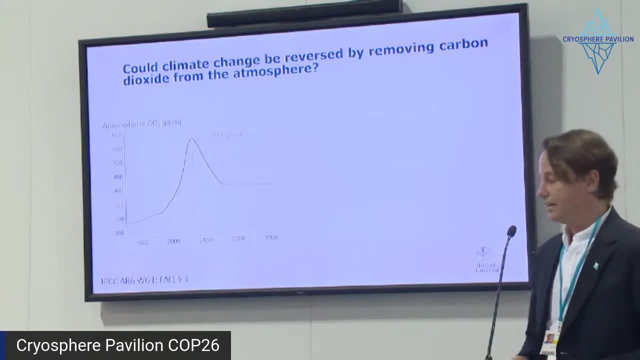 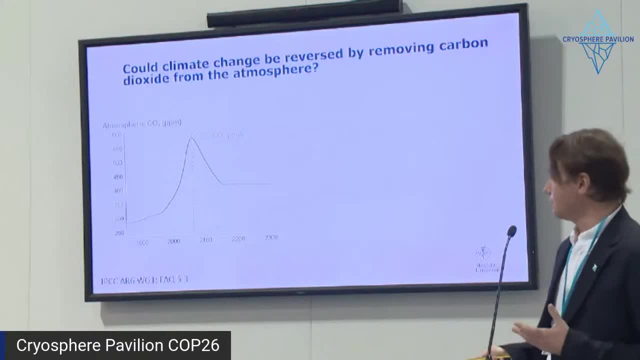 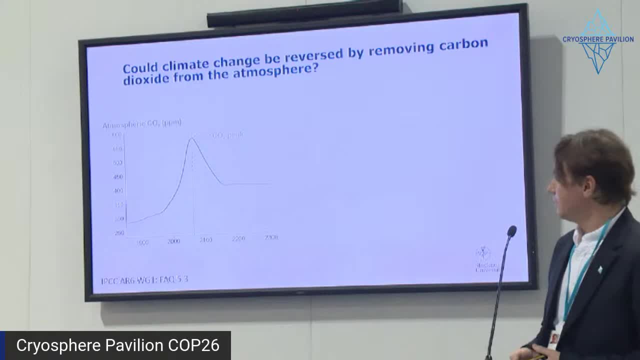 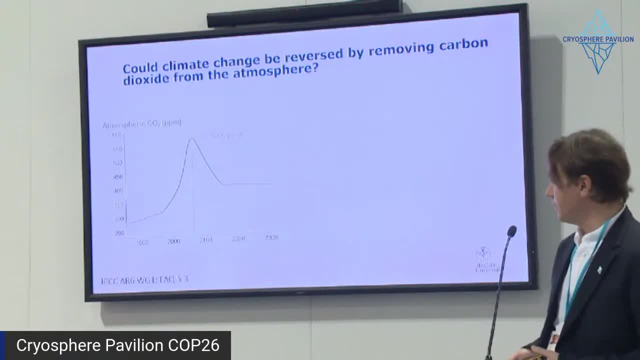 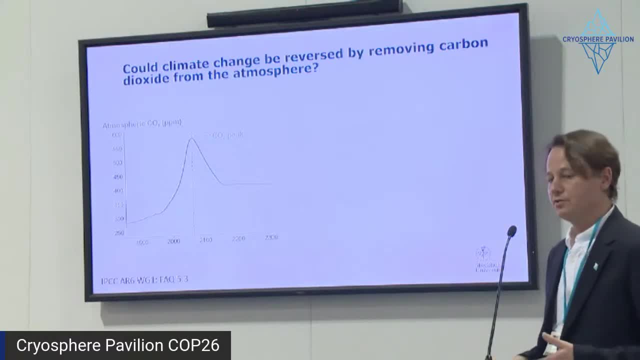 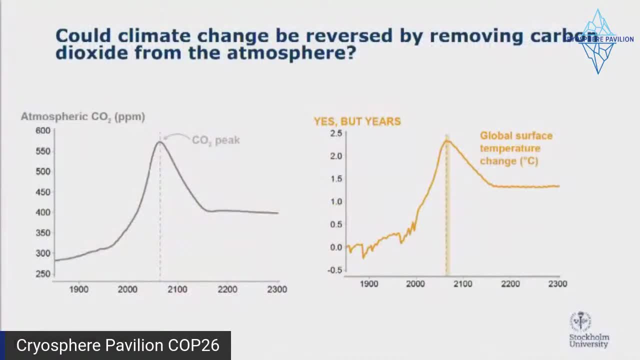 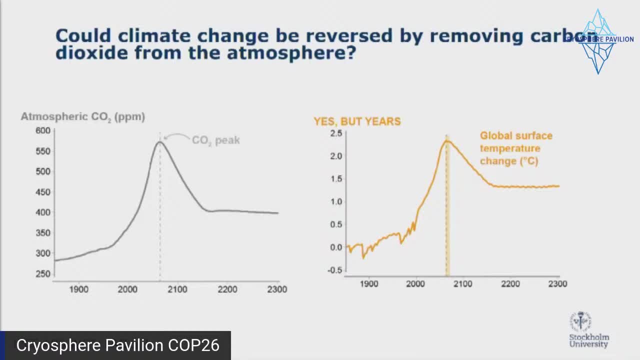 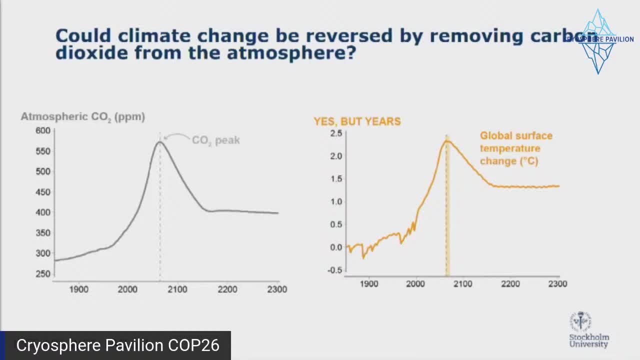 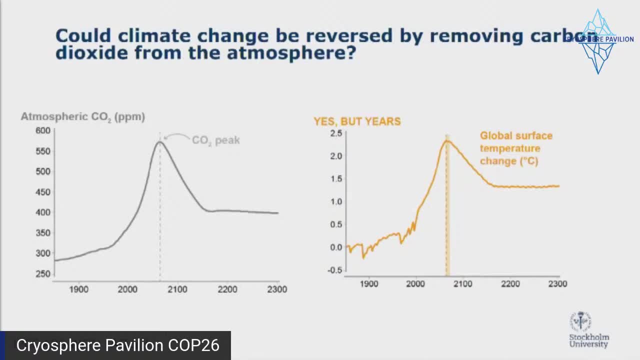 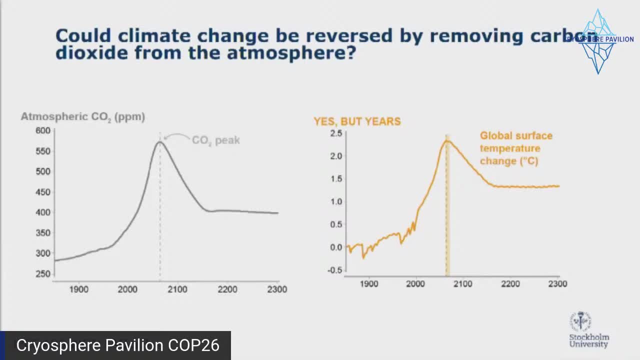 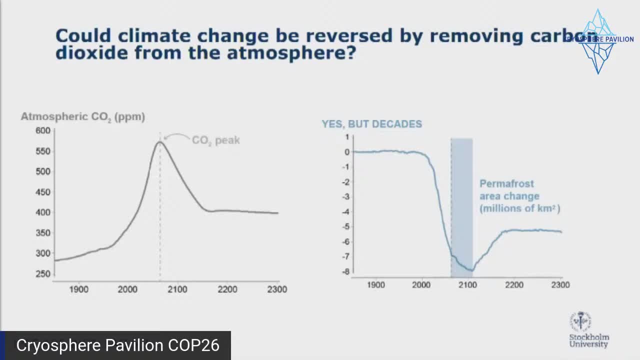 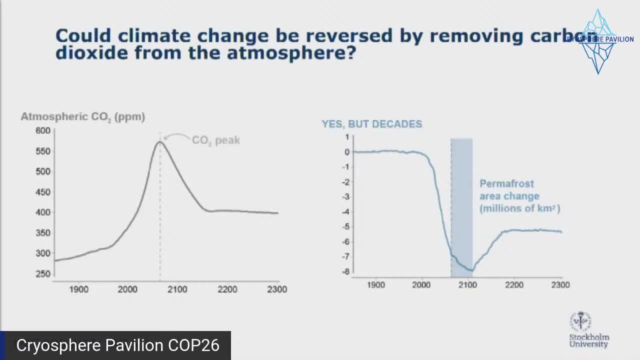 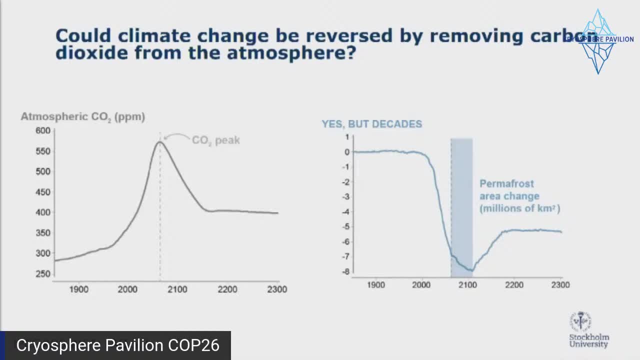 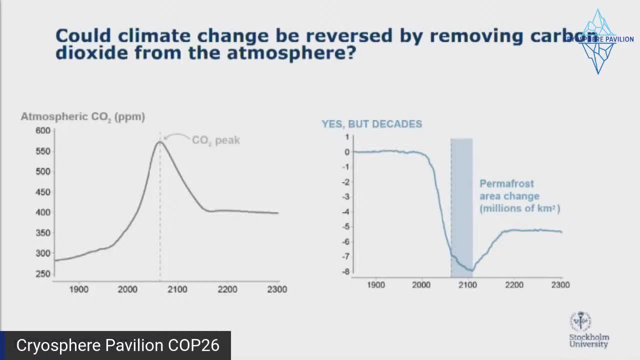 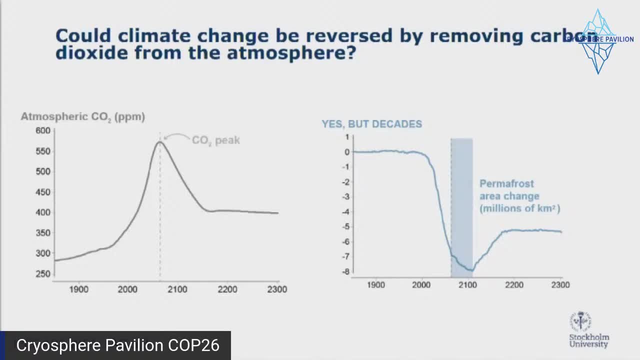 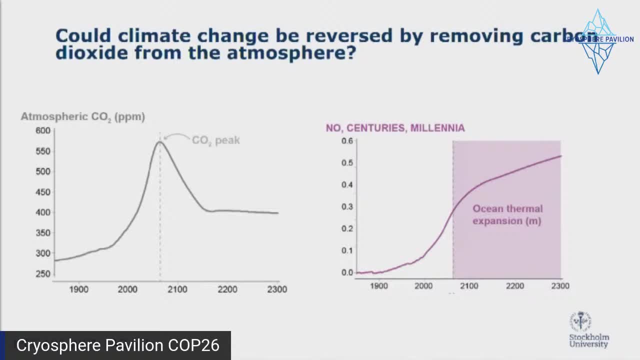 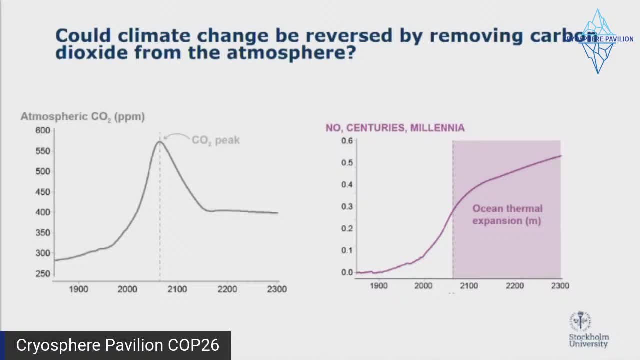 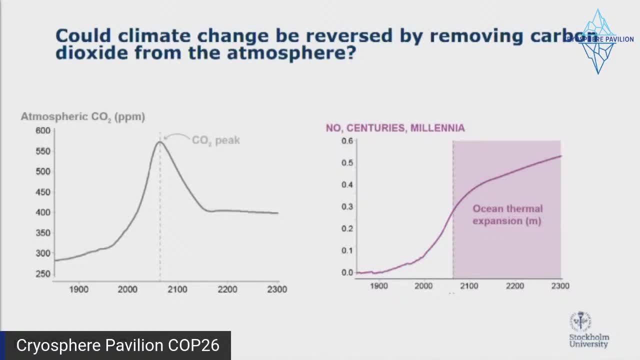 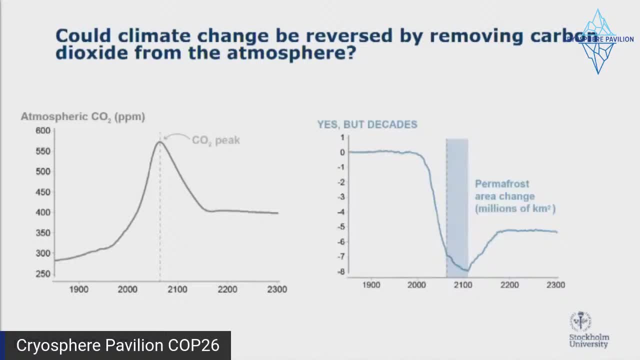 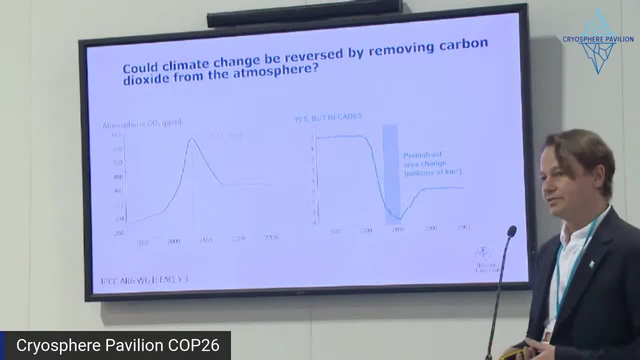 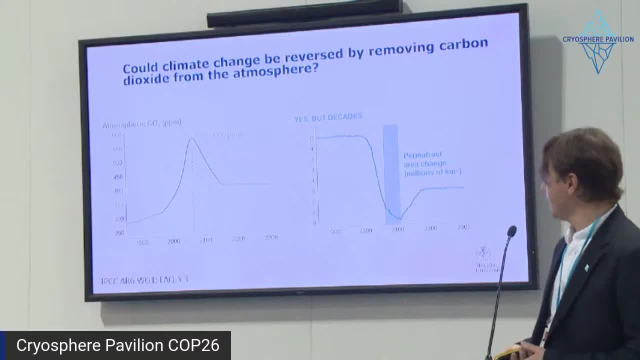 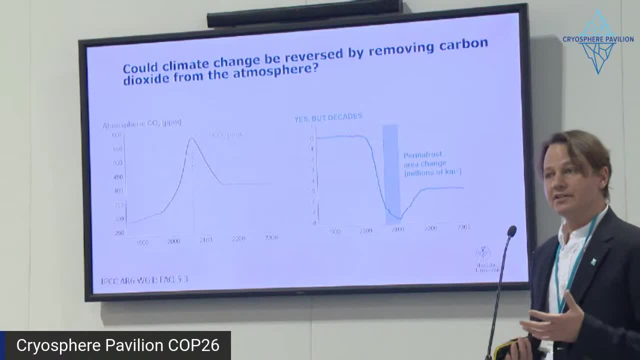 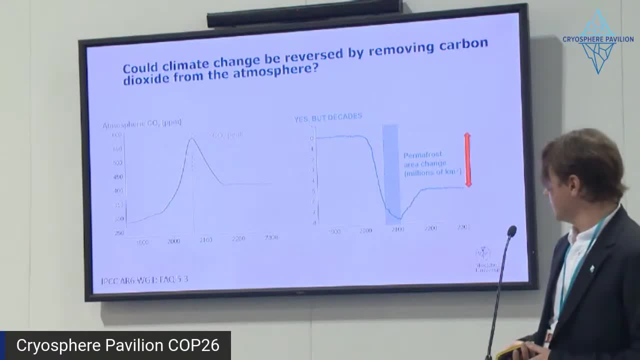 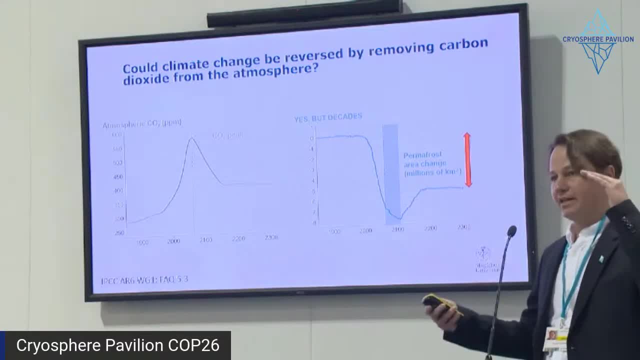 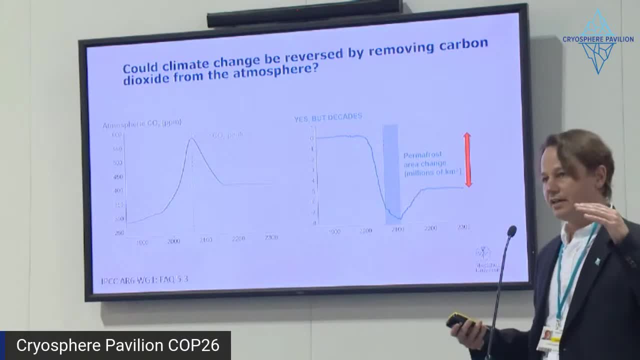 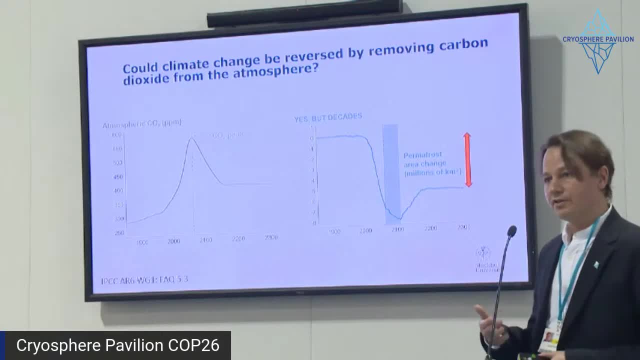 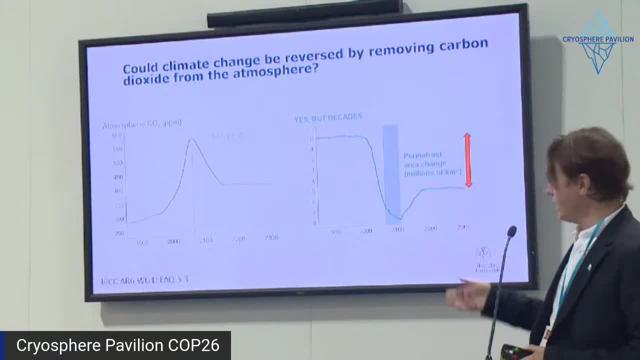 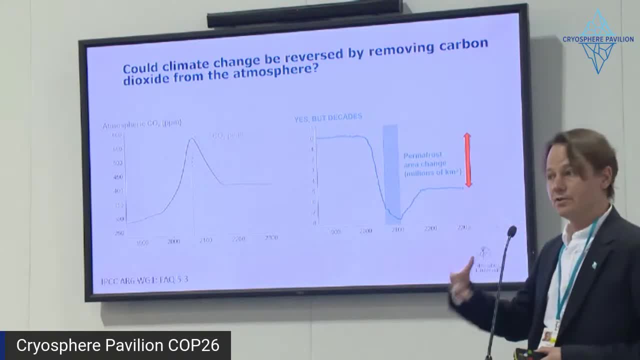 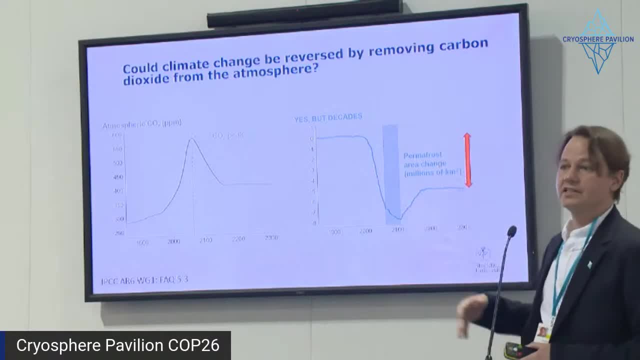 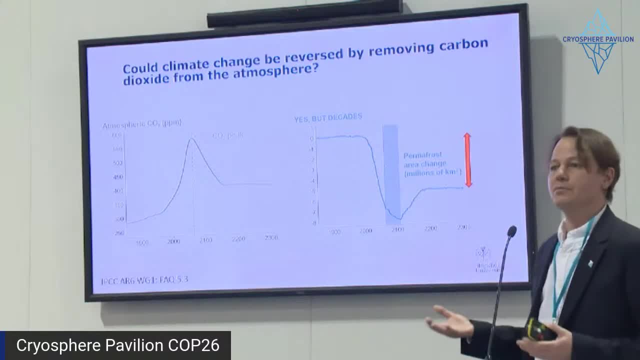 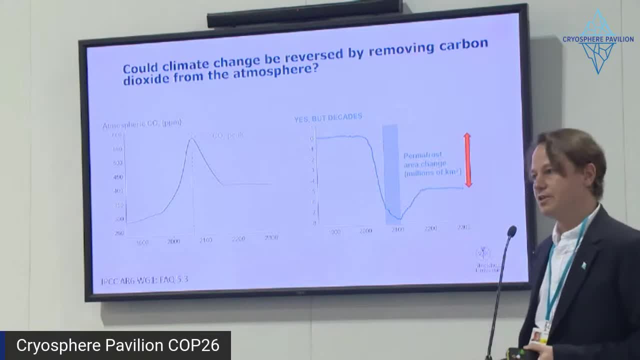 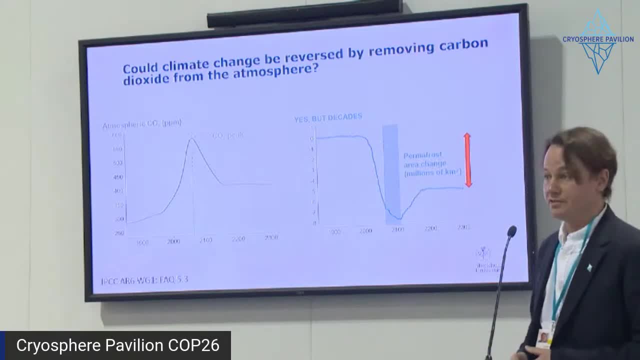 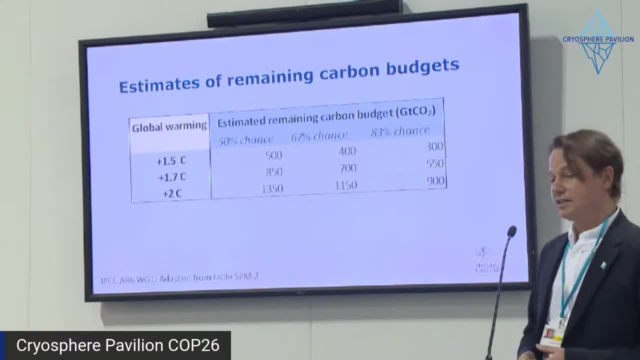 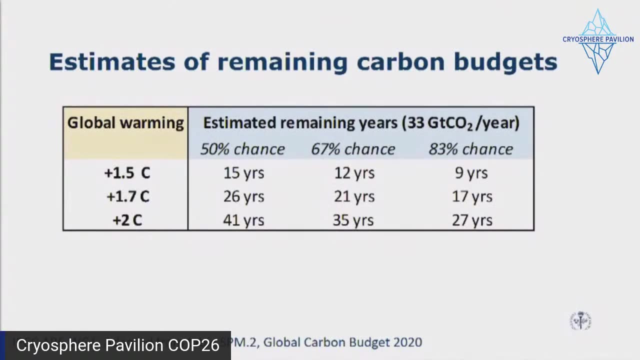 So the IPCC also provided estimates of remaining carbon budgets to stay under different global warming scenarios. So I'm just going to click to the next one where we recalculated this to the amount of years we have left if we assume that emissions stay at the level they are now. So if we look just at the 1.5 degree global warming scenario, 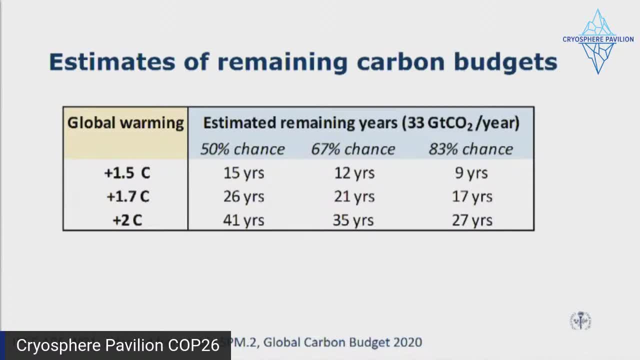 if we want to have a good chance, say an 83% chance in this case, we have about nine years left to sort of meet those targets And for the two degree warming goal somewhere close to 30 years. But it's really rapid action that's needed. 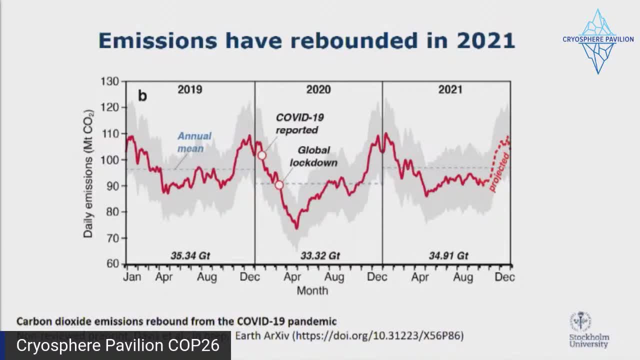 And I'm sort of ending, before I go to the conclusions, with a slide that just shows. this is from a non-reviewed pre-print of a scientific paper looking at carbon dioxide emission rebound from the COVID-19 pandemic. And this is from a non-reviewed pre-print of a 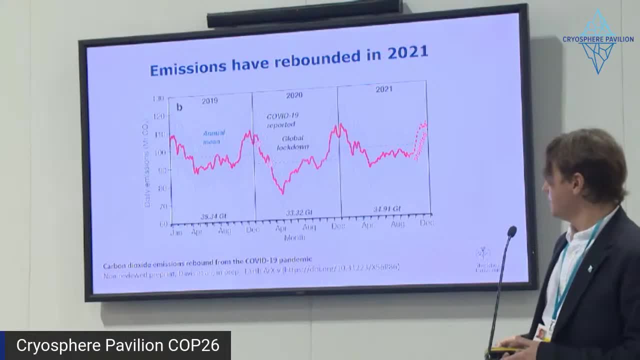 scientific paper looking at carbon dioxide emission rebound from the COVID-19 pandemic. And this is from a non-reviewed pre-print of a scientific paper looking at carbon dioxide emission rebound from the COVID-19 pandemic. You find the reference below here And it just 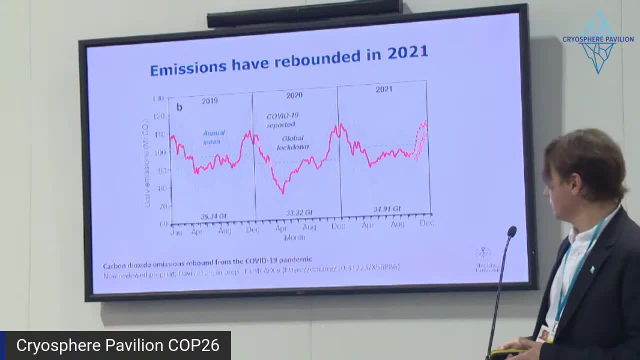 shows that the projected emissions for this year are almost at 35 gigatons, So slightly below 2019, but definitely above 2020.. So if we act quickly, we would still be slightly below 2019. this year We're about 1% below 2019.. So in theory, peak carbon could have passed us already. 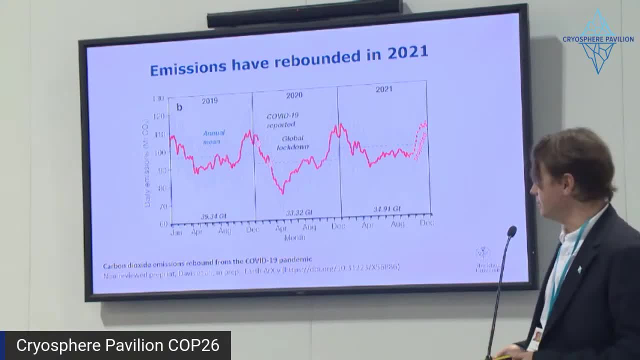 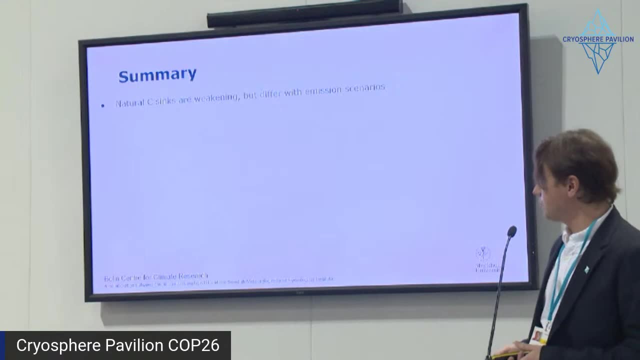 unless we go up next year. So let's hope that that's sort of where we land right. So let's hope that that's sort of where we land right. Summary of the overall talk on carbon cycle feedbacks. The natural carbon sinks of the. 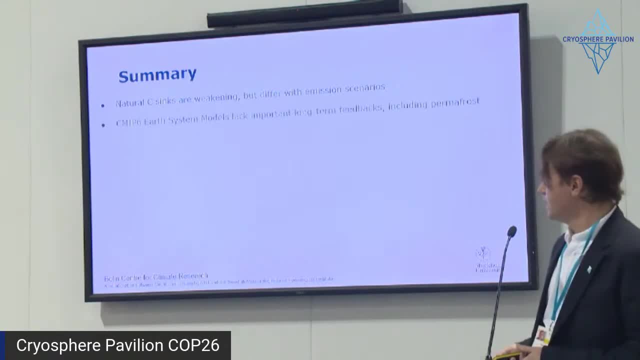 Earth are weakening. They differ with different emission scenarios. CMIP-6 Earth system models lack some really important long-term feedbacks, including permafrost, which is important to note, But the last IPCC report did quantify these missing feedbacks, which is a really good step. 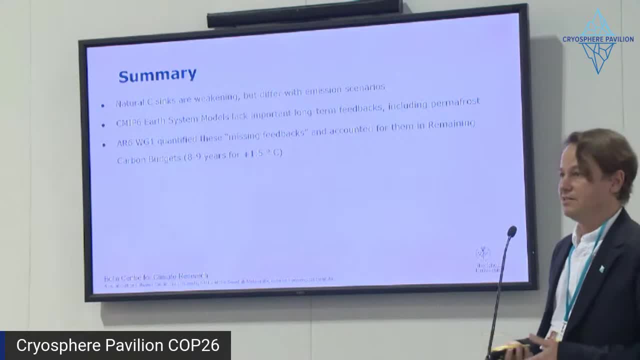 and accounted for them in remaining carbon budgets. We have eight, nine years to stay under 1.5 degrees, But the last IPCC report did quantify these missing feedbacks- which is a really good step, and accounted for them in remaining carbon budgets. We have eight, nine years to stay under 1.5 degrees. 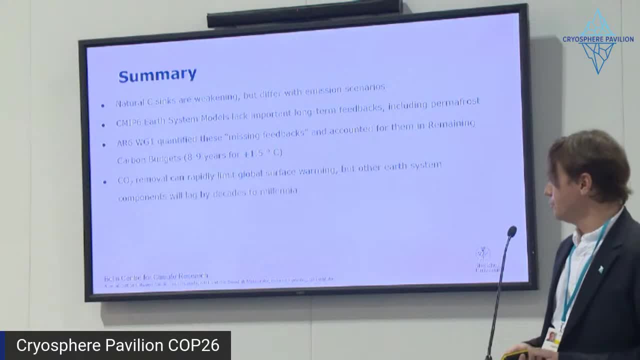 We have eight- nine years to stay under 1.5 degrees. We have eight- nine years to stay under 1.5 degrees And we also find that CO2 removal can rapidly limit global surface warming in the future, but a lot of Earth system components will lag by decades to even millennia. 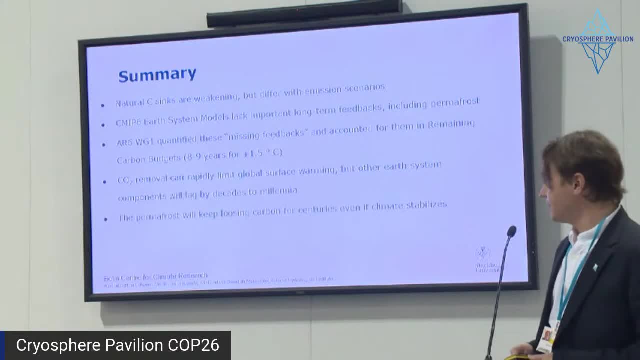 so this is something that we need to keep in mind And, importantly, the permafrost will keep losing carbon for centuries, even if climate stabilizes, which is the really key take-home message we want to have for this session. Thank you. 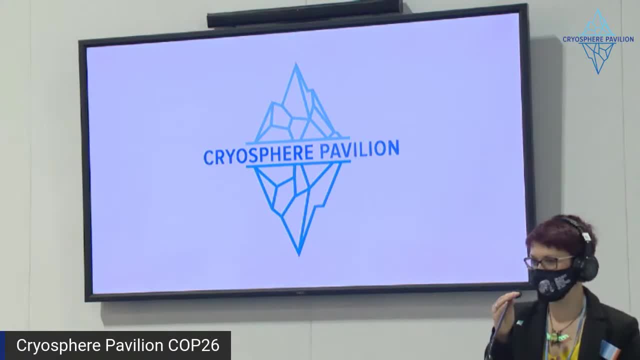 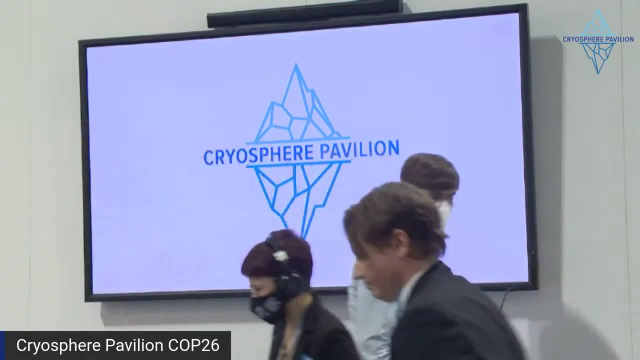 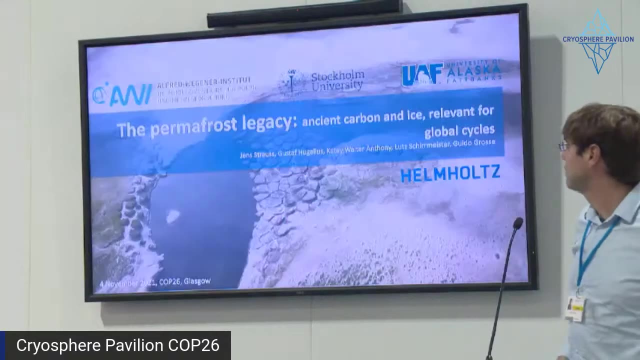 Thank you so much, Gustav. That was a fantastic, a lot of background information for us, And now I'd like to invite up our second speaker, which is Jens Strauss from the Alfred Wegener Institute. Thank you, Hello everybody, Thanks for being here and being on Facebook or wherever you want to stream. 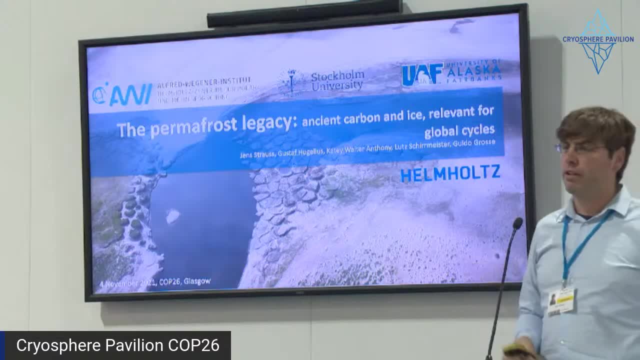 Today I want to talk about the permafrost legacy. So Gustav gave a nice introduction and what is possible when permafrost is thawing and what is happening if it's thawing. And I want to have a look at what's in there and what's the relevance of the ancient carbon and ice. 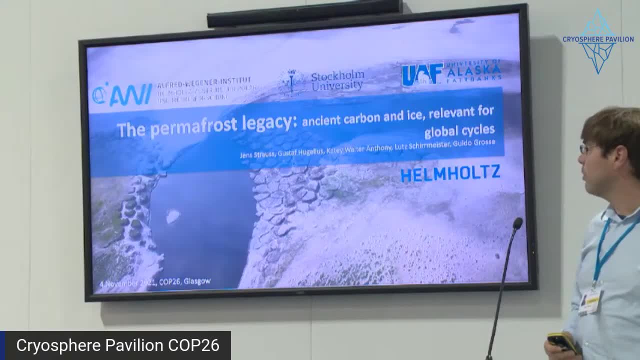 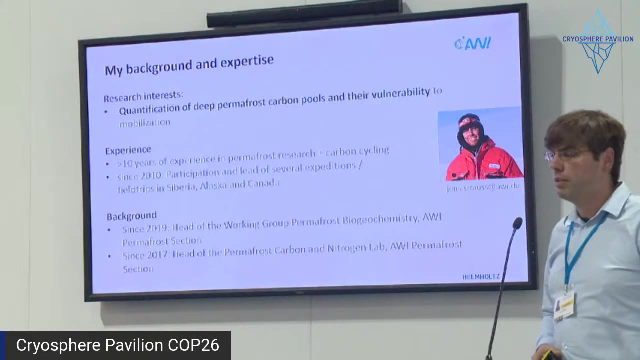 for the global cycles. But this is work with a big group. just name some names here: Gustav, Katie, Lutz and Guido, But of course there are many people involved in this. So my background first. So I'm doing permafrost research since a while, and I'm especially 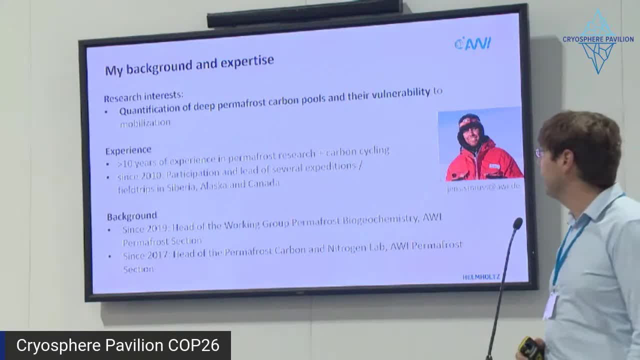 interested in permafrost In the deep carbon and how much is there and how fast it could be remobilized when it thaws. And I do this since many years And also field research is part of my work, So I go into the 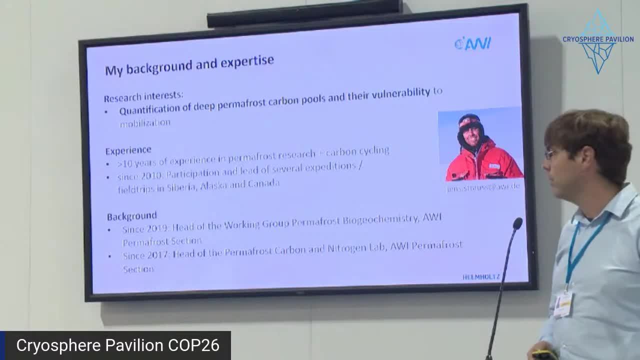 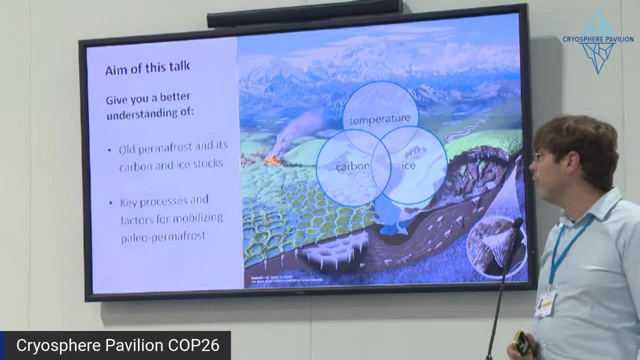 Arctic, taking samples and look how much carbon is there and which quality. So my background is: I'm at the Alfred Wegener Institute, based in Potsdam, and I'm leading the permafrost biogeochemistry group. The aim of this talk is getting you a better understanding of old permafrost and its carbon and its 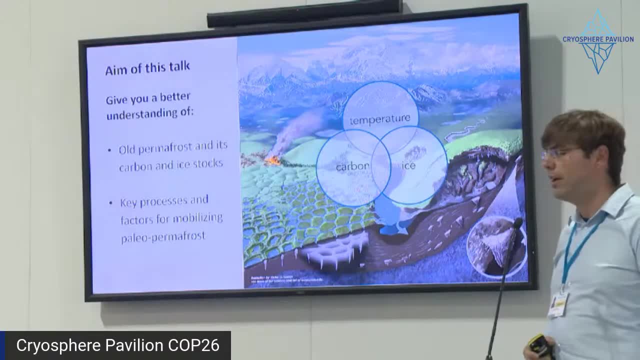 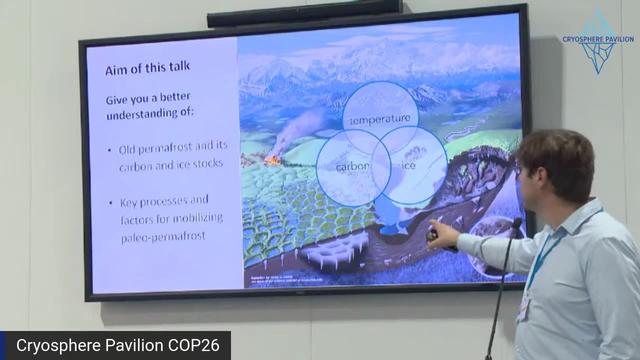 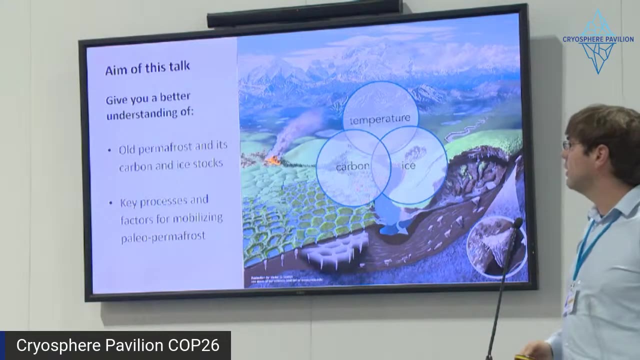 is KATalin. so that's very much because Chapter 87 of the project with cat and I stocks and the key processes which are factors, ask. the factors for remote, I think, is carbon. So you see, here you have the permafrost region is full of ice, it's full of carbon And there's a lot of things going. 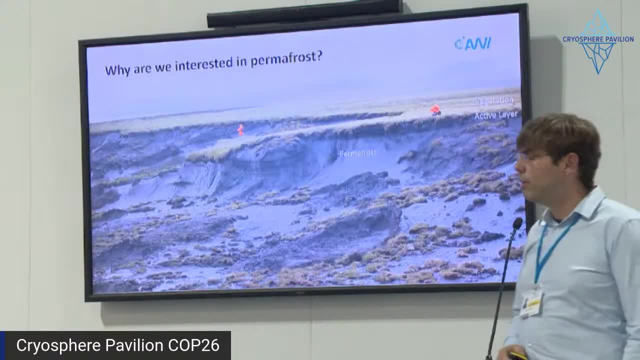 on. so this, this is the aim. But why are we curious about permafrost? I'm interested in permafrost, Of course. permafrost is the beauty. you see it here. there's the frozen ground, There's an texture, ear waxなん mascot. there's cool effects alsoヨтор. 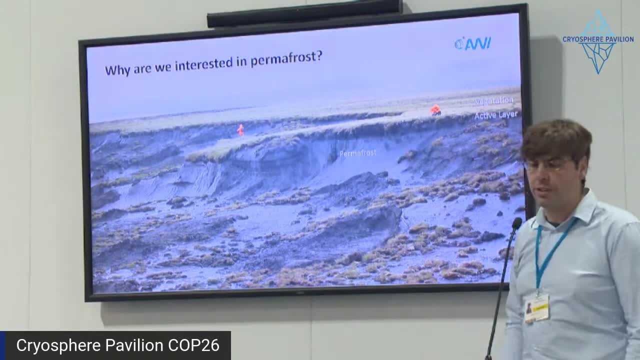 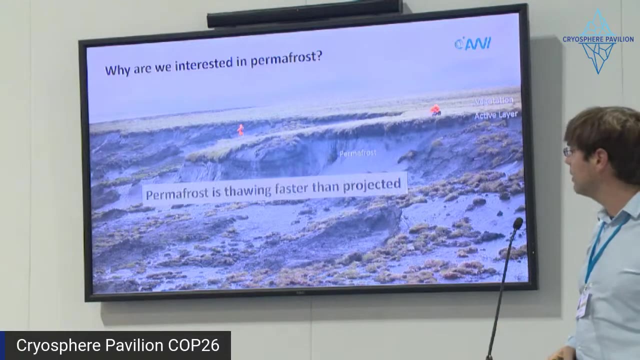 поқ Zheny an length of 8 km. about it attracts permafrostỨ layer which thaws and refreezes every year, So it's a seasonal unfrozen layer and the vegetation on top And of course, there's a lot of process like erosion and degradation going on. So this 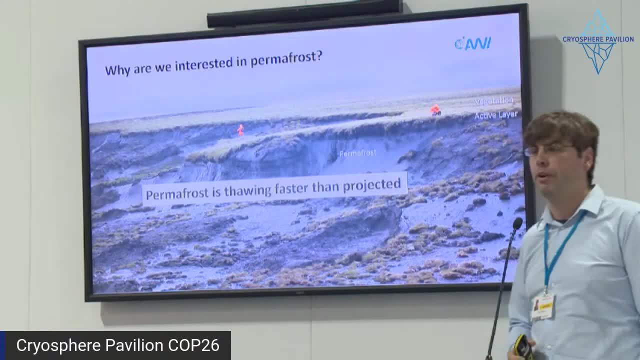 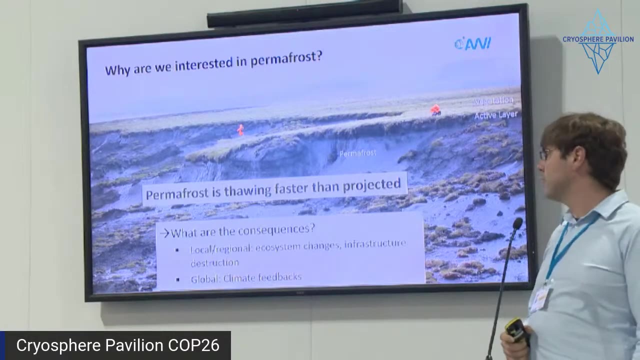 is exactly the point. Permafrost is thawing. It's thawing faster than we expect. Gustav said that the example for the high Canadian Arctic. it's 70 years faster than we thought before And this has huge consequences, Consequences on the local, regional area, but also for the global. 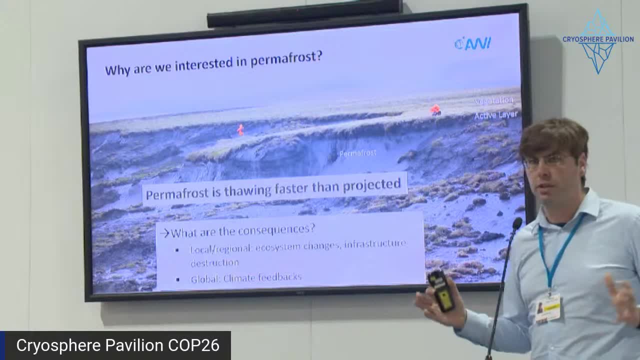 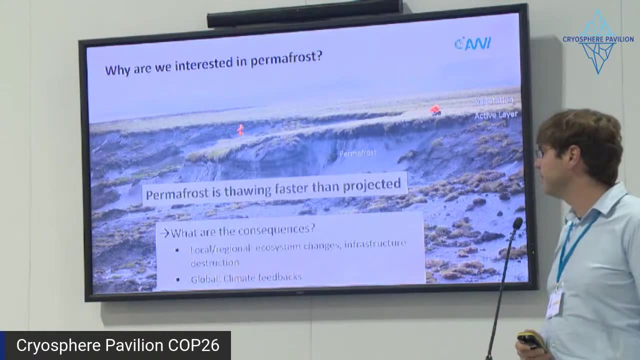 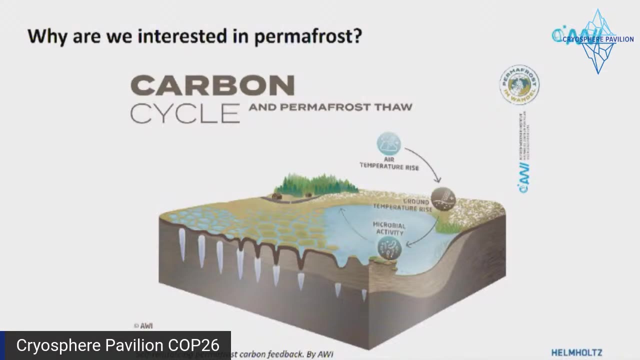 feedback. So locally its ecosystem changes, problems with infrastructure on top of permafrost, And for the global it's the feedback which are like here- a nice animation- the permafrost carbon feedback. So air temperature is rising And this causes more warming to the ground. This causes 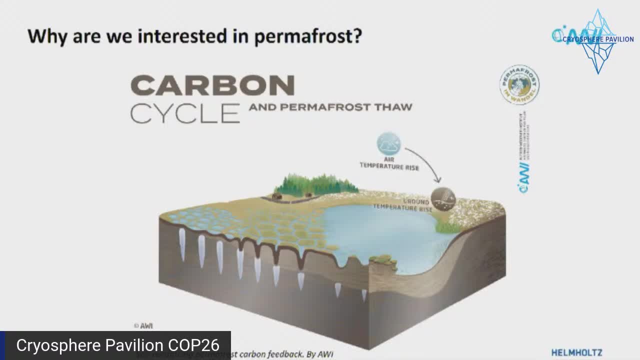 thaw And with thawed material it causes more warming to the ground And this causes more warming to the ground, And this causes more warming to the ground And this causes more warming to the ground. And with thawed material you can have microbial activity And this again releases carbon and. 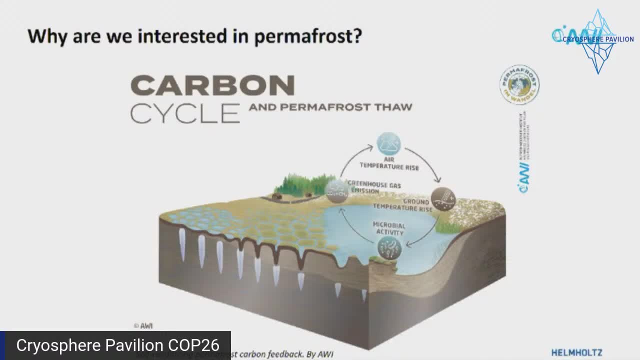 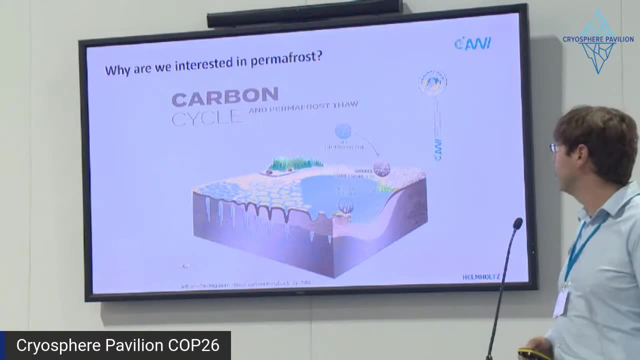 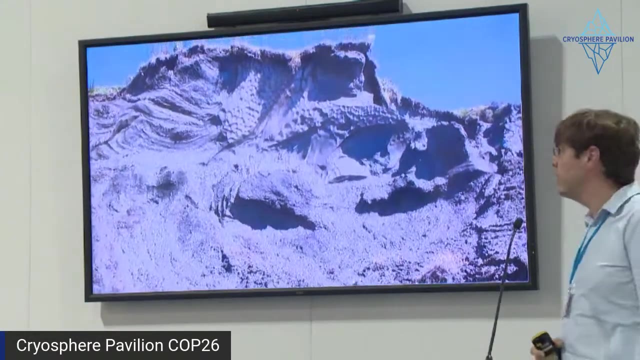 carbon as CO2 and CH4, methane and carbon dioxide, which again leads to warming, So this is a self-enhancing feedback. We call it the permafrost carbon feedback, as I said before, And here you see a video of this carbon from a Yiruma, which is a very ice-rich permafrost. 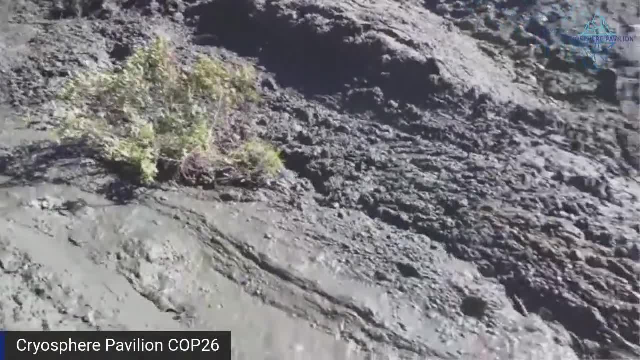 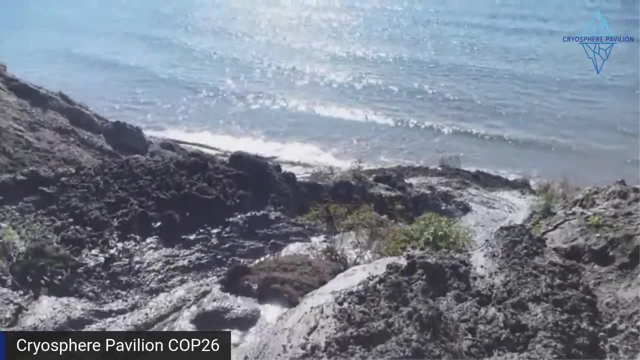 degrading on a sunny day. This is Alaska, Baldwin, Baldwin Peninsula, And it's rippling and dripping and dropping And there is carbon you see there going down into the ocean. So there's no river behind that, This is just the water coming out of. 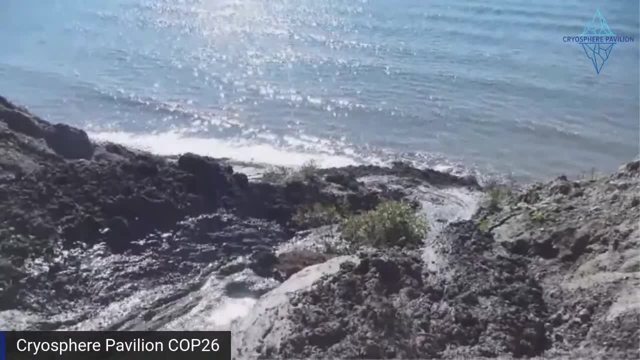 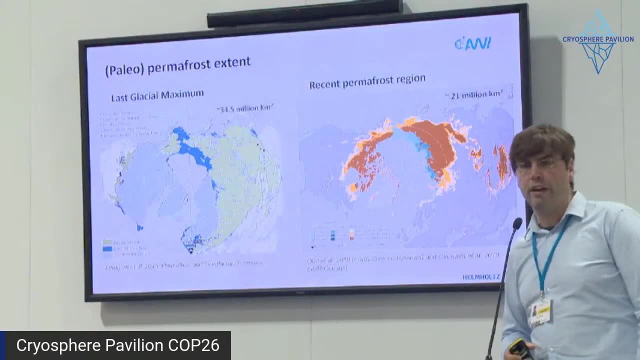 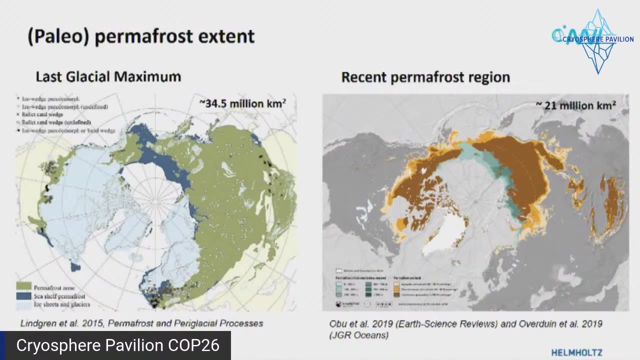 the icy wall you saw before And this is where we have been during the last ice age. This is the permafrost extent from a paper from Amelie Lindgren from 2015.. You see, all the green areas there are, or were, permafrost during the last ice age. So it's about 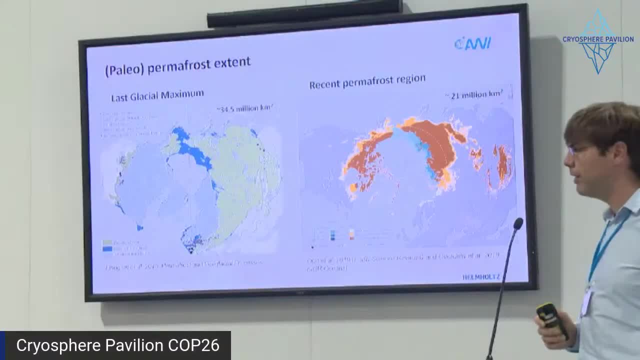 35 million square kilometers, including the subsea permafrost, the now subsea permafrost areas. on the shelves which you have a talk by Paul Overdeen this morning Today. this is the recent permafrost region. We have 21 million square kilometers, So this is a huge reduction of the permafrost area. 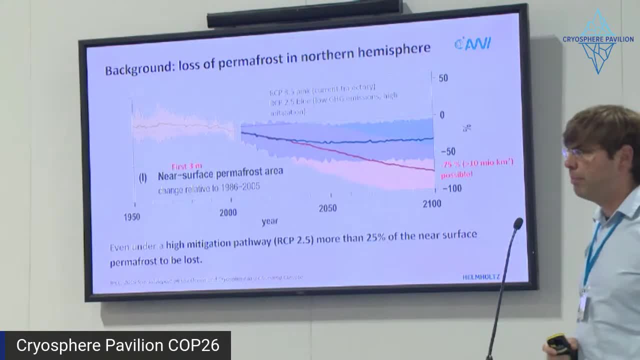 And we expect even more permafrost. So this is IPCC 2019 special report graph. On the bottom you see the years starting from the 1950 going to 2100.. So the future and the point here. So there are two. 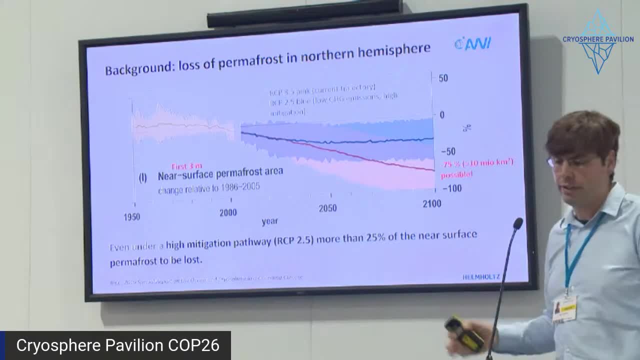 scenarios: the 8.5, which is the current directory. So the- if we go on as as we do now, and the 2.5 is the mitigation scenario with low permafrost. So this is the current trajectory. So the- if we go on as as we do now, and the 2.5 is the mitigation scenario with low permafrost. So going the emissions and high mitigation. Even in this lower scenario, we see here a loss of the permafrost area of more than 25%, And if we assume like high emissions, we can lose up to 75%, which is more. 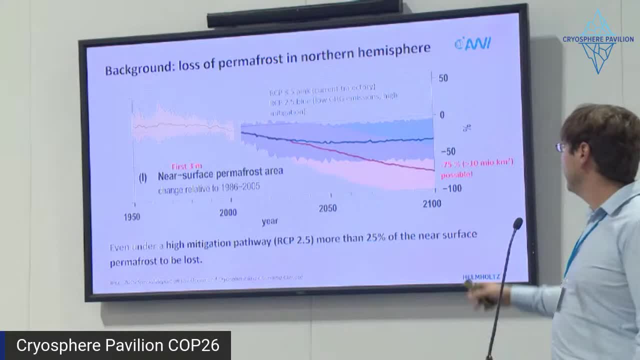 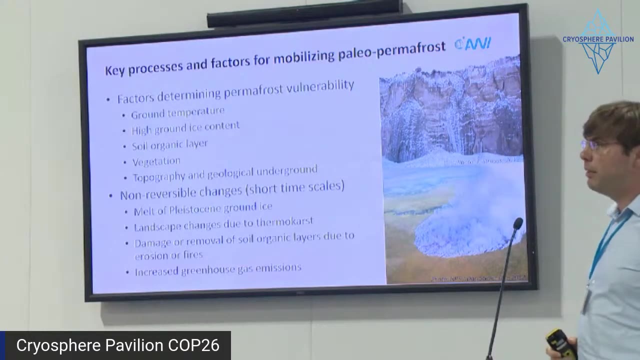 than 10 million square kilometer up to the end of this century. This counts for permafrost in the upper three meter, to make this point, Michael Alexander. So what are the key processes for remobilizing the permafrost? As said before, this is ground temperature. 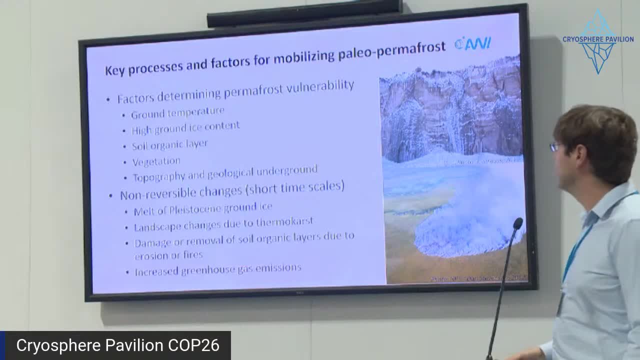 Ground temperature is affecting, of course, the ground ice content. You see here on this picture again Yiruma permafrost, like in the video before. there's a lot of ice. This is this. It's an ice wedge and sediment in there. 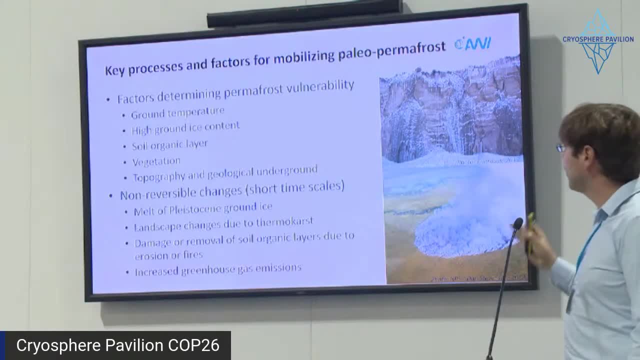 Of course you have soil organic carbon or soil organic layers in there. There's vegetation and topography and geological background which is somehow key for the permafrost vulnerability in future, And we have non-reversible changes on short timescales, like the melt of the permafrost. 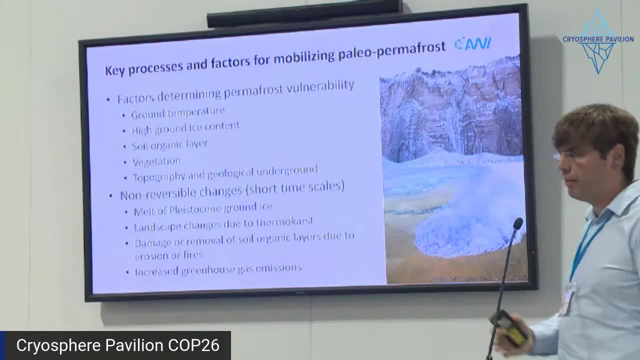 ice is happening and you can't build it up again, even if you have a century or two centuries or more, And you have landscape changes due to thermocast processes. I will show you thermocast in a minute. You have damage or removal of the soil organic layer. 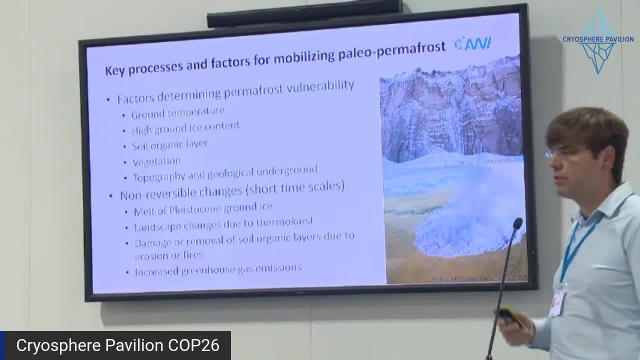 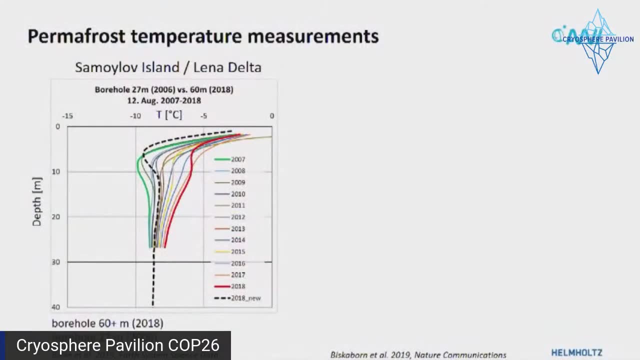 And there is a lot of greenhouse gas emissions. if you have this tall, That is what we see. We try to measure the ground temperature in permafrost. Here you see a borehole that's 27 meters, drilled in 2006 on Samoilov Island, which. 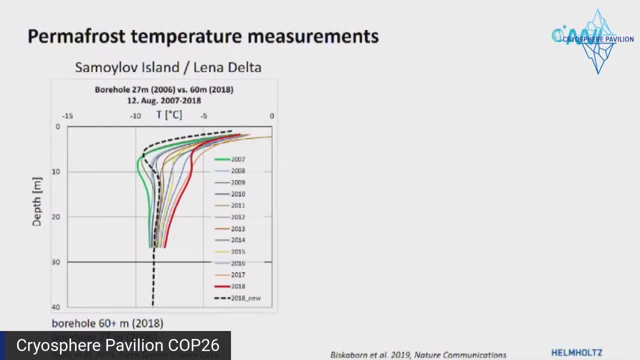 is in the Lena Delta Research Station. So you see, here there's a rise in temperature. So in green is 2007 and in red it's 2018.. So that's a huge rise in temperature. we measured there In 2018, I, with colleagues, drilled another hole for 60 meters to have an even deeper. 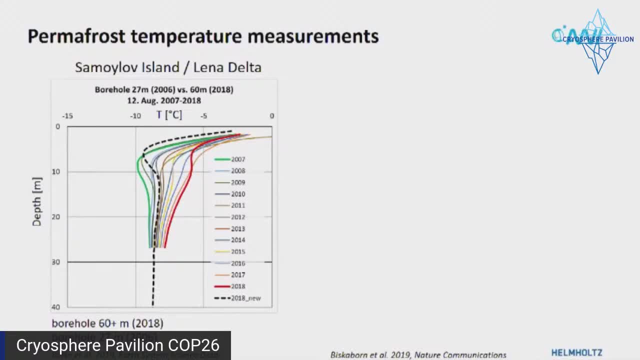 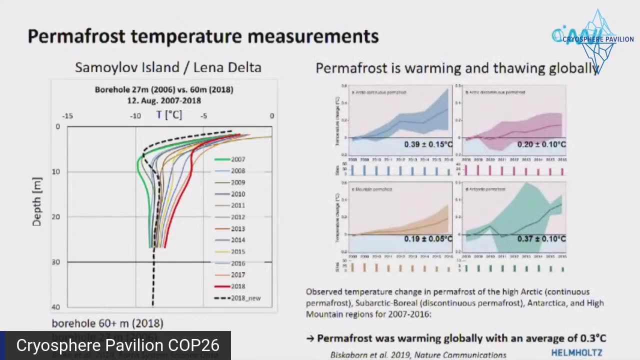 signal out of the permafrost in the future. So this is just the dashed line here. We don't just have this year, but there will be, of course, measurements, And this is not just a thing we see for Samoilov Island. 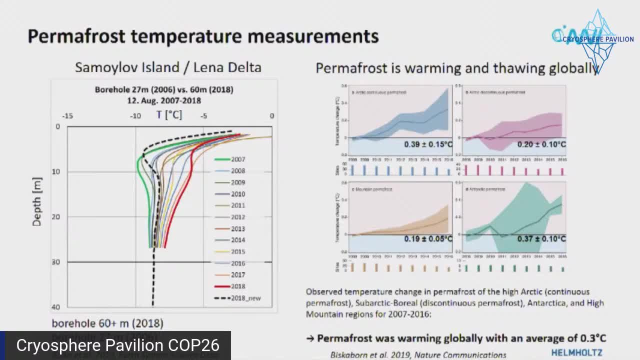 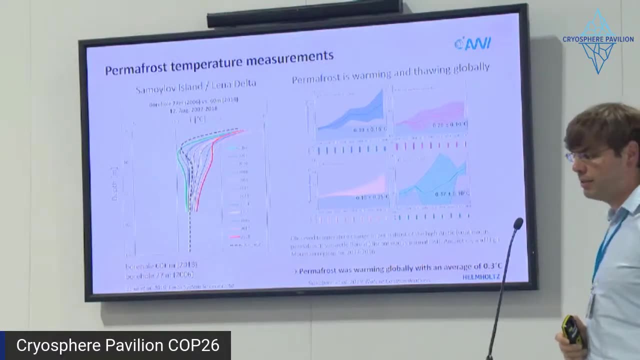 We see this everywhere. We see this in the Arctic, We see this in the discontinuous permafrost a bit south of the Arctic. Then we have this in mountain permafrost and even in the Antarctic. So everything is warming and it means it's 0.3 degrees Celsius in the last decade. 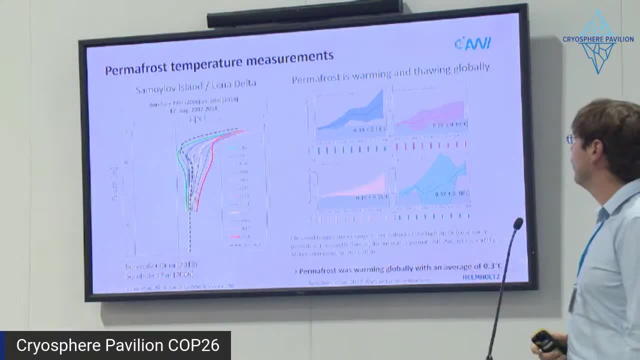 And for the Arctic it's the highest. It's nearly zero degrees, It's nearly 0.4 degrees warming since 2008.. So this is quite an alarming signal And because this temperature is affecting the ground ice, So the ice legacy- 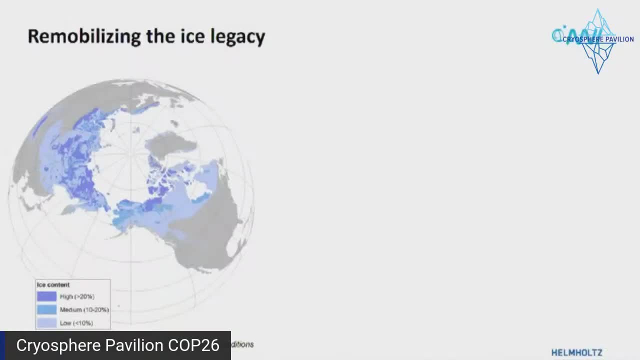 Here you see a map by Brown from 2000,, from from 1989, 98.. So there's ice. There are areas with high ice content, medium ice content and low ice content, the permafrost, obviously. 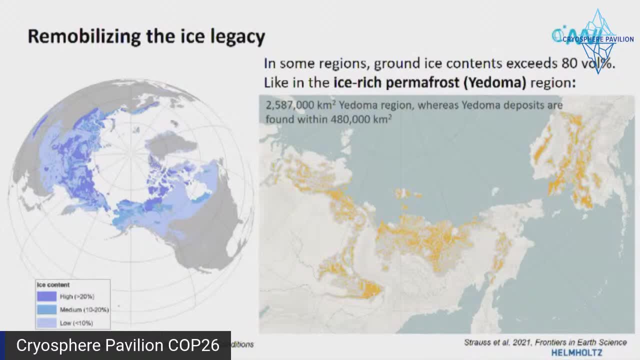 Also some areas like the Yeruma region, where there's a huge amount of ice and a huge amount of carbon in there. Up to 80% of these deposits can be ice And up to 80% of this can be then thawed out and melt and be gone then. 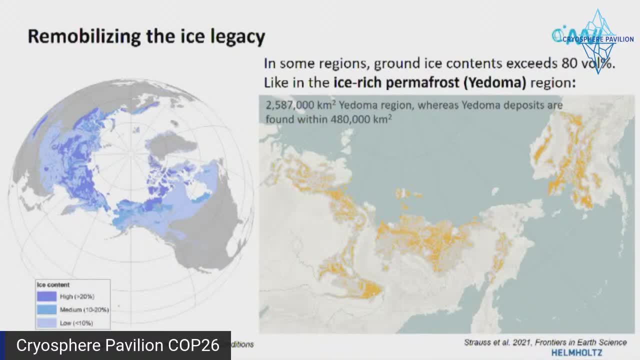 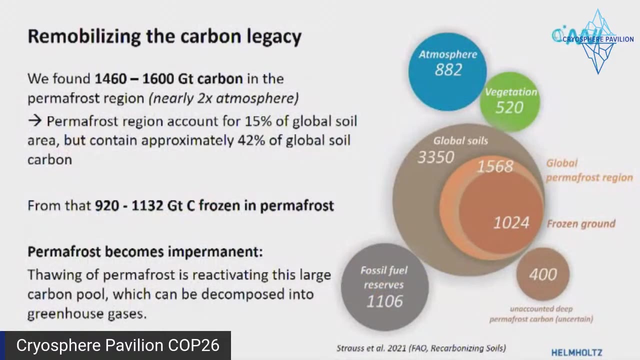 So in this area here in yellow you see, it's around 500,000 square kilometers in Russia and in North America. So this type of permafrost is very vulnerable for changes. Yeah, By uh temperature, ground temperature rise. uh, in this permafrost there's also a lot. 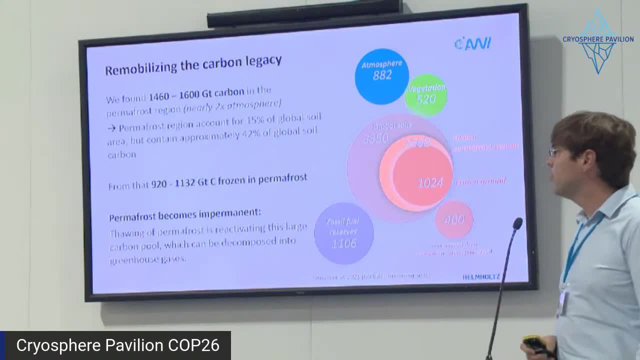 of carbon. We had this before. It's up, So it's up to 1,600 gigatons carbon, which is nearly twice the amount of the atmosphere, And there is a and permafrost has just 15% of the area of the global soils, but it's. 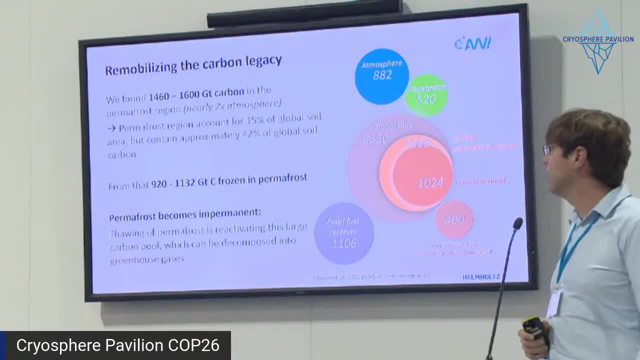 stores uh 42% of the global, global soil carbon. Out of that, Yeah, There is um nearly 1,000 gigatons frozen into permafrost. So this is actually the permafrost which is vulnerability- uh, vulnerable for future. 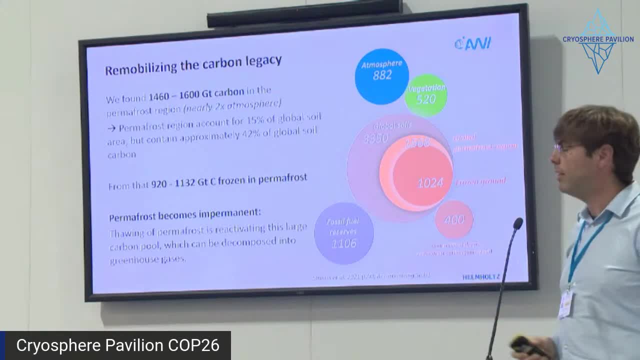 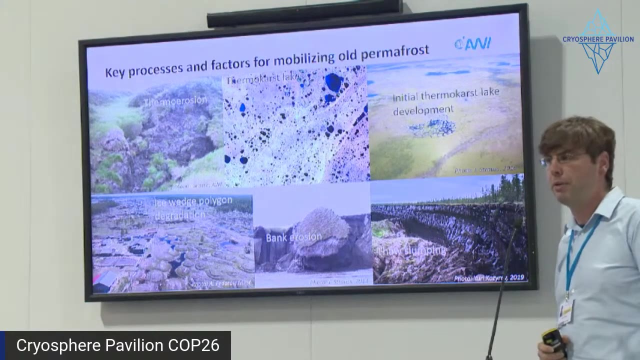 thaw, And this uh is a likely scenario because permafrost becomes impermanent with uh warming, as you have seen before. So these are the key processes here in images for re-mobilizing the deep carbon in the deep permafrost. 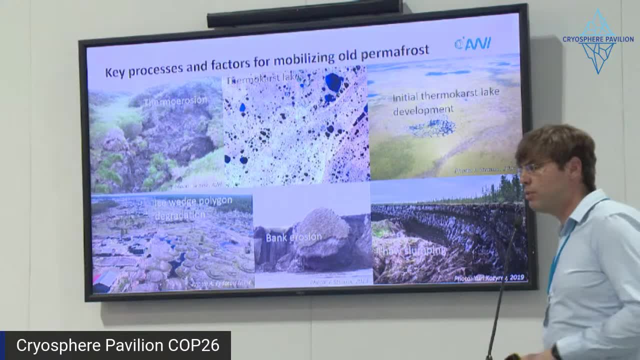 Yeah, And then these are over there. Then you have degradation of ice veggies, And this degradation of ice wedges makes the bumpy ground. So this is in Shrub Cha. This is an an village in Yakutsa, So there's a big problem with ice, which saw and and uh, surface subsidence. 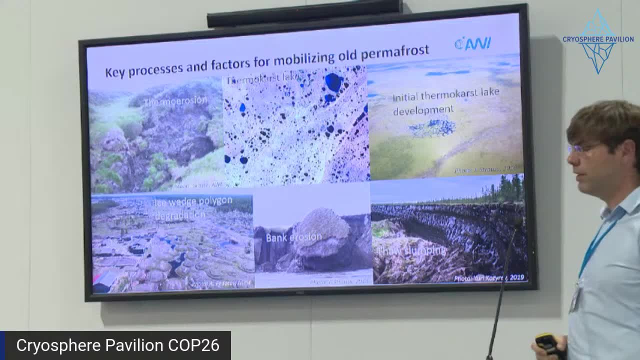 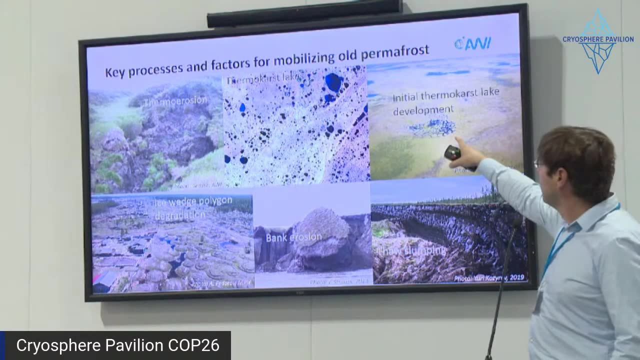 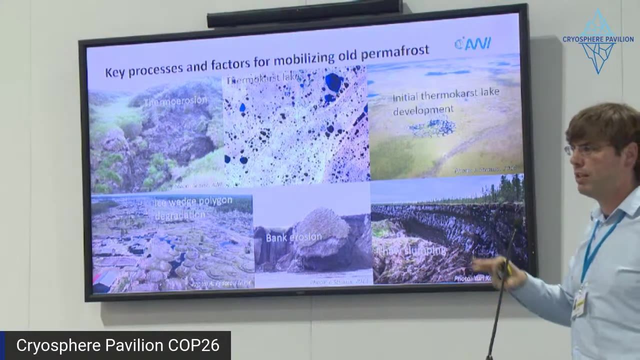 But we have uh, bank erosion, river erosion, um coastal erosion, and this is also ice vegetation, leading to thermocross, Right Yeah, And BSC. there are thermokost lakes everywhere, so this is a local process, but actually it's everywhere, so it. 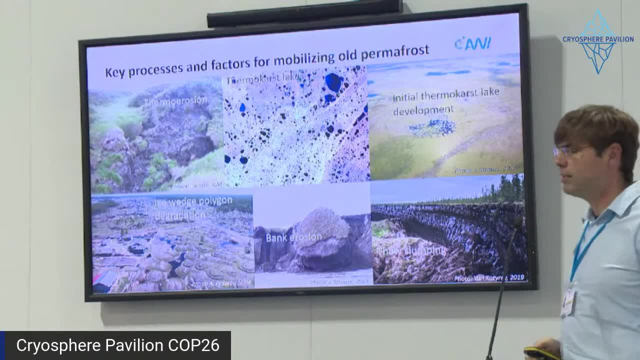 is like: yeah, it is possible to remobilize a lot of carbon with the thermokost processes. and this here is like: this is the Batagai mega slump, which is also in Yakutsia. yeah, this, this wall here is about 60 to 80 meters deep, so this is quite a, quite a big, big thing. 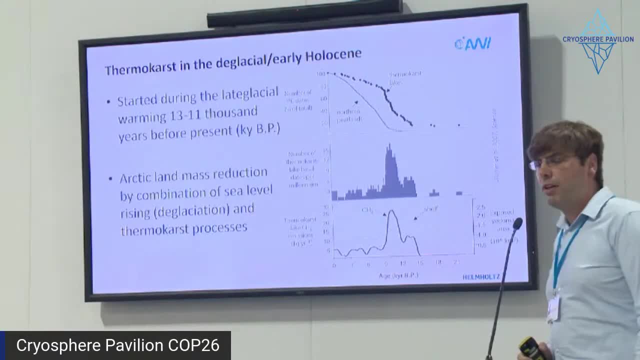 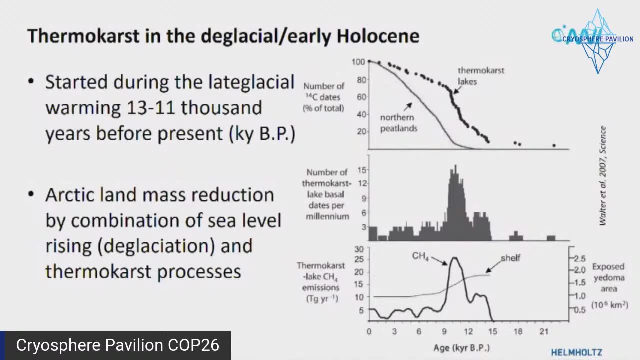 Thermokost is not a new phenomenon. it was there before and it was starting during the late glacial or deglacial periods in 13 000 years before today. you see here on this graph, this is the age and this is the transition from the glyphosate to the Holocene. so there were a lot of 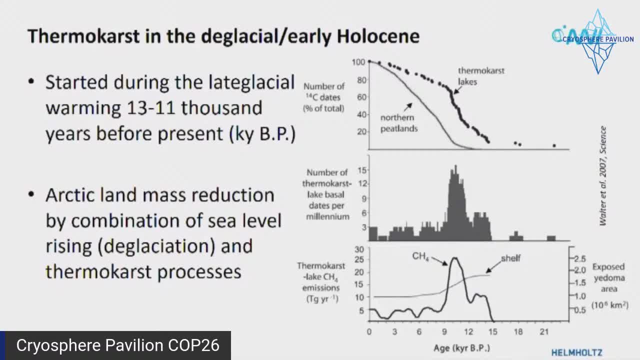 thermokost lakes initiated in this time. here it is here, and there was a arctic landmass reduction by a combination of sea level rise and thermokost processes. so all of that, this is not a new phenomenon, but it is still working and it's still emitting greenhouse gases, and this is how it works. so, being the early Holocene there. 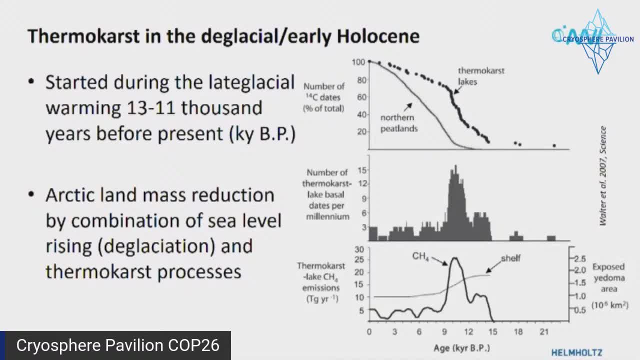 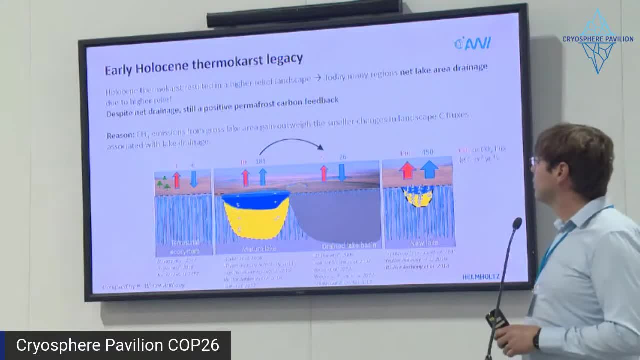 was thermokost, and this thermokost was cutting into the, into the surface, leading to a higher relief. right today we have this higher relief because the thermokost processes have been around since a while and there is more net drainage, but still there is a positive feedback of thermokost. 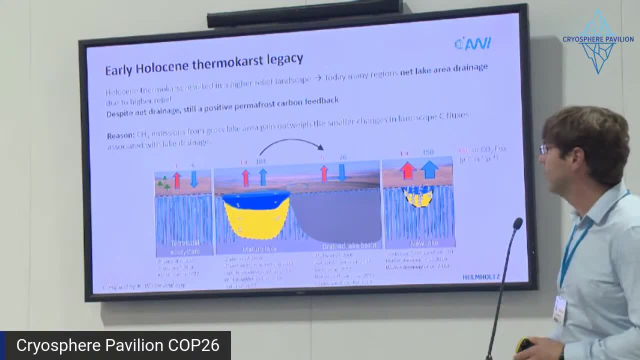 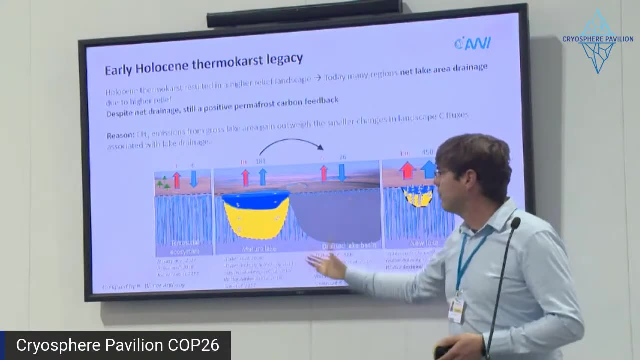 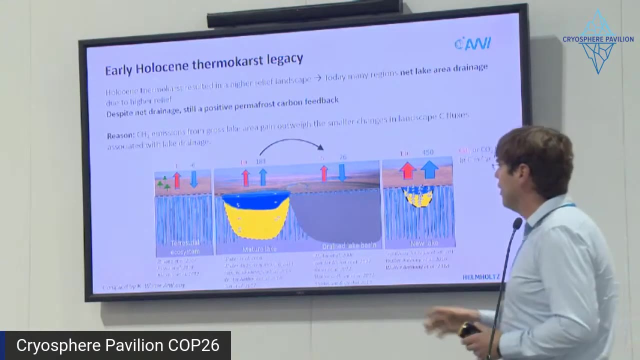 so there's more going out than going in. the reason for that is here. so you have here this. you have this frozen, unfrozen ground, the talik we call that. below you have production of greenhouse gases. if the lake drains, it looks like this and you see here. 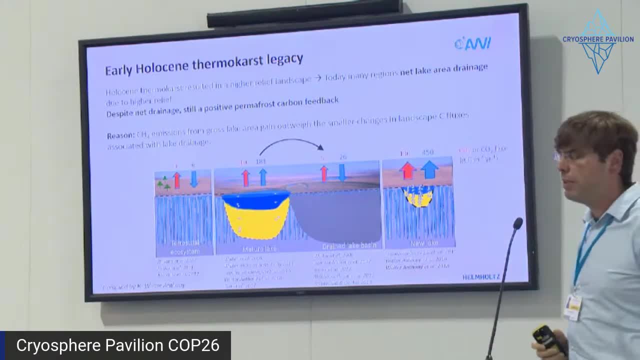 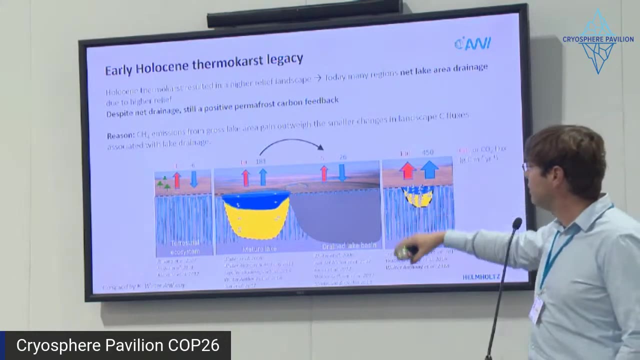 in red and in blue the fluxes of co2 and methane anyway. so ch2 or methane emissions from the leg, from the new lakes or the old lakes, outweighs the reduction of the flux when it's drained. so it's still a positive feedback, even though more lakes are drained today. 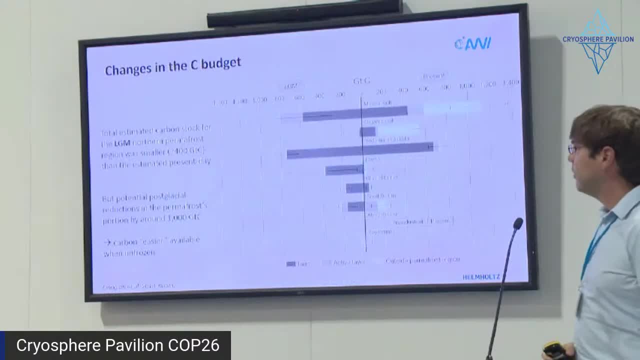 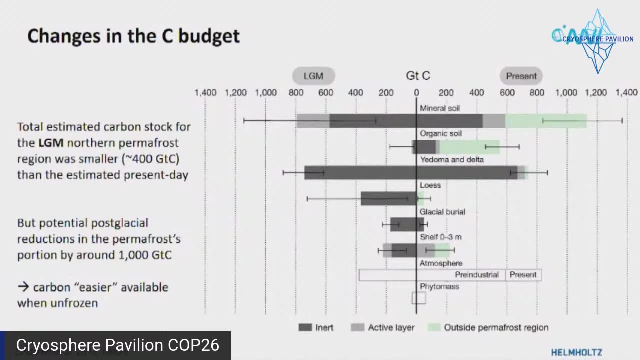 and this results in this, this graph here. so this was also done by Littren in 2018, published in nature. you see, on that side the last spatial maximum carbon budget and then this side the present carbon budget, so the total estimated carbon stock during the last glacial maximum. 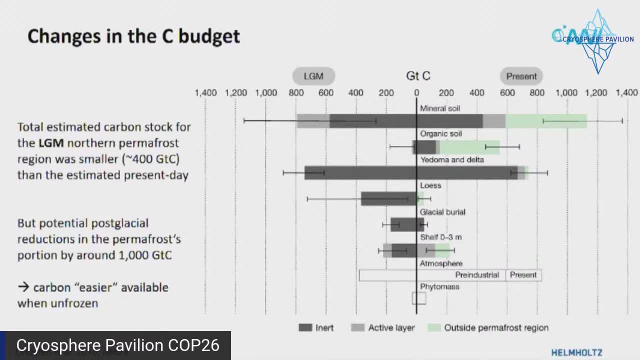 was a bit lower than today, but in the in the last glacial maximum, more of this carbon was frozen in, so not accessible for microbes. right, and today, um, we have around thousand gigatons of carbon not in permafrost anymore, so it's easier available when because it's unfrozen. so this is. 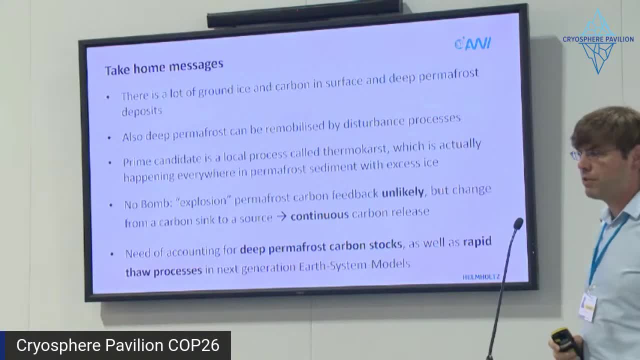 what we see here. my take-home messages for you are: there's a lot of carbon and a lot of ground ice in the permafrost region. this is even if the permafrost is deep- means not that it's not like being reached or reachable for uh thor, because there are processes like thermocost. 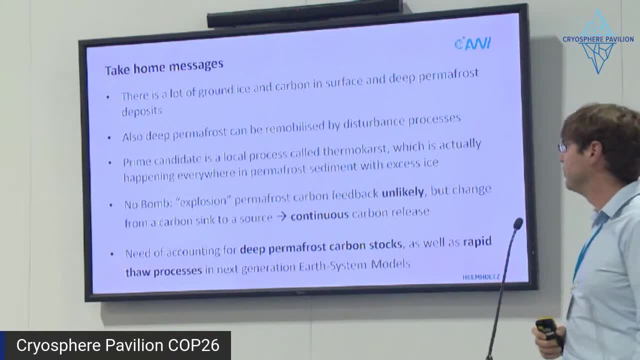 which have the opportunity to remobilize deep carbon. but there is no bomb, there is no explosion. um, with the permafrost carbon feedback, we don't have this explosion, but a change from a carbon thing to a source. but this happens continuous and not like an explosion. 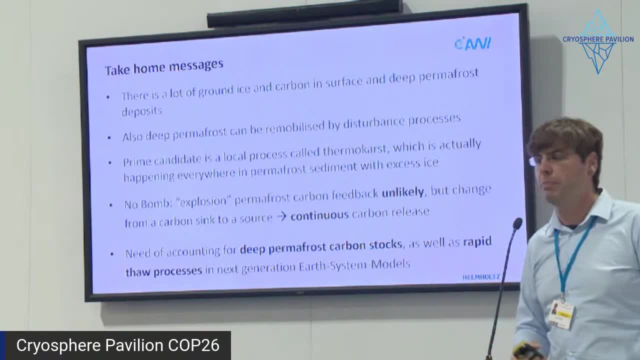 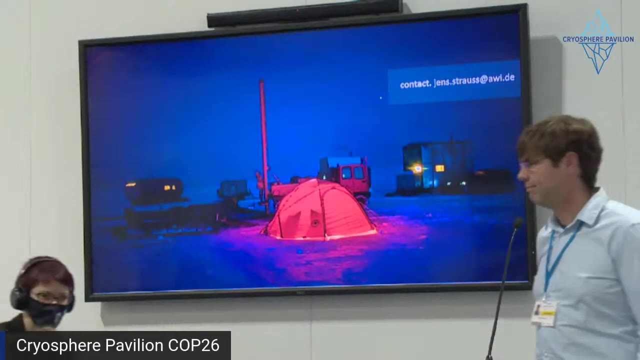 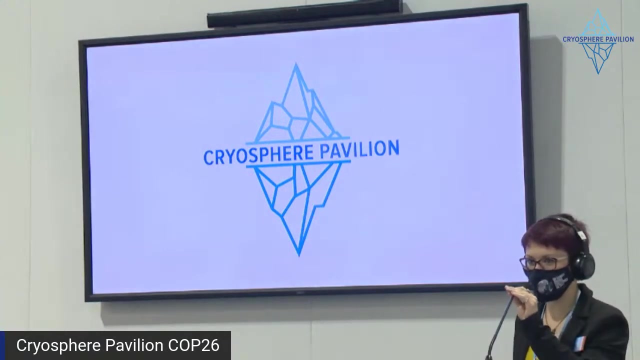 and we need for account the carbon pools of the permafrost region, as we had before, also the deep carbon pools in the next generation earth system models. thank you very much for your attention. thank you, this is another fantastic presentation and we'll now move on to our final speaker before. 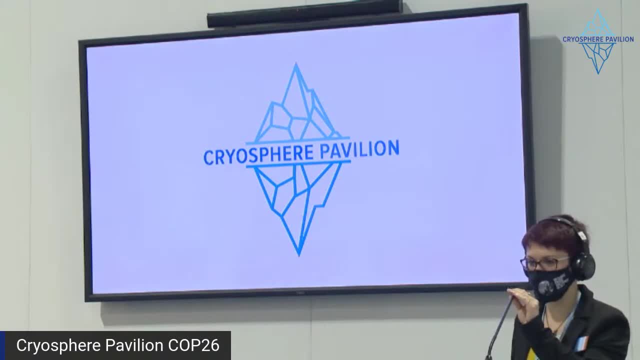 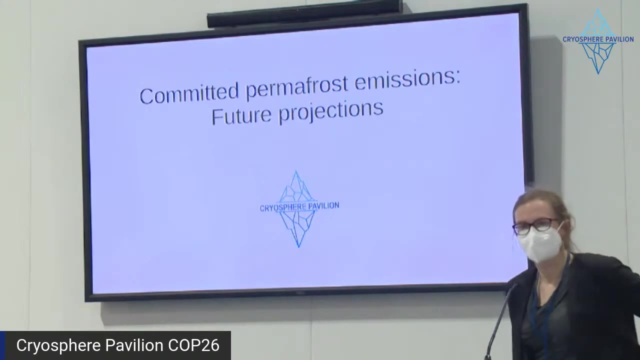 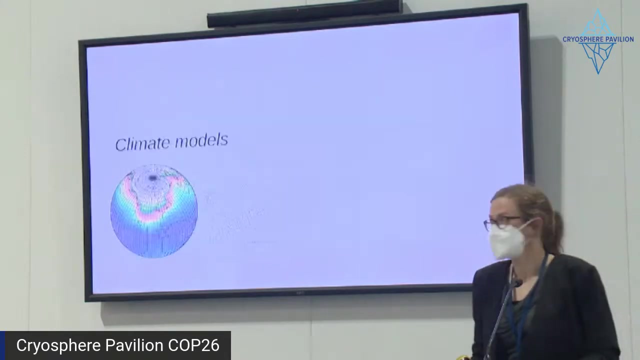 we move on to our panel discussion, which is sarah chadburn from the university of exeter. thank you, thanks, hi, everyone. so i'm going to be talking about future projections. so, oh, thanks, sorry about that. um, so when we think about future projections, we have to think about models. so 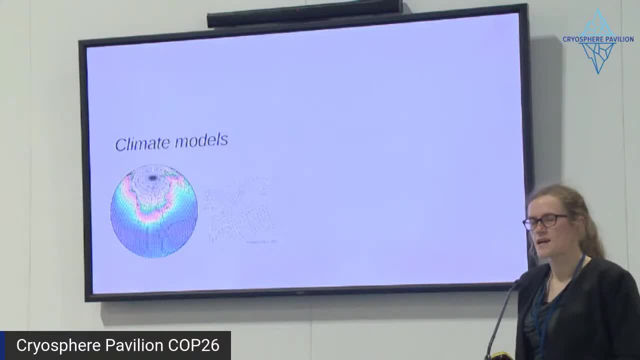 I guess all of us here would acknowledge the important role that climate models have played in warning us about the consequences of climate change, and models are used, for example, to give us our carbon budget, which is the amount of carbon that we can still emit to keep global. 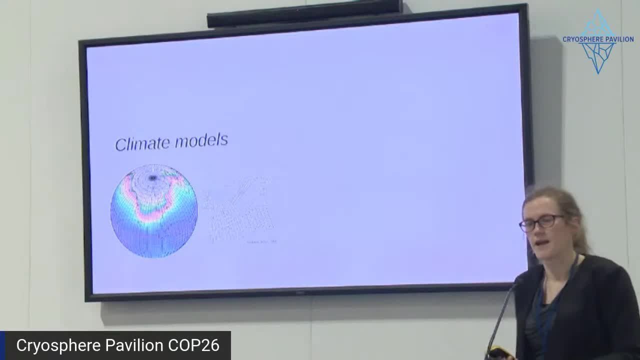 warming below a certain level and, as you know, it's not very much. now these models are. they represent work by thousands of people over tens of years, which comes together bringing all of their knowledge and expertise in to make this, this one model, which is essentially a computer simulation of the whole earth, which is an amazing human achievement. but, as you can, 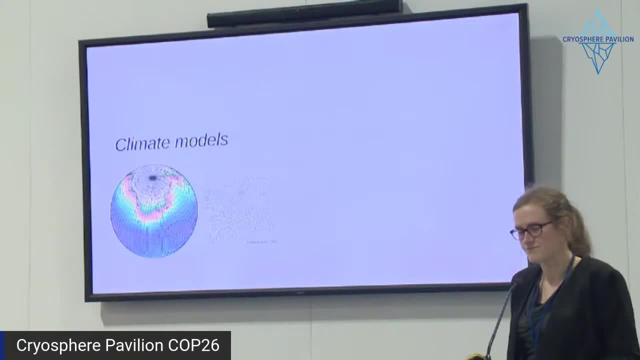 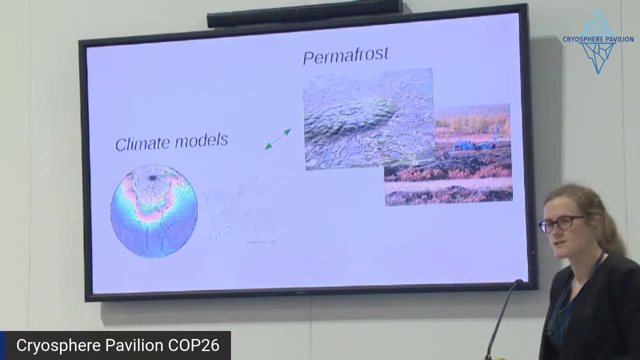 imagine. it's also incredibly challenging and difficult, and these models are used to help us understand the future of the earth. so climate models, in the end, can only be as good as our understanding of the earth that has gone into them. and permafrost you've just. 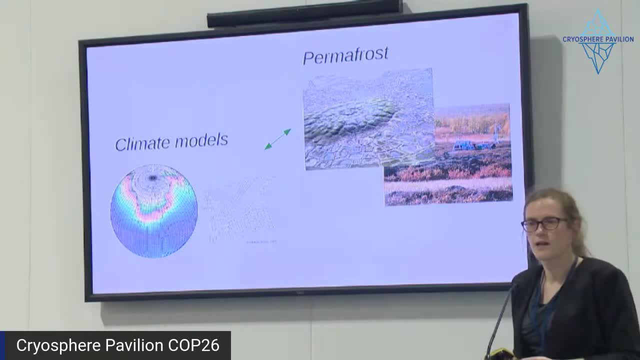 heard a lot about permafrost from my colleagues. permafrost is no exception to this, so if we want to look at the future of permafrost, then we need models. this is the best tool that we have, but this is also a challenge. so permafrost- 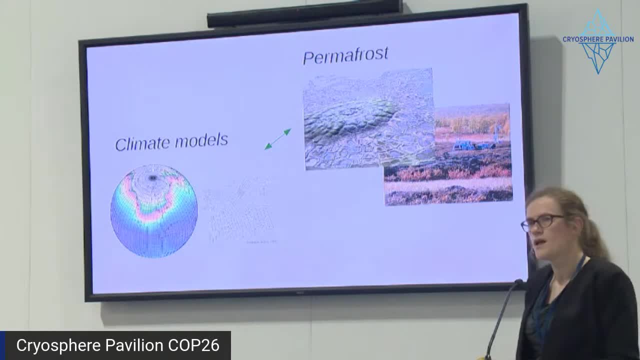 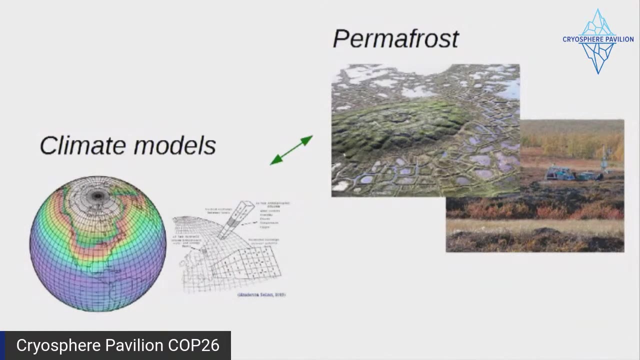 has. historically it's been difficult to measure and difficult to model, partly because of the complexity of the landscape there, as you can see illustrated quite nicely on that that picture. also because of the harsh environment in the Arctic which makes it difficult to actually get there and to measure the permafrost. so it's only actually very recently. 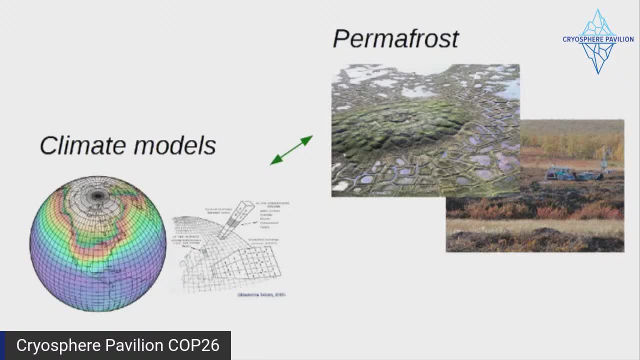 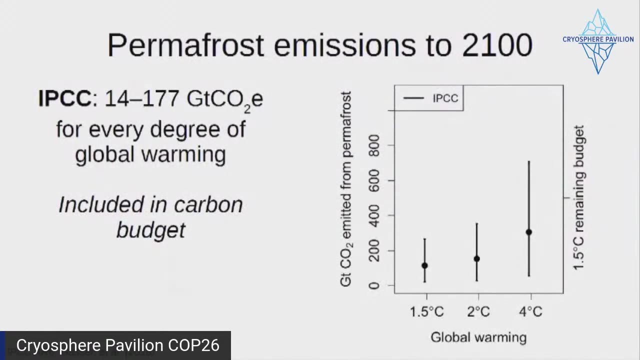 that we've really been able to include permafrost in these climate models and this latest IPCC report, which Gustav talked about. um, this is the first time that the permafrost carbon emissions have been included in the carbon budget. so the IPCC report estimates, uh, that between 14. 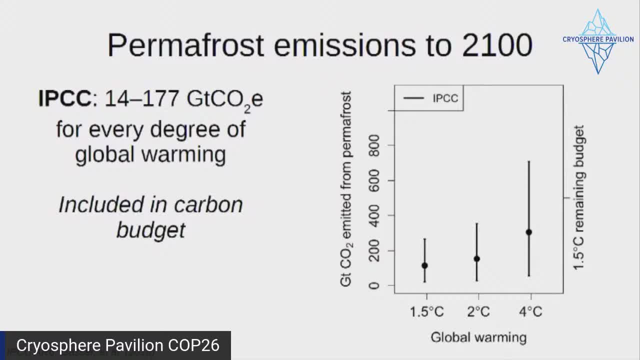 and 177 gigatons of carbon dioxide will be emitted from permafrost for every one degree um in which we warm up the plant planet. As I mentioned, this is included in the carbon budgets for the first time. Now. this plot shows basically this information, but then the amount of emissions for different. 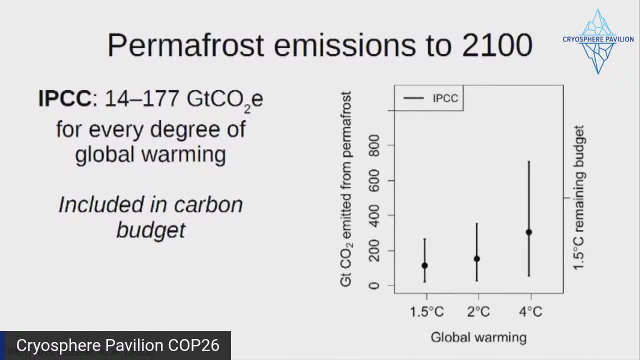 amounts of warming such as 1.5 degrees or 2 degrees. You can see the range there is huge. There's a lot of uncertainty there, but the one thing that the models all agree on is that the more warming we have, the more emissions we get from permafrost. Essentially, 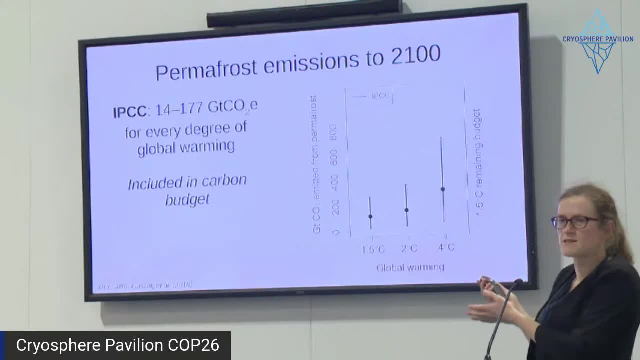 the more that we warm the earth, the more carbon will be emitted from permafrost, and that makes it even harder to keep the warming in check. Limiting warming is basically a double win if you consider permafrost. Now, the concerning thing is that there are 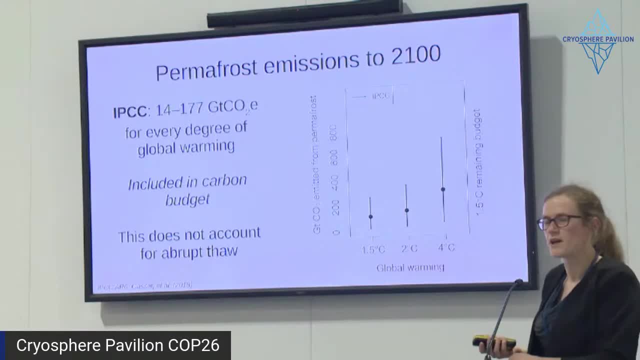 still some things that have not been included In this estimate and, as I mentioned, this is because it's difficult and we're only just starting to be able to quantify them. One of the things that has recently had the first estimate of how much might be emitted from this process is this abrupt thaw, which 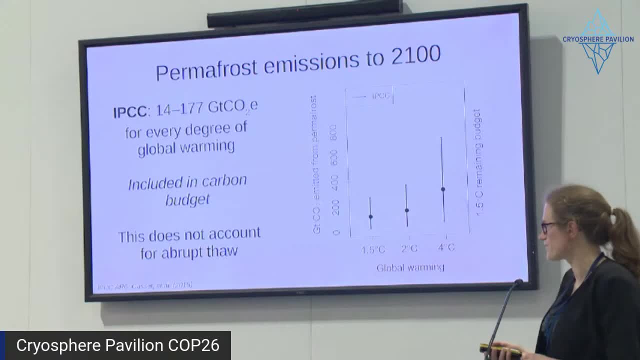 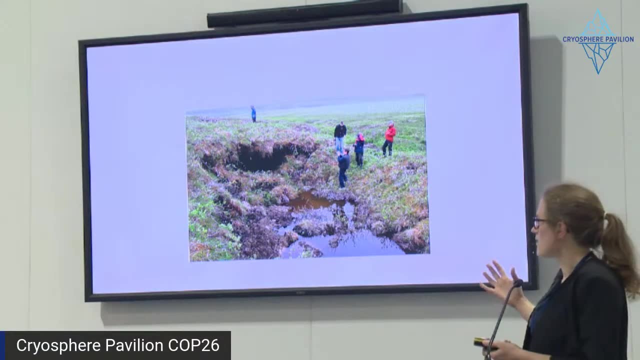 Jens has talked about in the previous talk. Abrupt thaw is difficult, both in the sense of measure and model, because it happens quite dramatically, quite quickly, but in very localized areas. It's difficult to predict exactly where and when it will happen. and 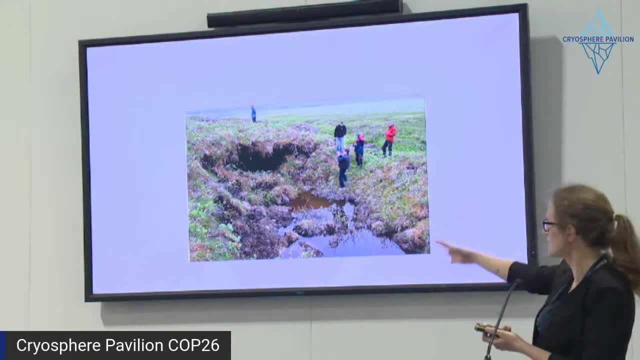 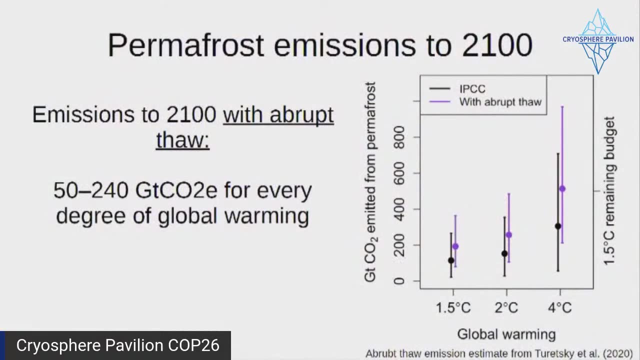 then what will happen to all of the carbon there? because obviously this is quite complex. what's going on there? The very first estimate that we have. the news isn't good. put it that way. What I've done here is, As a rough estimate, I've put the values from this paper by Turetsky et al I will give 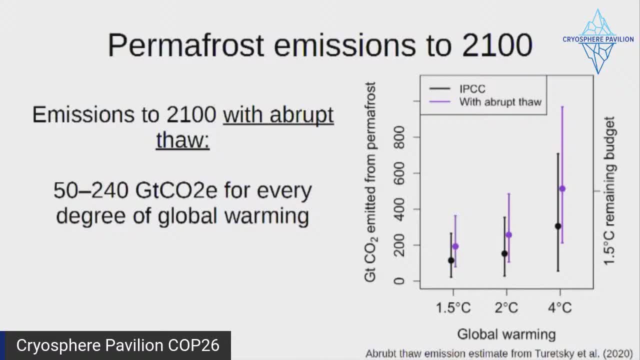 you all the references at the end. This was the graph I showed you before with the black lines, and then if you add on these emissions from abrupt thaw, then you get these purple lines. This is now between 50 to 240 gigatons of carbon dioxide equivalent. That's a lot. 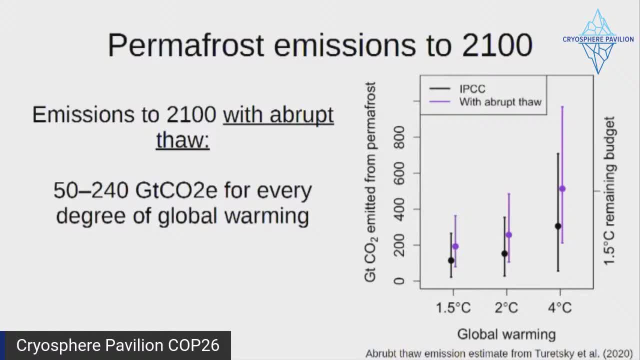 for every degree of global warming. It's increased it by around 50%. As I say, this is our initial, the first kind of study that has fully quantified this. I also wanted to point out that I'm saying it's gigatons of carbon dioxide equivalent. 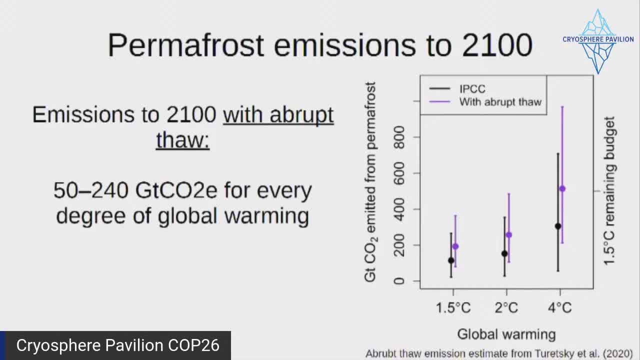 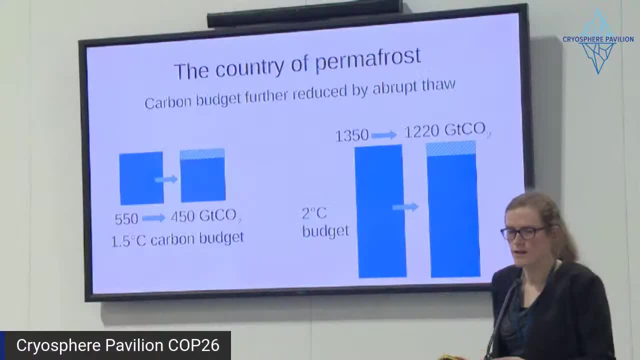 that's emitted, because a lot of the emissions that come from this process is in the form of methane. I wanted to show you what this means for the carbon. I'm going to show you the difference. Turetsky et al has a global warming of 50%. for every degree of global warming It's increased. 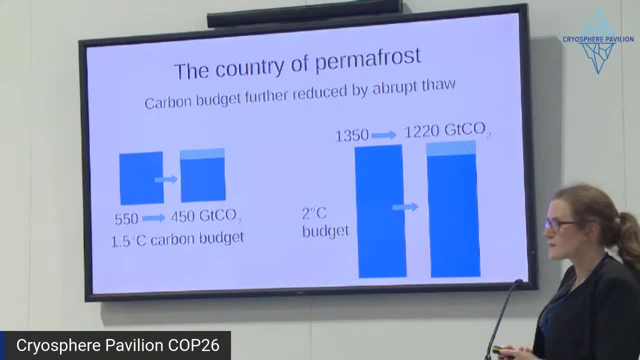 it by around 50%. As I say, this is our initial, like the first kind of study that has fully carbon budget. So, as I mentioned, a lot of the emissions that we predict from permafrost were included in this carbon budget for the first time. but this abrupt thaw estimate. 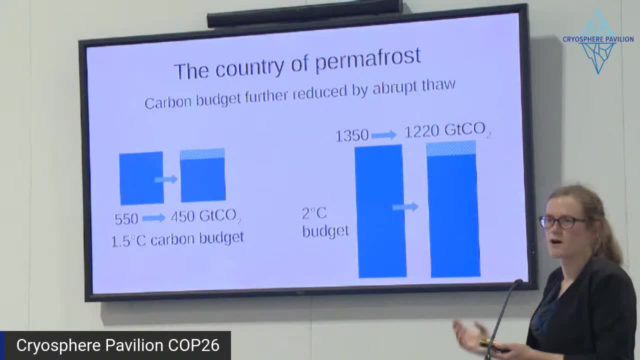 I've basically just taken that estimate off the carbon budget to show you what impact it has, and it's about a 10% to 20% reduction in the remaining budget. So a way you can think about permafrost is it's like another large economy which is emitting carbon to. 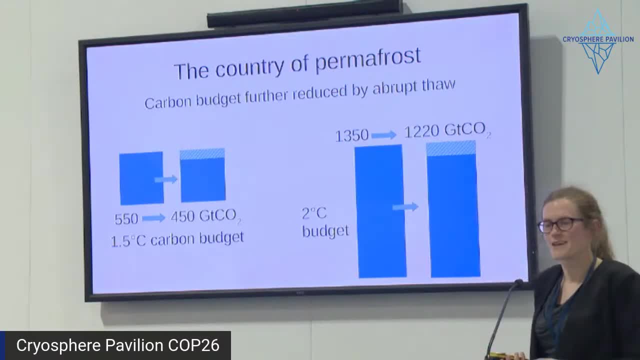 the atmosphere, like all of the other countries' major emitters in the world. But the difference is that permafrost hasn't signed the Paris Agreement and the country of permafrost has not got plans to reach net zero. So, essentially, this is bringing us on to the subject of our session, which is committed. 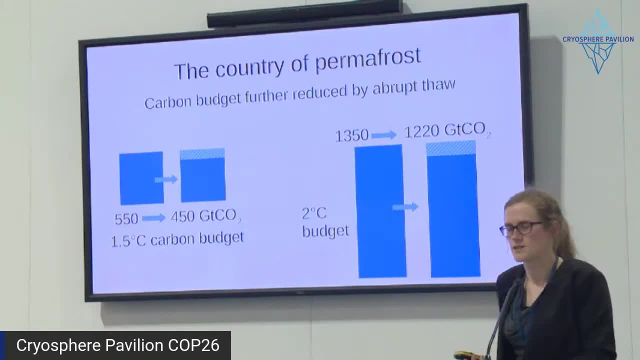 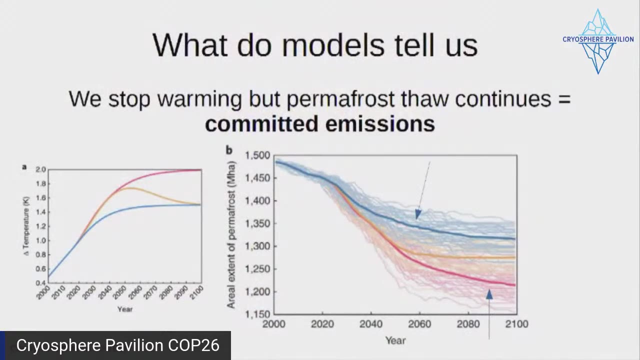 emissions in the long-term future and intergenerational justice. So permafrost will keep emitting carbon to some extent for a very long time. So I'm going to first of all just dig into why this happens, or what the models are showing. 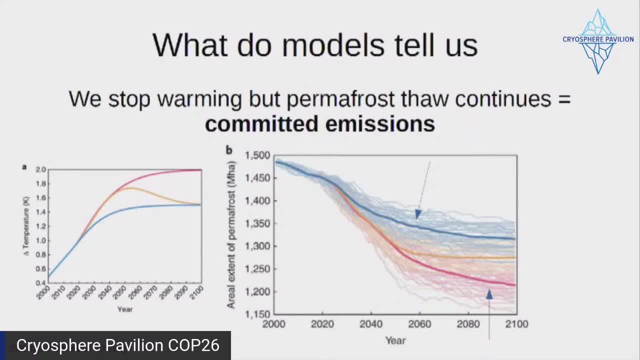 So what I'm showing here is a plot where you can see the amount of area of the land that is covered by permafrost. It's declining over time as we warm up the Earth and that corresponds to warming, which is shown on the left, And what I'm trying to indicate. 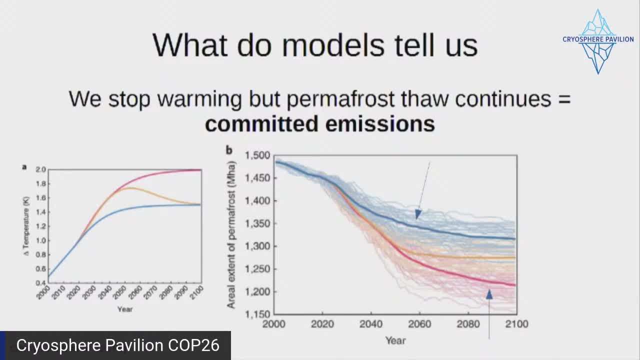 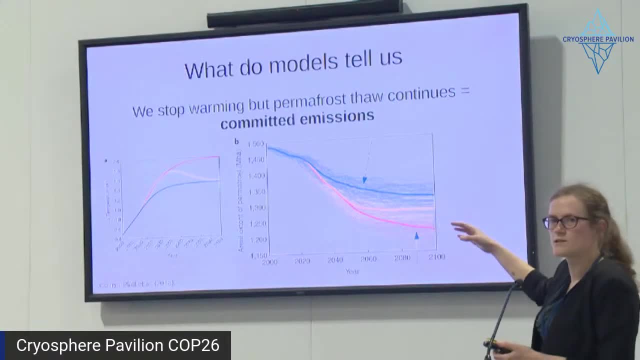 here is: I've got an arrow on the blue line and on the red line there showing approximately when the warming stops, But then you can see that the permafrost area continues to decline even for several decades afterwards. So essentially one of the reasons why we have committed. 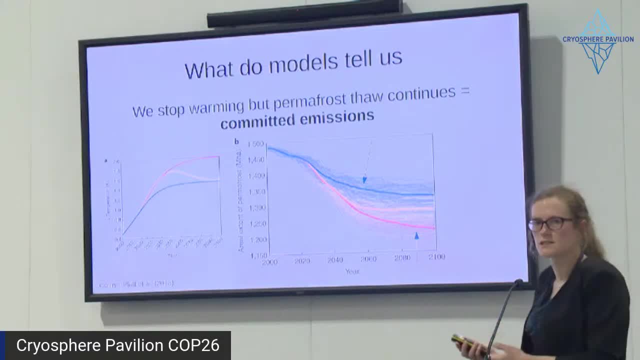 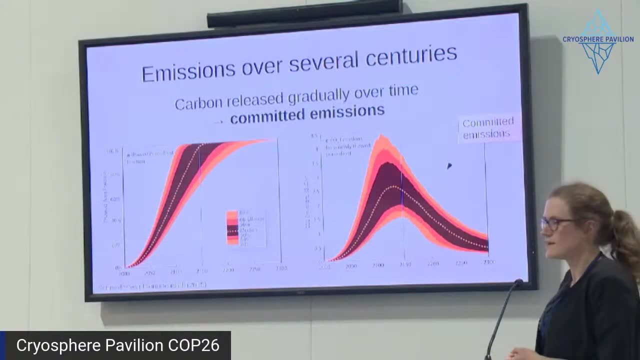 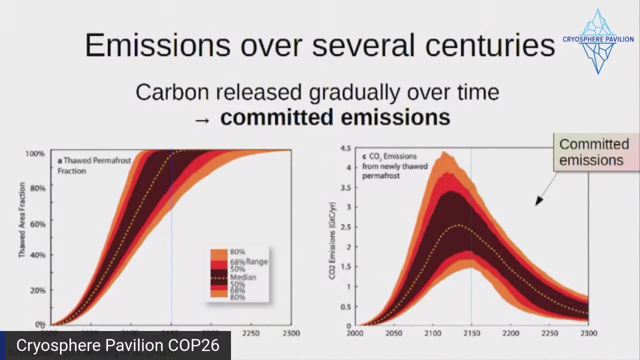 emissions from permafrost is when we stop the warming, the permafrost will still continue to thaw for some time afterwards. And then the other reason is that even once the permafrost has stopped thawing, the carbon will continue to be emitted, And what's going on here is that the organic 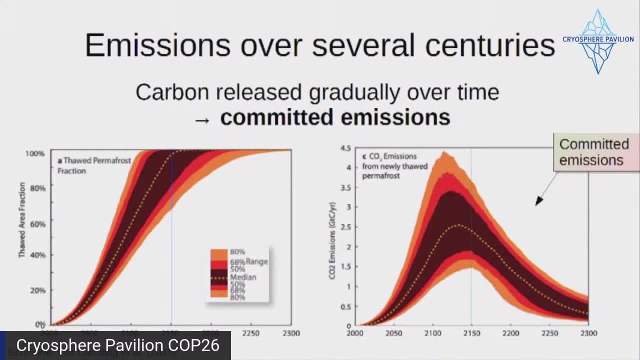 material in the soil gets gradually decomposed after it's been thawed And that means that the carbon is emitted from the permafrost gradually over time after thawing, And this is illustrated here. so on the left we've got a plot of how much permafrost has thawed. 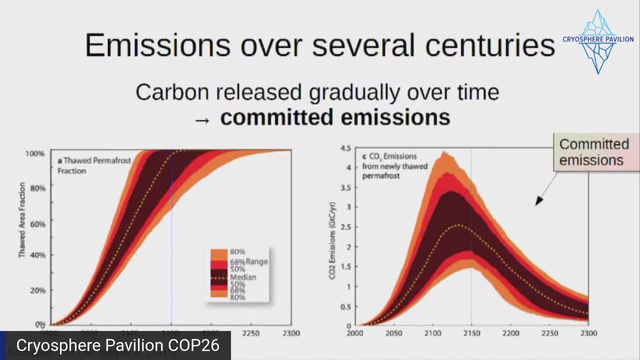 So at 2150, in this particular model all of the permafrost has thawed pretty much. But if we look here, this is the amount of carbon emissions we have each year and at this point the thaw is finished, but the carbon 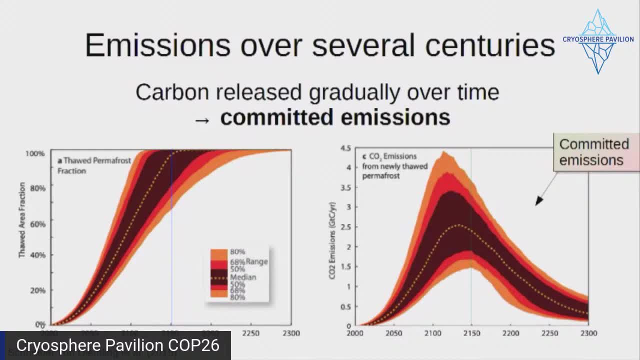 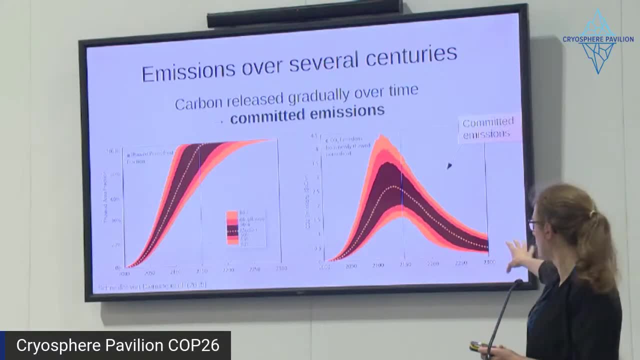 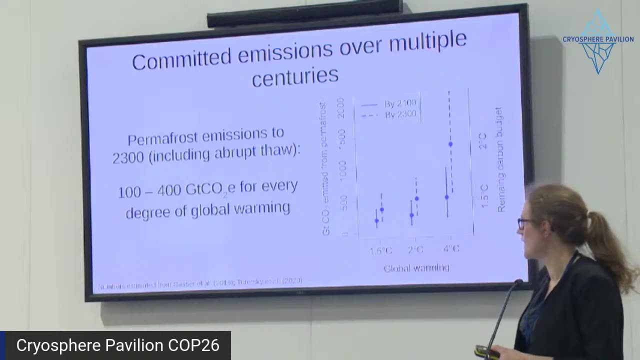 emissions are only declining very gradually over time, as the carbon is the vulnerable. carbon is sort of gradually used up and it's only reaching something that looks like net zero in several centuries time. so we have some very um again initial estimates of this, um which, again, i've 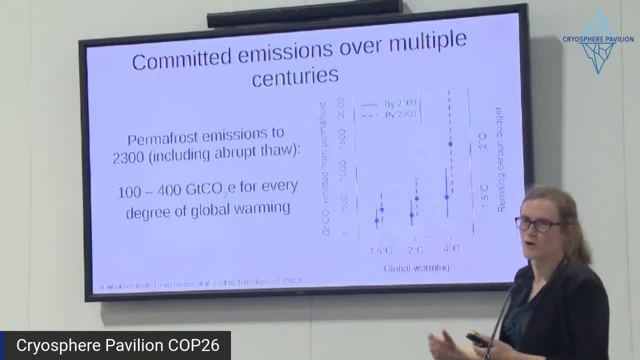 added on, uh to this plot. so i'm just increasing the scale of the y-axis every time, um, putting on these, these new emissions, um. so now, if we account for the really long term, how much carbon would be? we have roughly between 100 and 400 gigatons of carbon dioxide, equivalent for every degree. 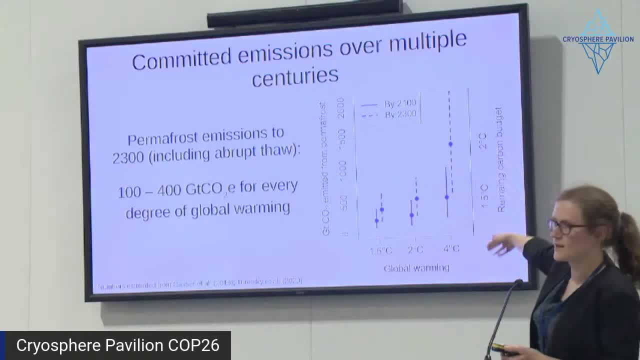 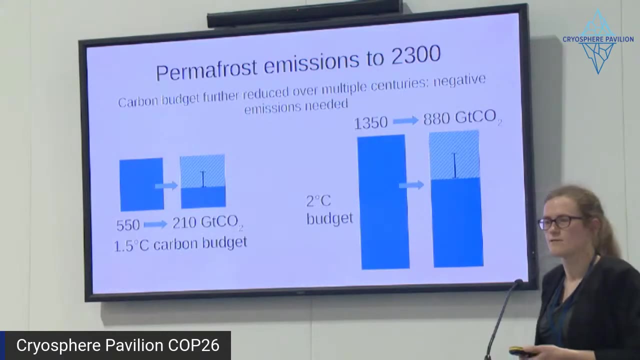 of warming and you can see. so these dashed lines are these these long-term emissions, and it's looking like roughly doubling the total amount of carbon that is emitted. so again we can look at what this means for the carbon budgets. so in this case, i've taken off what was already. 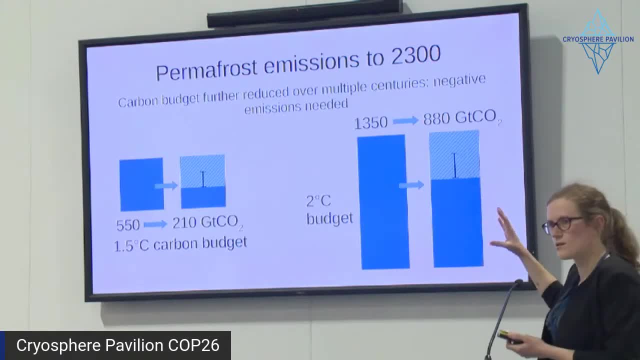 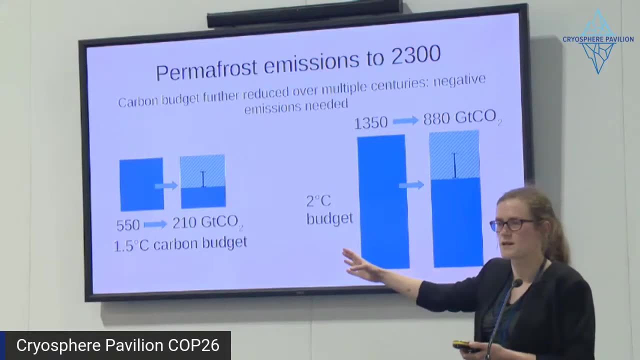 taken off for the abrupt tour on the other slide, plus these long-term emissions and you can see for the the budget that we have left for one one and a half degrees, which is obviously pretty small. this can use up actually more than 50 percent of the budget, so we can. 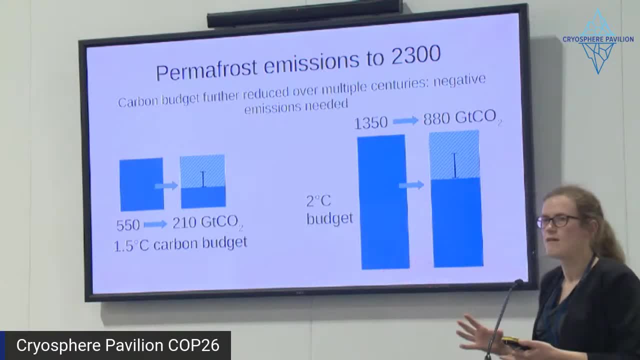 either think of that we have a very small budget left, or if we used up this whole budget this century, then we would be committing future generations to continued negative emissions. um, in order to keep the temperature uh stable or below the level of 1.5 degrees. 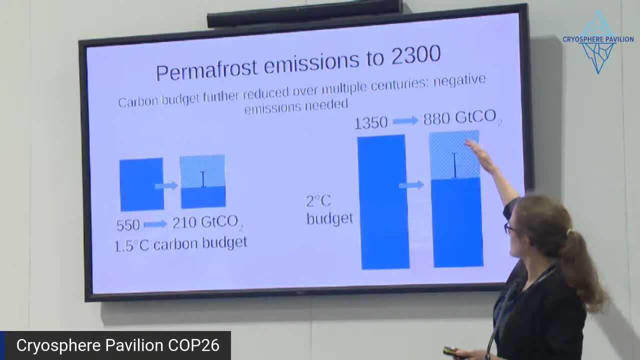 um, oh yeah, i was just going to show these, so the bits i've blocked out was sort of the maximum estimate, but these arrow bars are showing actually the range of uncertainty and what the estimate might be. so that's highlighting um the work that we still need to do scientifically. 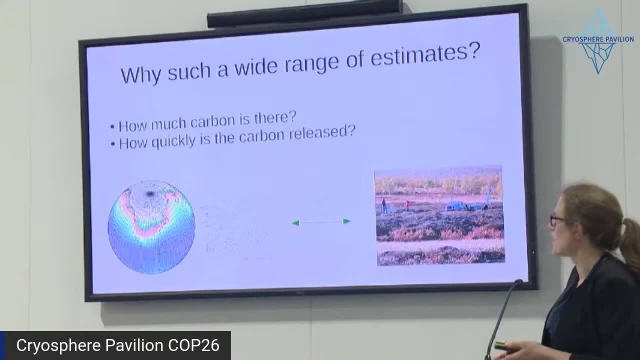 and the uncertainties that we have. so i just wanted to quickly point out some of the the major like areas of research and so one of the things that you you might expect that we might know how much carbon is in there. but actually this is really difficult to know because you can't see it from a satellite, because 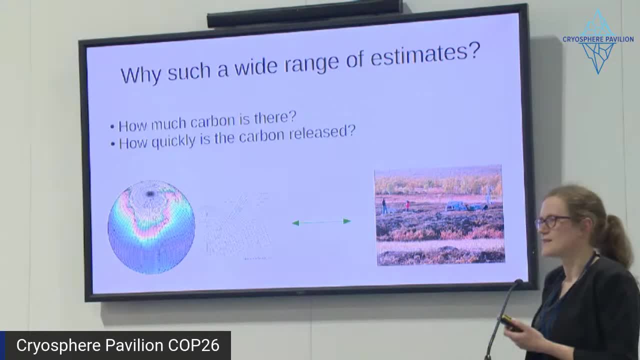 it's all below the ground. so, um, this is something that is still contributing to the uncertainties: how much carbon is actually there? we know it's a lot. And then something that is really uncertain is then, once you thaw carbon, how quickly it will be released. 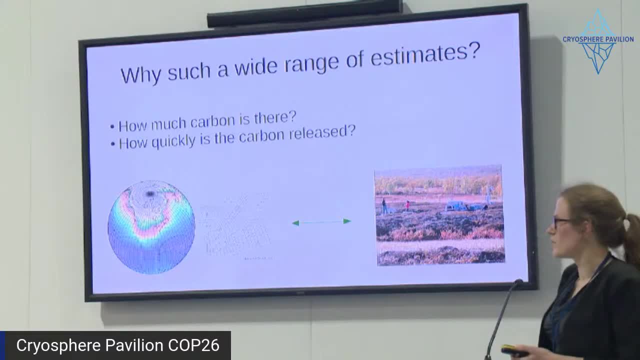 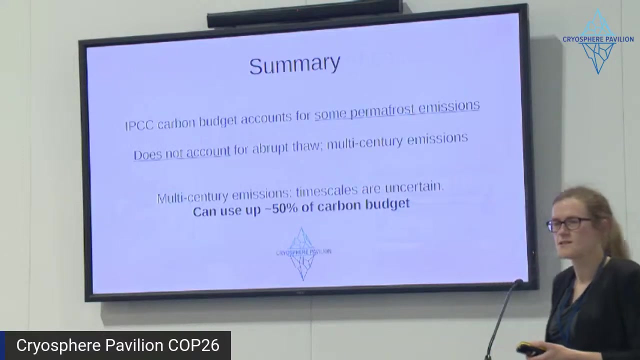 And so it's really important that we don't just run these models and say what does it say about permafrost, but that we continue studying the permafrost itself and asking: what does the permafrost tell us about our model? So, just to summarise, the IPCC most recent report has included permafrost emissions in the carbon budget for the first time. 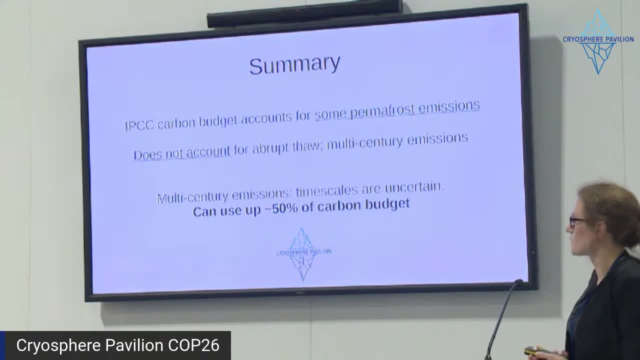 which is great progress, but there are missing processes, some of which we have not quantified at all and some of which we have initial estimates of how big these emissions might be, And that I've shown you today is the, the abrupt thaw processes and the longer-term emissions over multiple centuries. So, in summary, permafrost emissions will continue over multiple centuries and they can use up to 50% of our remaining carbon budget at the high end. And permafrost has no plans to reach net zero until at least a long time after the rest of us do. 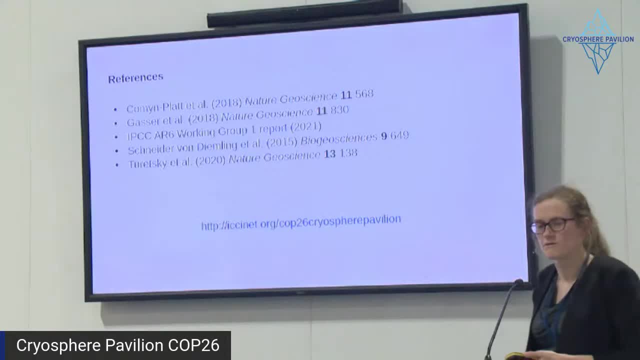 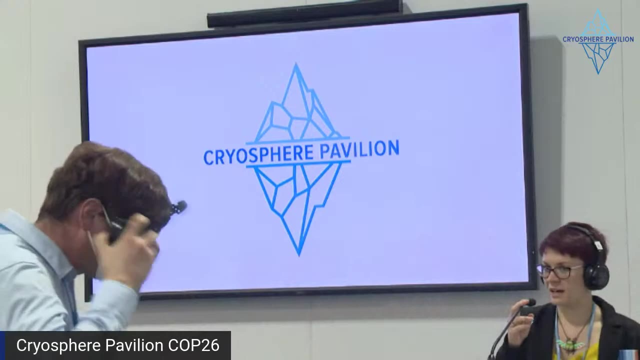 So there are the references and there's the link for all of the talks today. Amazing, Thank you all of you. And so we've talked there a lot about, obviously, the emissions from permafrost and particularly the sort of long-term implications of that. 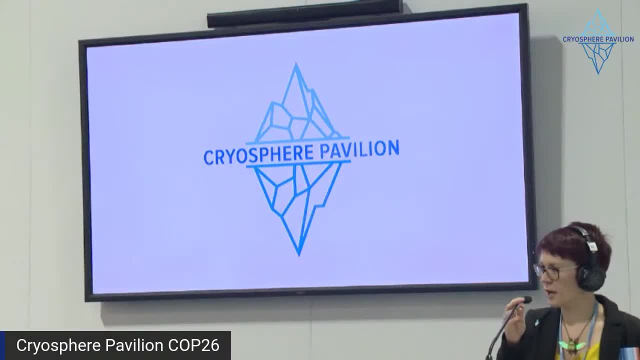 And so, to sort of delve into that a little bit more, we're now going to move on to a panel discussion, And I'm really honored to introduce our panel participants, who will be Darcy Peter, who's from the Woodward Climate Research Center. 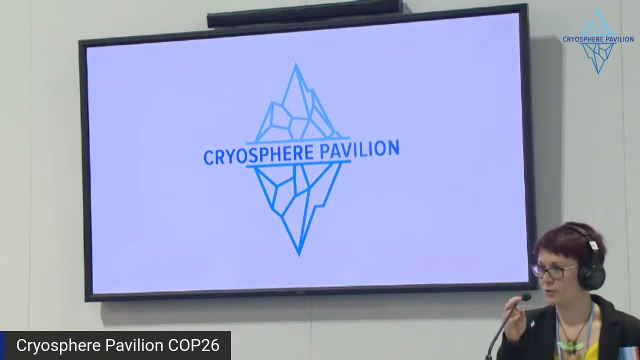 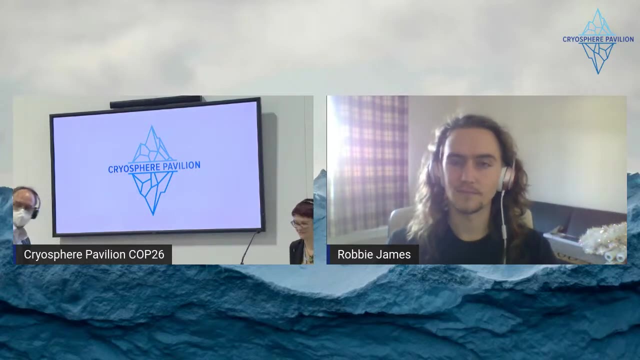 Ruth Miller from Native Movement and Robbie James from Green New Deal Rising, who'll be joining us remotely. So I think we're just bringing up setting up the panel and we will be with you in just a second, Thank you. Thank you so much, Michael. 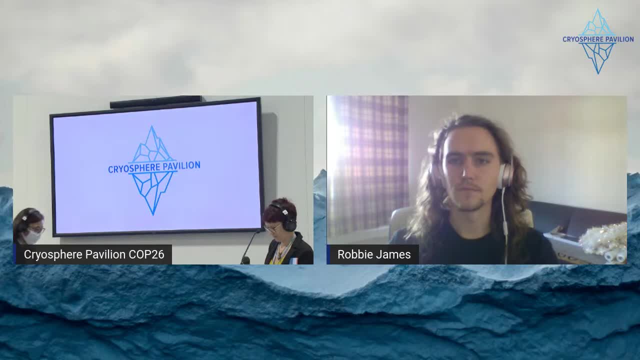 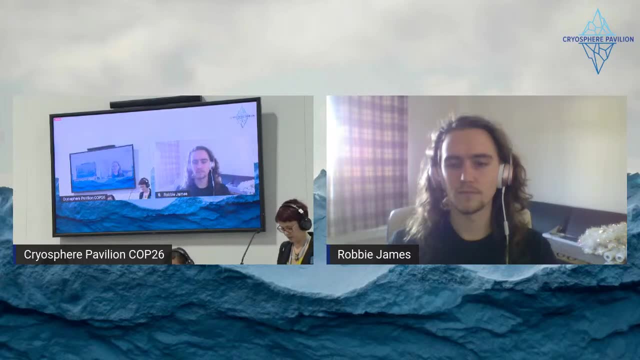 Great, I will be trying toừa you to head the chat logo there. If you could sponge that logo towards the mic, as much a feature of your station. Fantastic, Took me a couple days to check in to see how it looked. 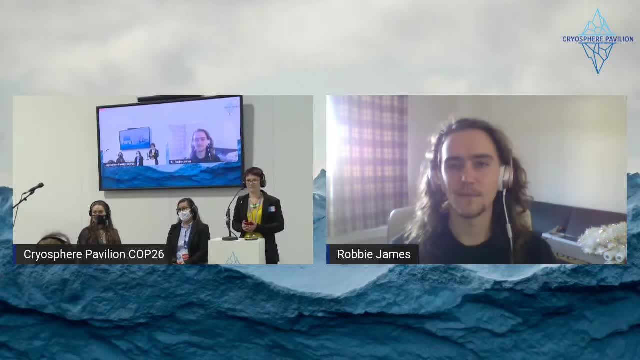 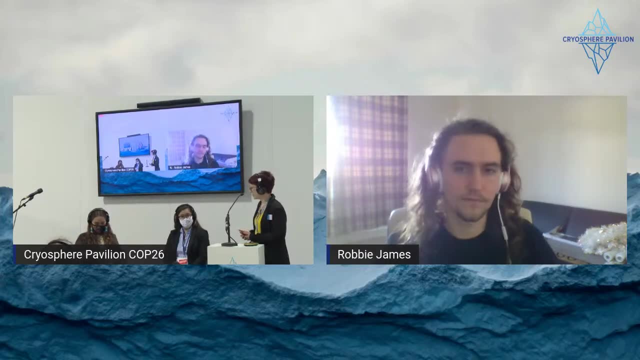 Great, Fantastic, Okay, so I think, to kick off, it would be great if just all three of you could just briefly introduce yourselves and tell us a little bit about where you're joining us from. So maybe it makes more sense if we start with you two here on the stage and then we'll move. 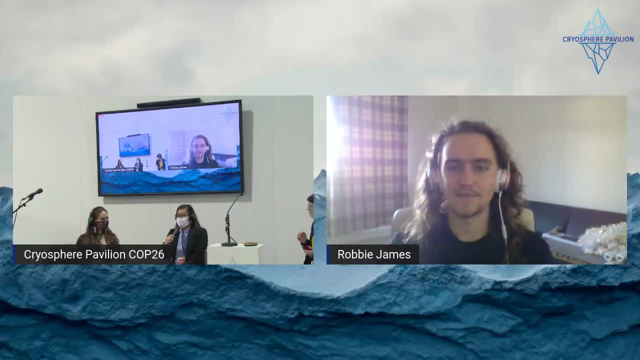 over to you, Robbie. I'm Koyukon and from the village of Beaver, Alaska, I'm an Arctic resident and I'm an indigenous youth and I'm a scientist at Woodwell Climate Research Center. 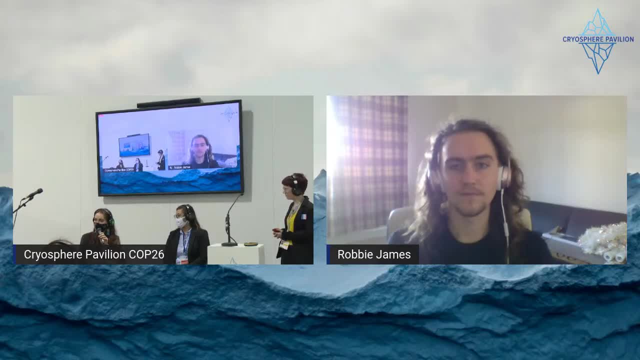 My English name is Ruth Miller. My Danang name is and I am Danang, of the Chiang tribe from the Lake Cork area. I grow up within my territory in Alaska. I serve as the climate justice director for an indigenous matriarchal advocacy nonprofit. 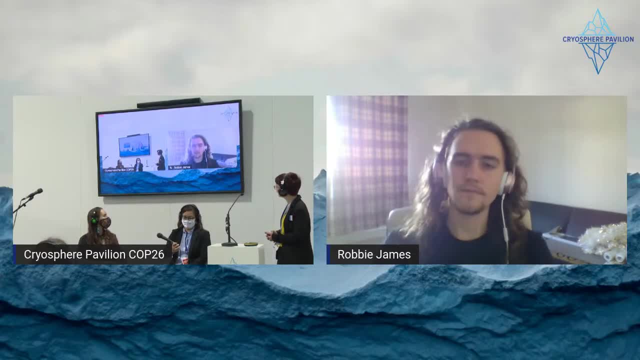 called Native Movement. Hello, can you hear me? okay, yeah, awesome. so hello everyone. my name is robbie. um, i'm sort of new uh to activism, to climate activism. i've done that through the green new deal rising uh leadership program and i'm i'm also studying a master's of biology at swansea university. 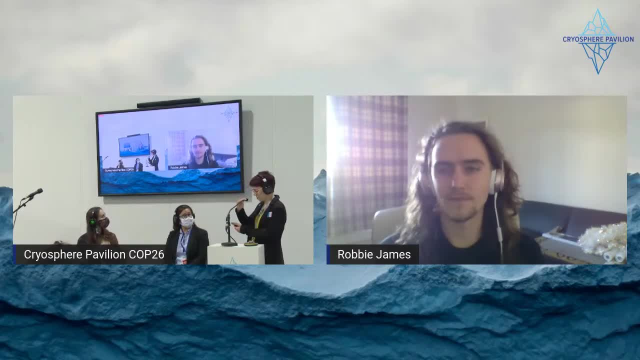 thank you, um. and so first off i'd like to kick off um, if it's okay, um, with a question to uh, to both darcy and ruth. so obviously in the, in the talks we've just heard, we've talked a lot about um, the fact that permafrost and the arctic cryosphere broadly kind of responds to 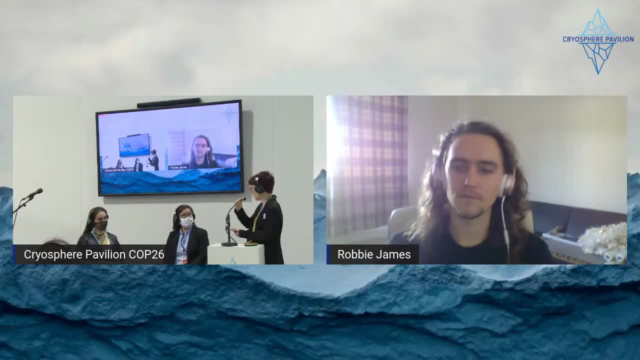 warming over very long time scales, um, and, of course, at the same time, we're seeing impacts happening in the arctic today. so i was just wondering if you could um share your thoughts with us about sort of your responses to the talks and what this means to you as arctic residents. 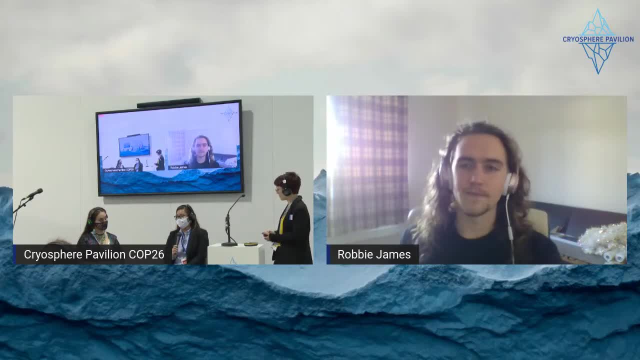 yeah, so, uh, in my experience in beaver alaska- it's located about 100 miles north of fairbanks alaska and about four miles below the arctic circle- um, the permafrost slot changes that we're seeing are hugely detrimental to food uh, security and 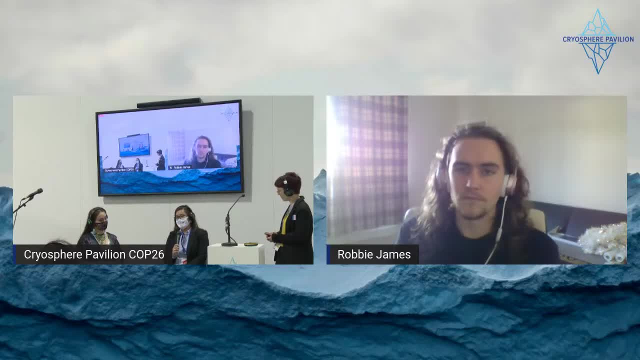 it's causing severe food insecurity. um, yeah, the river banks are eroding. um, houses are falling into the river. um, salmon can't find their spawning grounds. salmon account for 34 of all protein along the yukon river. um, and so yeah, and on top of that, uh, there's the challenge of policy and regulations. 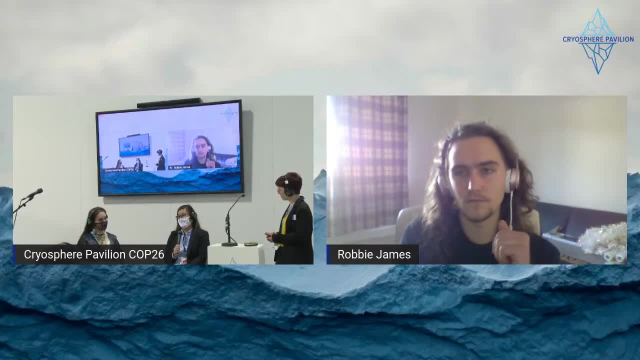 this year was the first year that my village was not able to fish for salmon at all, um, for the first time in at least my parents and i's lifetime. so there are many contributing factors. permafrost definitely is not helping, at least in my family's experience. 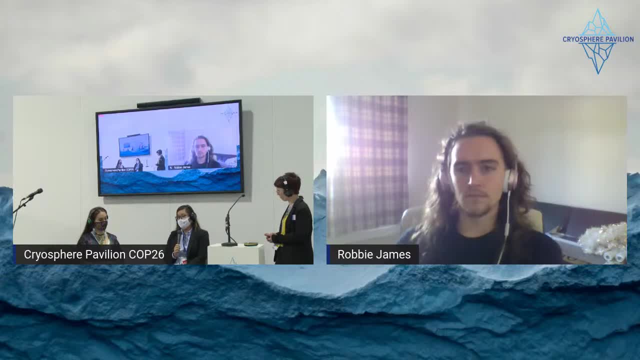 it's causing huge food insecurity and therefore adding pressures to harvest different animals that also have different policy struggles. so food insecurity is probably the biggest one for my generation and for future generations. yeah, our indigenous communities are incredibly adept at adaptation. we have lived with by and for our lands and waters for tens of thousands of years. however, when our 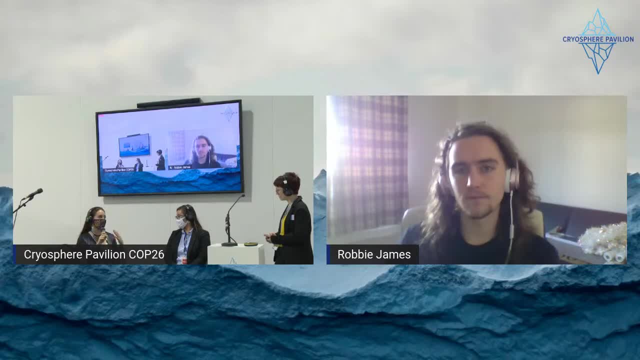 ecosystems are changing at such a rapid pace. i mean, we in the area that darcy just described. my mother grew up there and there are new lakes that i can visit that didn't exist when she was a child. um, that's a cultural thing. um, you were talking about tross�agissae now, compared to my, 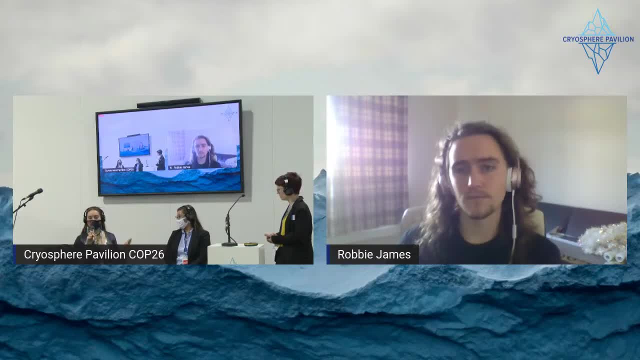 many of them in fact. And of course, we know that the methane being released by thawing permafrost is a threat amplifier. It is a feedback loop that will only accelerate the rate of further thawing. But from an Indigenous perspective, though we are adept at adaptation, we also understand that we 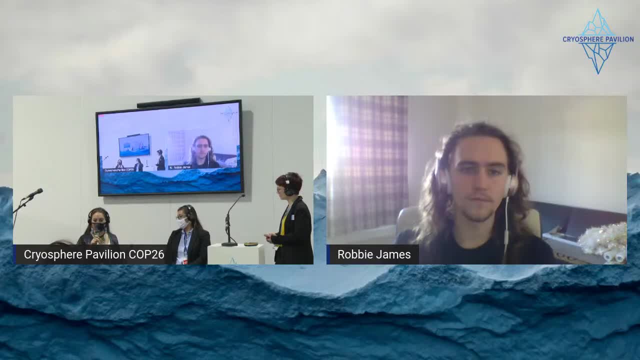 are at a precipice, a global moment of decision-making that we will never be able to come back from. We heard in the last presentations that once that, despite you know, immediate climate action, which, as I'm sure we all know here at the UNFCCC, is debatable whether or not. 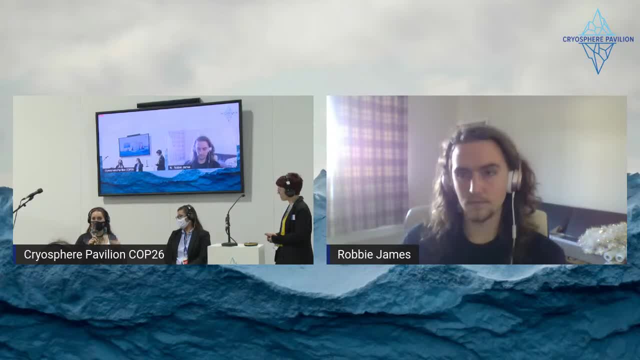 that will happen, even with climate action. now, we will still experience the impacts of continually thawing permafrost that we cannot recover from, And so we are not only being asked to deal with the lived impacts on our food security, on our cultures. 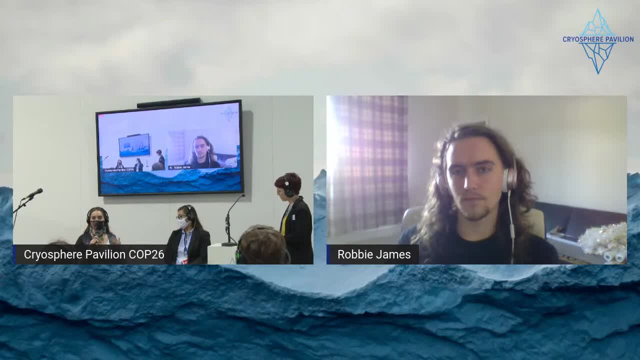 and to adapt quickly to lands that are becoming quickly inhospitable to us. but we are also, you know, the harbingers of what is coming, because we are tasked with the responsibility of not only suffering first and worst, but also relaying that to spaces such as this and describing the ways. 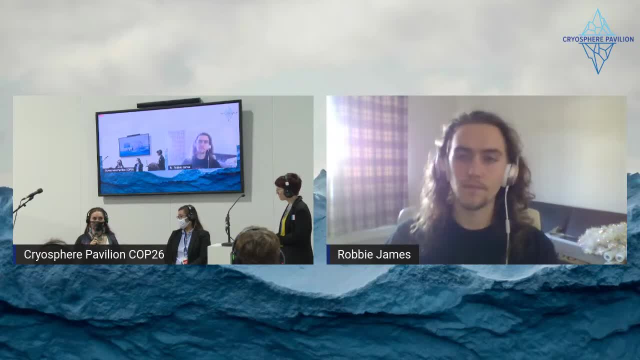 that our lived experiences are being impacted today, And so it's not only a matter of you know. so the question was: you know what is the impact of melting permafrost? Well, we're going to continue having these impacts for hundreds of years. that will only get worse. 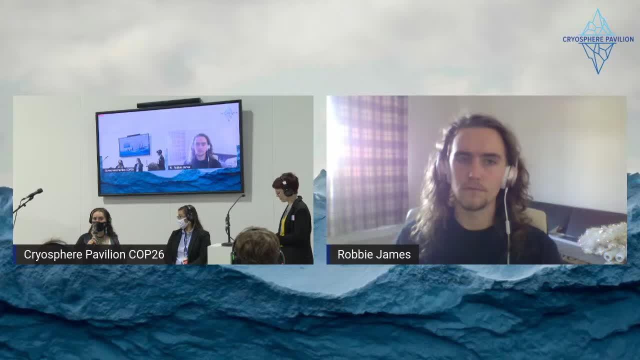 So to me it's also there's a relationship with fear that this threat is ever present, that we cannot recover from. We can only try to not make it worse. So much it's really powerful, And so I'd like to sort of open the floor to Robbie and ask so. 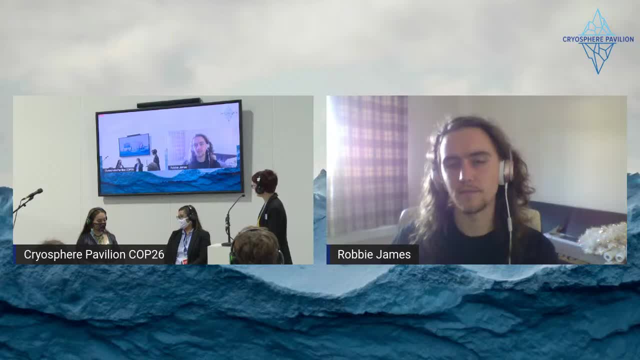 obviously you're participating in COP as a youth activist with a UK Green New Deal rising, a UK-based organization, And we all sort of know that young people around the world have really been kind of spearheading a lot of the discussion about climate change and climate action over the last few years, And so I wanted to ask you about sort. 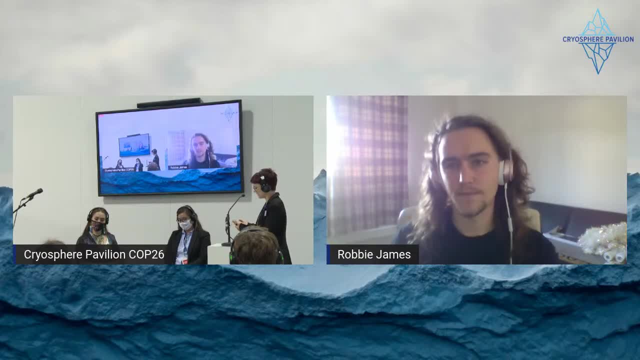 of. given that, do you feel like the impacts that climate change has on younger generations and on future generations in the context of the issues we've discussed today? do you feel like those are being taken more seriously as a result? Do you feel like they're being taken more seriously as? 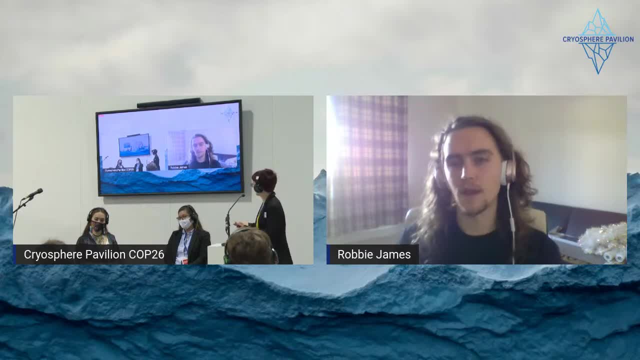 a result? Do you feel like they're being taken more seriously as a result? Do you feel like they're being taken seriously enough? Yeah, just your thoughts on that. Yeah, so I think to different extents, from different groups. I think overall the conversation. 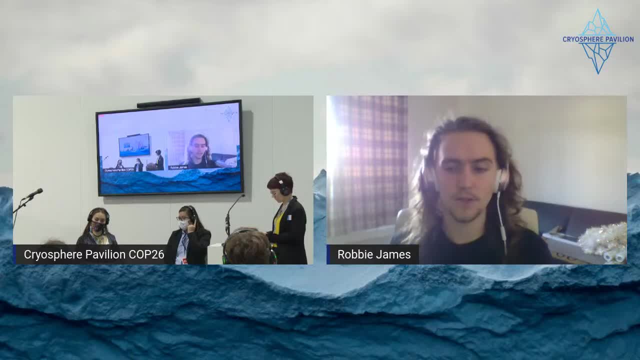 is getting better. I think Greta did a great job at putting youth into the center of the movement. I mean, at the end of the day, youth are the biggest victims, so it makes the most sense that they're the ones who have the loudest voices as well, or whoever are the biggest victims. 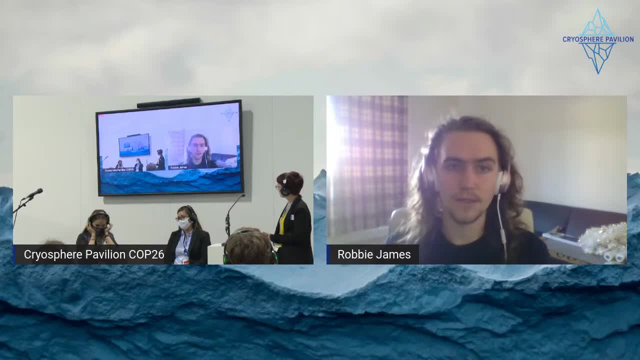 So that includes indigenous communities and multinary communities in areas sensitive to climate change in developing countries as well. So yeah, but however, I think a lot of – I think the further up you go, the more hypocrisy there is. So I think like, especially in the UK, our government. 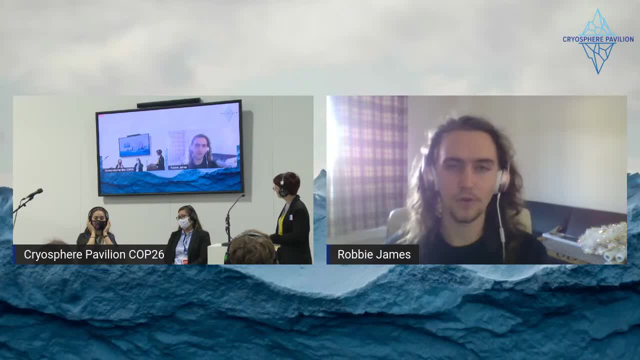 their words and their actions don't really seem to match up. so therefore, the answer would be no from them, because it doesn't – you can see it. talk all you want. You can speak in foreign languages. speak the language up And, hopefully, like we have, along with our therapy, doing yes, do need to. 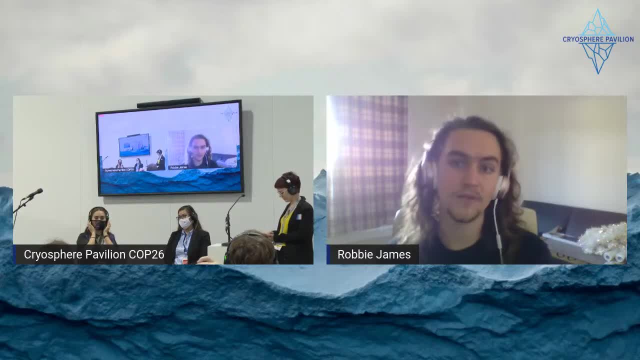 of course, actually partner with them or lack lots of roles for them to work and help them out at, seems want you can say that you give these features, but if you're approving, uh, oil and gas fields and things like that, then you really you're really not um, but i am thankful to see that overall. 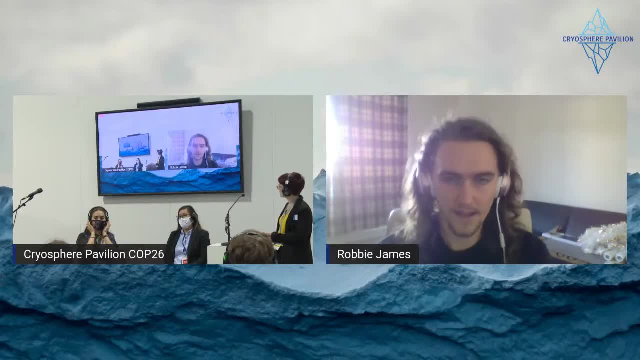 i think in the sort of wider, wider sphere, it is, uh, getting better, but we just need the people in power to take that really seriously. ravi, it's, it's actually great to meet you, um, and i'm i'm sorry, i know this question wasn't for me, but um, it also just brought to mind. i also serve as the 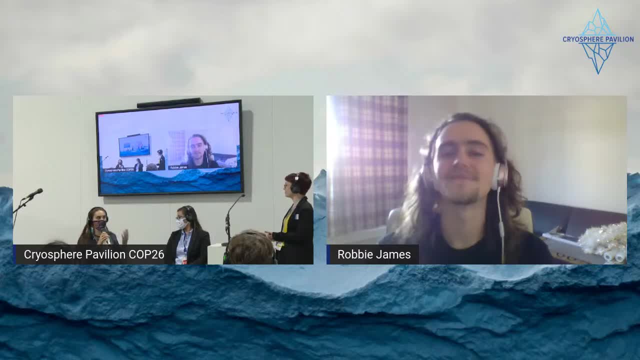 alaska state lead for the national green new deal network in the us and facilitate a lot of the both policy and narrative pushes on behalf of national green new deal priorities and from an indigenous community's perspective. after after the first few months of our work, we started getting 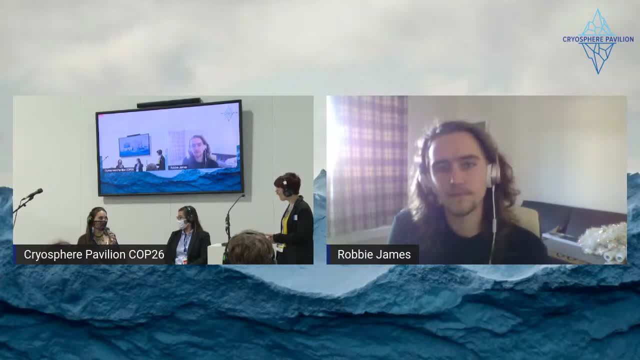 you know, so much appreciations and gratitude from the national network leading the infrastructure and the transportation bill, those that have been following, i'm sure just as tired as i am, um, especially around narrative work, the way that we were describing and educating national green new deal policies and translating them to an alaska perspective, the reason that we were so adept at. 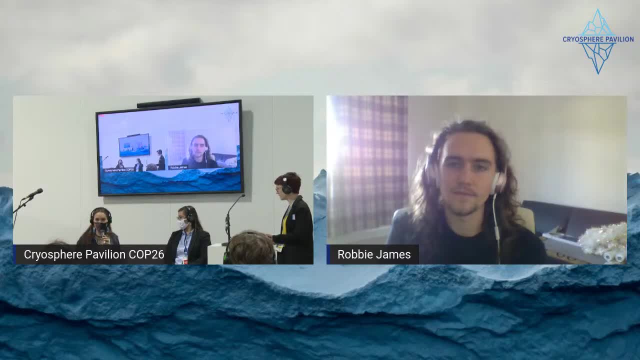 that is because it is indigenous values of justice and reciprocity that underline just policies, and so when we received this work, we knew that we would never want to or be able to sell it to the our communities. that is not our way of being or our theory of change, so we did the translation work. 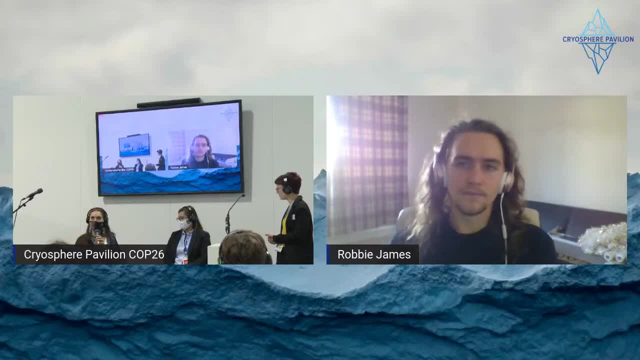 of um finding the values framework within our indigenous cultures and making the green new deal conform to that. so we have done this as well with the framework of just transition and also work very hard to do this not just with green new deal policy and just transition, but also with climate. 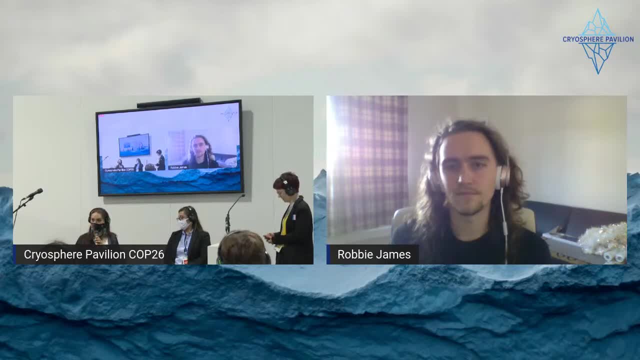 science to make it relevant to our, for instance, our oral histories and our traditions of story telling. uh, to think about the ways that we can integrate climate science into culture camps when we're out fishing on our rivers, or or moose camp when we're out hunting. um, and from a green new. 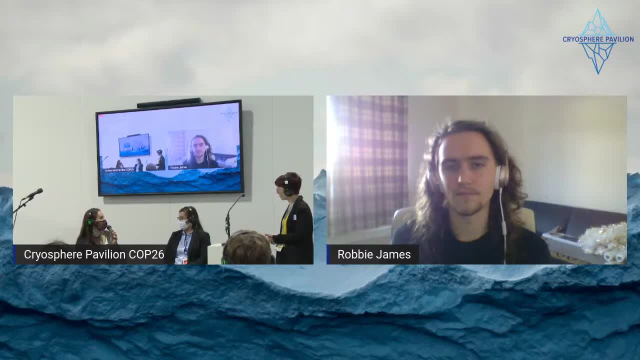 deal network. you know specific framework, just because i'm i'm so happy that you're participating, robbie. um, that is, the only way to make policy and climate science relevant to indigenous communities is not to start from there and bring it in, but to begin with our indigenous communities and think. 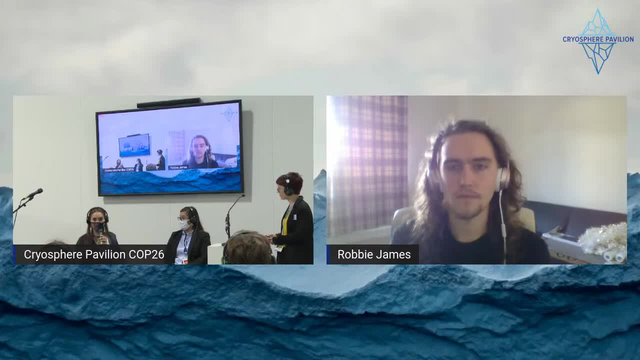 about what indigenous values being integrated into green new deal policy and climate science can look like fascinating. thank you, ruth. um, and i guess, slightly building on that um, could you speak a little bit to why it is so important that indigenous youth in particular are really included and welcomed into these spaces, uh, like here in carp, and i'd be really interested as well to. 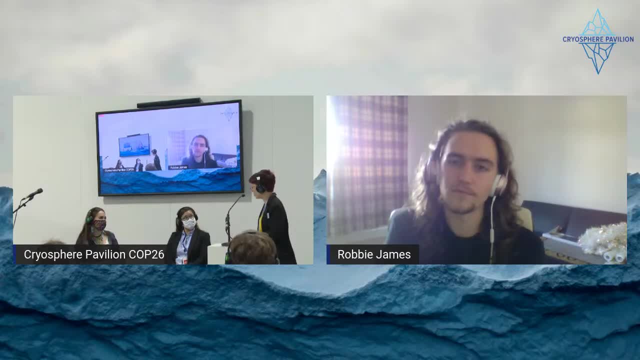 hear both of your thoughts on how effectively that's been done at this cop and perhaps what we could do better. darcy handed the mic to me because she knows this is my thing and i'm just going to say it's my favorite thing to rant about. um cop 25 in madrid was my first cop. 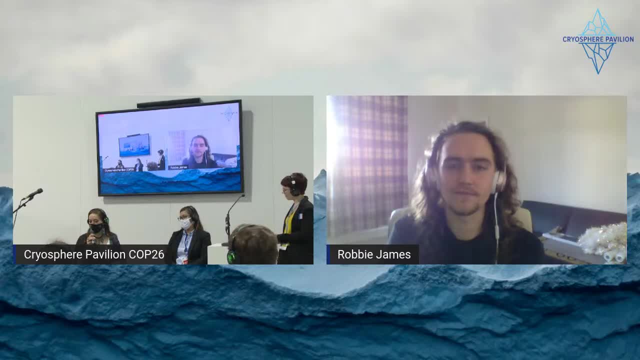 um, there are a number of folks here in the audience who who accompanied me there as well, and, um, by the time we left, we left so deeply exhausted and traumatized that we wondered if, if we would be able to responsibly bring youth here again, because it is such a toxic and colonial. 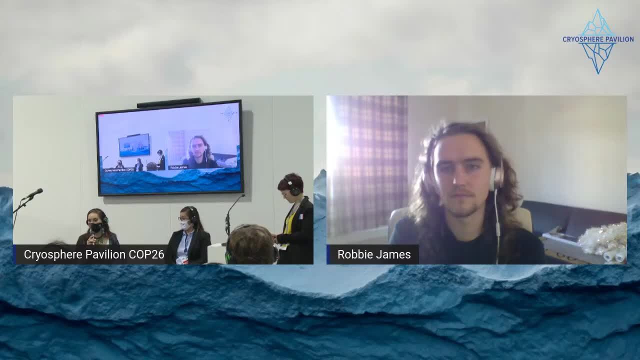 environment that praise. it extracts from us and, and if we are given a platform, it is often tokenistic. so any of any youth inclusion- particularly global south youth inclusion and indigenous youth inclusion- that is achieved here at the cop is is on our backs. it is because of our labor and our resilience to make our own voices heard, to pave pathways for us, and 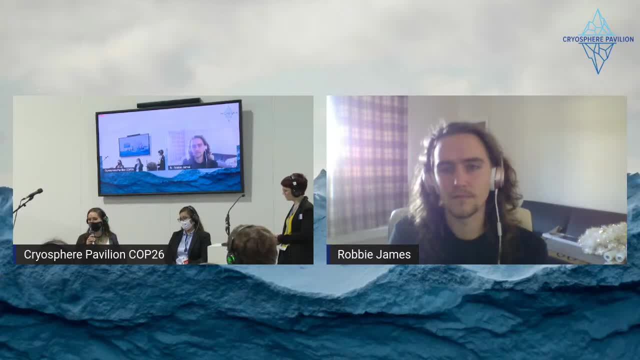 to code switch to be here speaking proper english, to take our, our cultures, our traditions, our languages, knowledges from our elders and and translate it to the country where we live. you are here in a way that others who are so far from our cultures might understand This COP in particular. 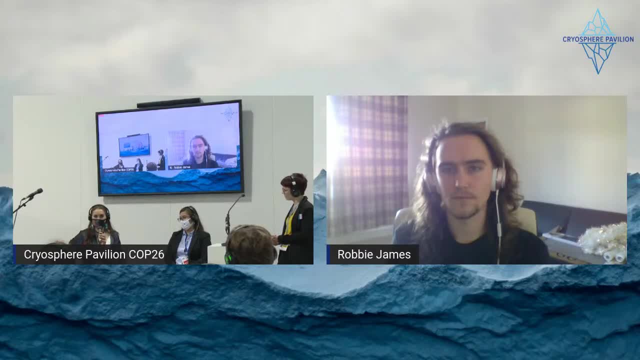 is being elevated as the most inclusive and diverse COP, and I could not communicate enough that there's nothing farther from the truth, which has been widely addressed already, even in our first few days here. There is a huge disparity in access to this COP, particularly from the 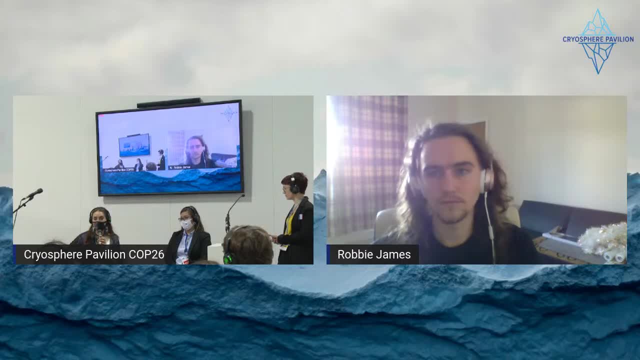 Global South and those who have not been able to access vaccines, particularly those who have not been able to access broadband, even through virtual offerings. But additionally, there are very, very few frameworks for which Indigenous peoples can arrive here, and there's very little. 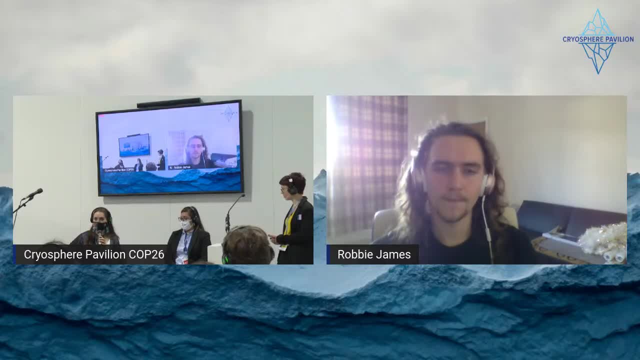 funding. So myself as Climate Justice Director of a non-profit, we fundraised to bring youth here. It took about $15,000 to bring three Indigenous youth, including myself, here. Last year when we brought 11 Indigenous youth, it took about $100,000. And that burden 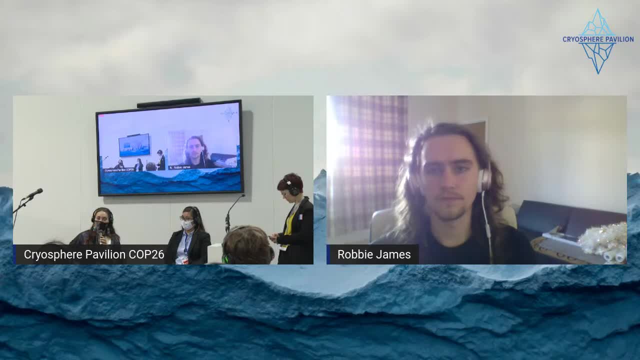 was on us to fundraise alone, And now that we are here, many of our options are to do media stunts, which is important, but there is very few invitations to join high-level negotiations for any youth. but even through, for instance, Yungo, the youth constituency group, which 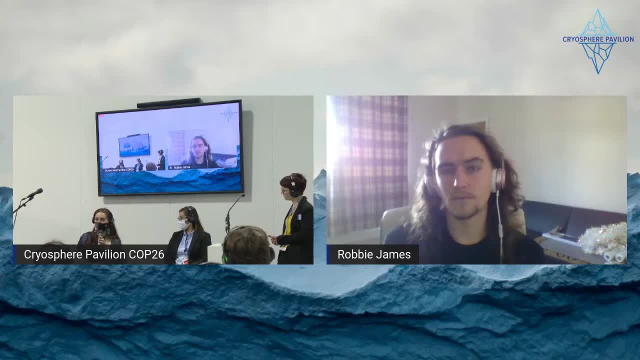 I also participate in. the options are few and far between, And I'll just add that I was honored and pleased to be part of the Yungo Foundation and I'm very happy to be part of it. I was also part of both the Youth for Climate Pre-Cop Summit hosted by the government of Italy. 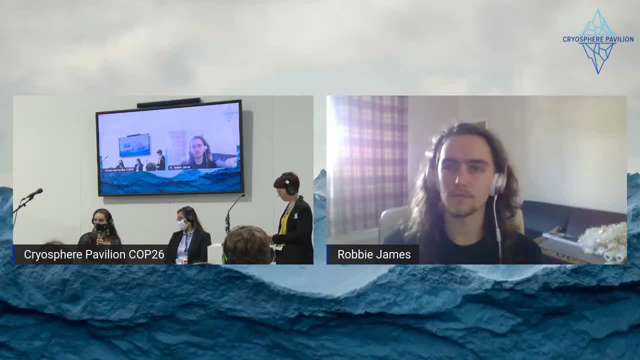 last month, as well as the UN Conference of Youth, COI 16,, hosted by the Yungo constituency just before this COP, which are, you know, the formal pathways for youth to be involved. At the first, at Y4C, I was the only Indigenous person from all of North America, no Indigenous people from. 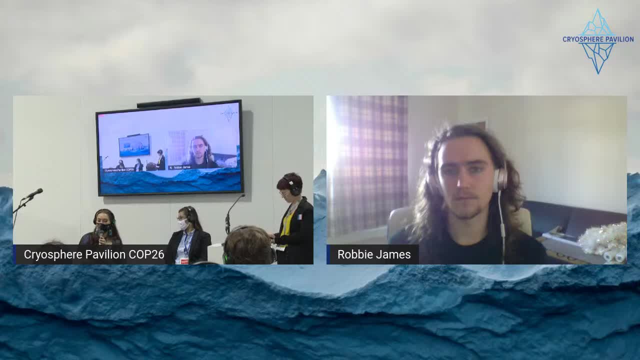 the Pacific or Asia. There was one other Indigenous youth from Brazil, two of us there alone At COI 16, again, I was the only one from North America And I can tell you this is nothing to brag about. It is profoundly lonely and desperately heartbreaking. So if we want to, 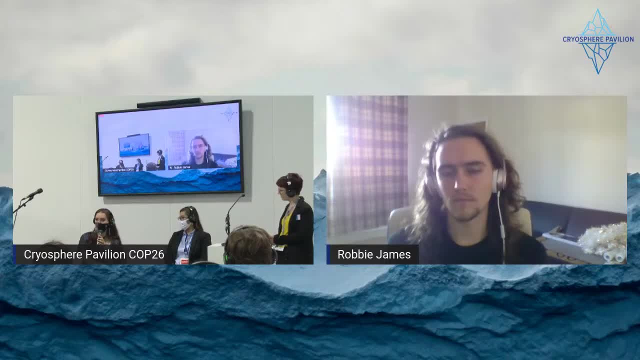 look towards actual engagement with UNFCCC processes. it's not enough to give us the option of fighting our way in here. We must be deeply integrated into all levels of decision making and policy writing, as our Indigenous governance structures teach us. I don't know how to follow that. Oh man, I'm so happy I gave you the mic first. 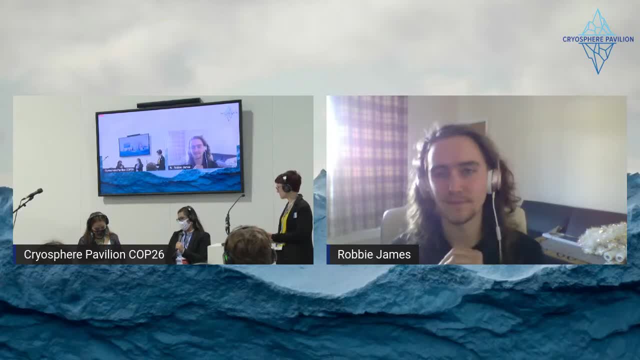 Yeah, so obviously there's a huge disparity with age and gender and race in terms of the science community. It's no different in the policy community. I'm really honored to share the stage with you and share the stage with Robbie. Yeah, no, it's, it's amazing, But I 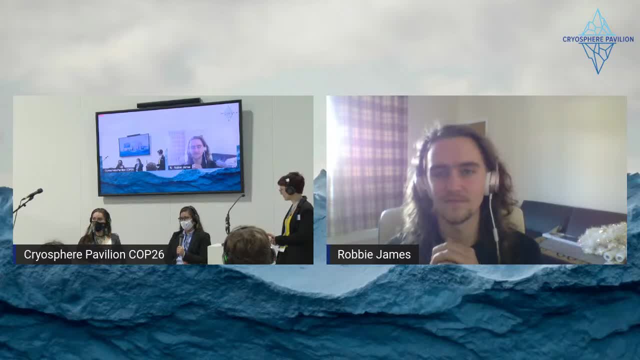 also deeply realize. you know, coming from a village of 30 people, it's very small, it's very tight knit. It's a completely subsistent way of life. There's no grocery store where I'm from. Not everybody has the privilege of going to college like I did. 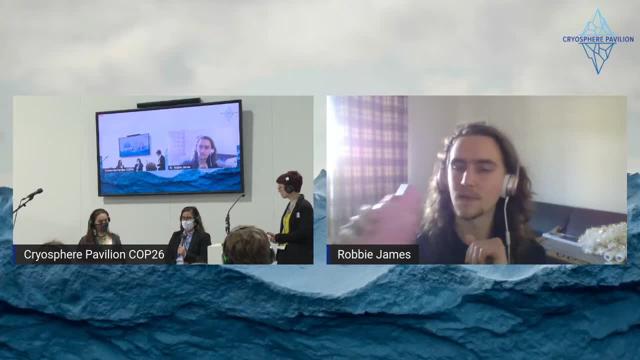 or of coming here like I do, And I recognize my privilege And I'm just deeply humbled to be here And it's, it is very overwhelming, I can't say that enough. Um, COP 25 was also my first COP. I I didn't even see Ruth. 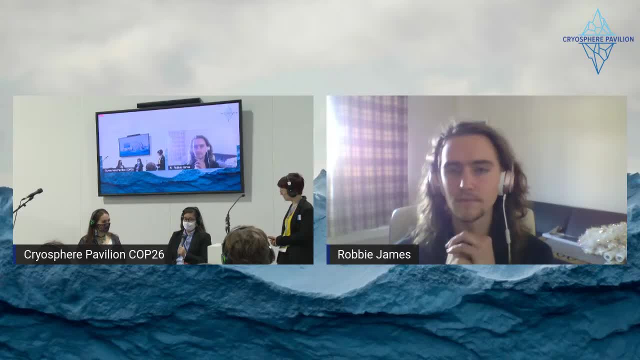 when I was there, Yeah, like it was insanely isolating. This is a completely uncomfortable space for me. I understand the privilege I have to sit here and have these conversations and tell you my way of life and my people's way of life, But I also understand that it's not just me here. 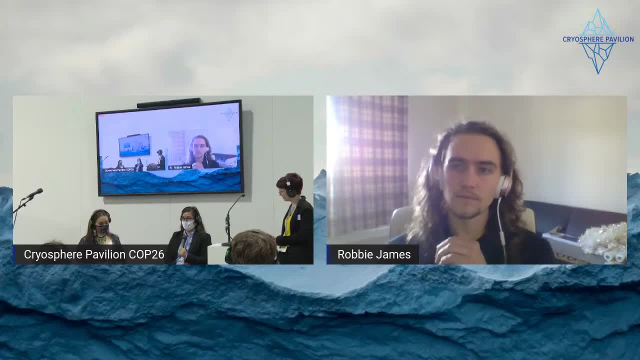 It's all of my elders, It's all of my people, It's our subsistent way of life, It's everybody who I've ever spoken to, every elder, every cousin, Everyone who's going through depression. I mean there's many different factors that permafrost. 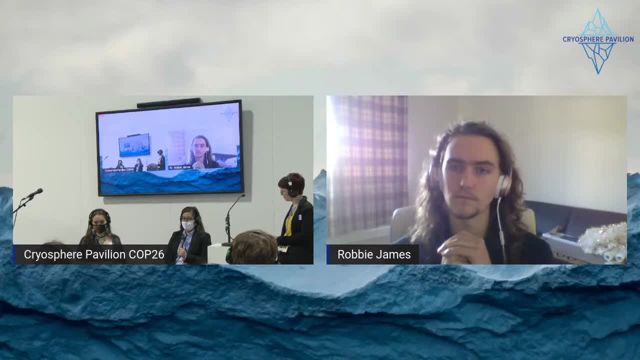 on climate change has on my people, And I recognize that it's a privilege to be here, but it's also very isolating And I'm very grateful to be here, But I don't think I can put it any more beautifully. as Ruth, I think that, yeah, it's a lot on our shoulders And 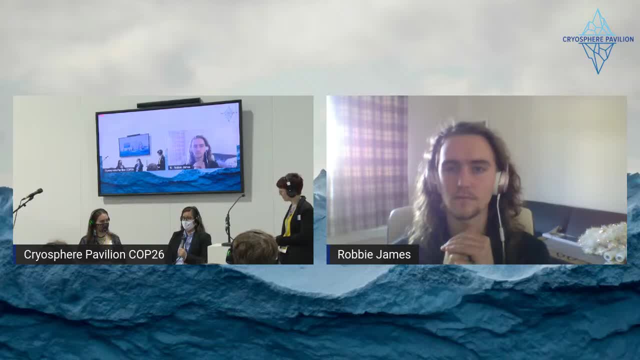 it's really overwhelming. But yeah, I mean, spreading the word is the most that we can do at this point. Not a lot is being done at COP. We all know this, As indigenous people, we know this, So hopefully things change. I don't think. 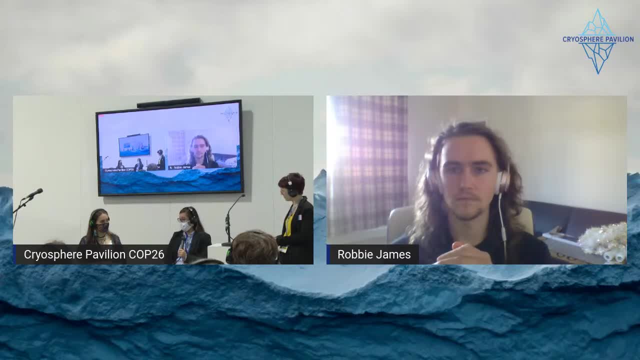 this is where the change happens. I think it happens when we're in line for the bathroom, when we're in line for food. after these talks happen, when we interact with each other. The networking is really what gets the work done, And I'm not networking for myself and 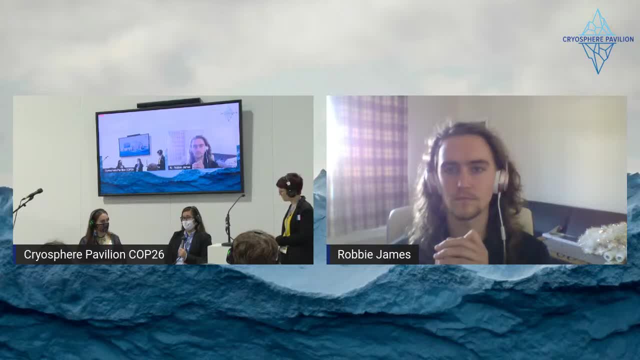 for my organization, I'm networking for everybody who can't be here. Thank you so much for sharing those experiences with us, And I guess I want to pick up on your point, Darcy, about really making change happen and looking forwards And, I guess, thinking. 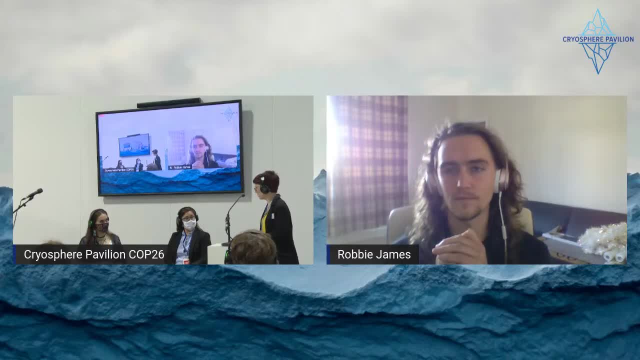 about COP and these processes, but also more broadly. obviously, the three of you are here as young people, as activists and advocates, as scientists, as indigenous youth, And I just would like to hear your thoughts about how do we bring those communities together and work. 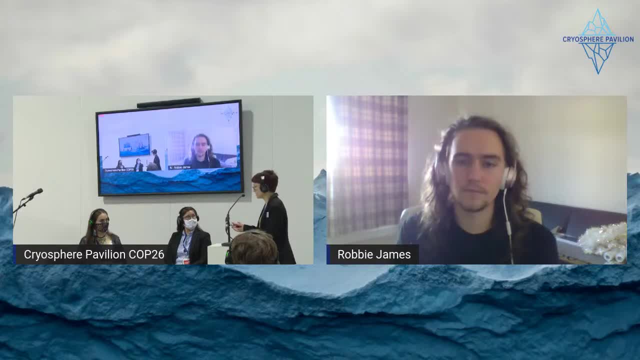 together more effectively, particularly sort of the scientific community, you know who are sort of here. How do we work with those different communities to really support each other and really make that change happen? And I wonder if, maybe, if we could start with Robbie and then maybe we'll. 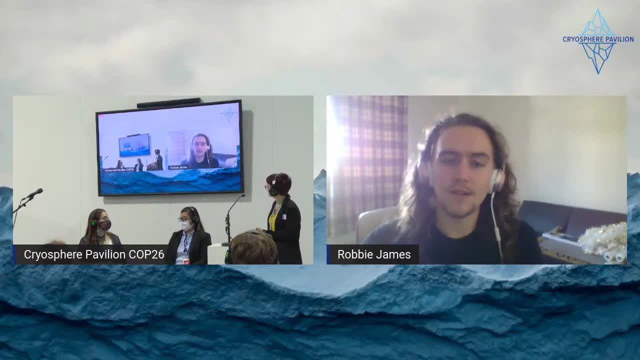 come back to the stage. Yes, I think the most valid voices are those who are the biggest victims, And then so I think having those voices coupled, I mean, in my opinion, with sort of a powerful voice of a scientist, Having those two groups working together, I think would be absolutely invaluable to 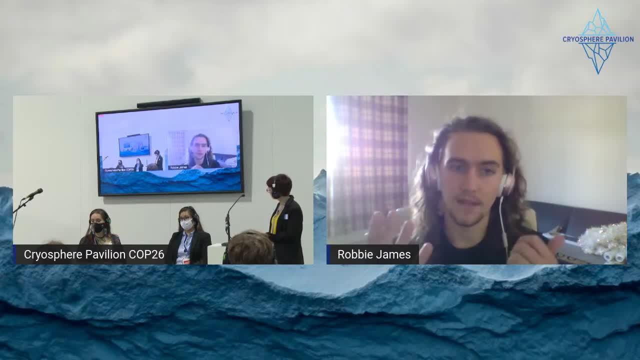 getting the message across. But, yeah, like the youth are obviously going to have to deal with this for longer than everyone else, But then sort of indigenous youth, that's sort of a bit of a double whammy there, really isn't it? 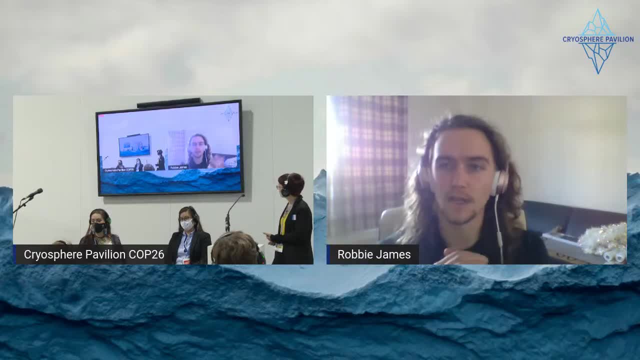 So, yeah, I would say like for scientists to get involved and go out and reach out to these communities and then, if they have any sort of platform, use that platform to amplify those voices. Yeah, I think that would be really, really invaluable. 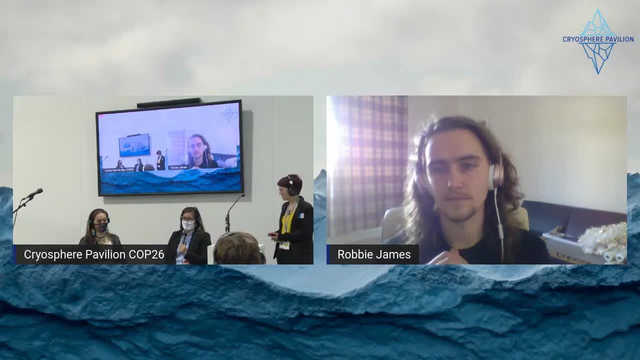 I agree completely. Yeah, so there's no framework in place for how to work with indigenous people as scientists or as engineers, as policymakers, But there are those that exist, depending on which community you're working with or want to work with. So just doing research. 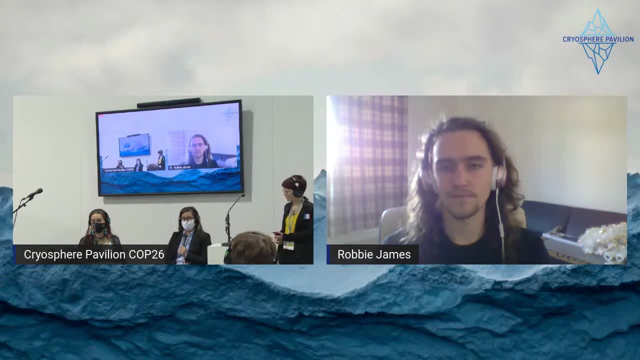 We're all researchers. I mean a lot of us are researchers There's. it just requires simple Google searches like tribe in this area, tribe here, tribe there. like reach out to them, talk with them before you have any grant in, before you have. 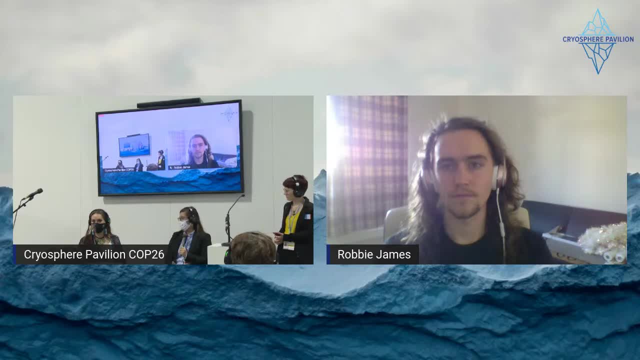 any funding. before you have any money, before you have a plan on what you want to do, Reach out to the place in which you're wanting to work. Talk with the indigenous people there, Work with the tribe, the city, the state. 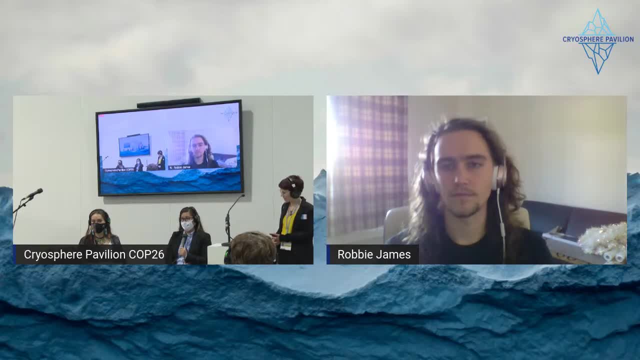 There can be multiple entities in one town and develop a project together. Don't bring I mean similar to what Ruth was saying- like don't have something and bring it into the community, Develop it together. It it should be a symbiotic relationship. 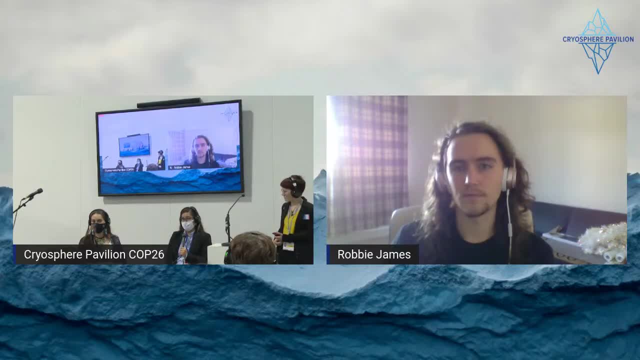 It should benefit the researchers and the indigenous people. I'm a firm believer in the question of what good is research if it only benefits other researchers, especially when it comes to climate change? in the Arctic, I mean, we're experiencing climate change at two, three times the rate as the rest of 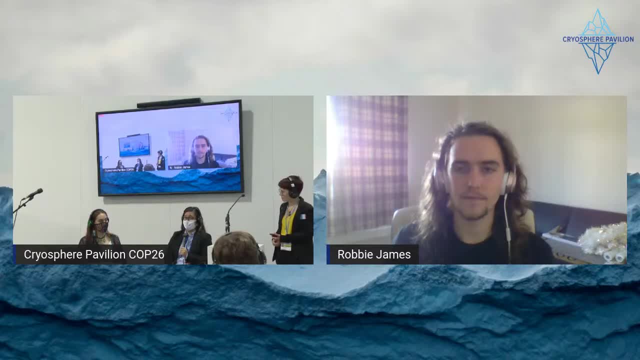 the world. If what was happening in Alaska was happening in New York City, there'd be an uproar and there'd be huge amounts of funding. But since we're in it- We're a predominantly indigenous community state with very small populations- it often 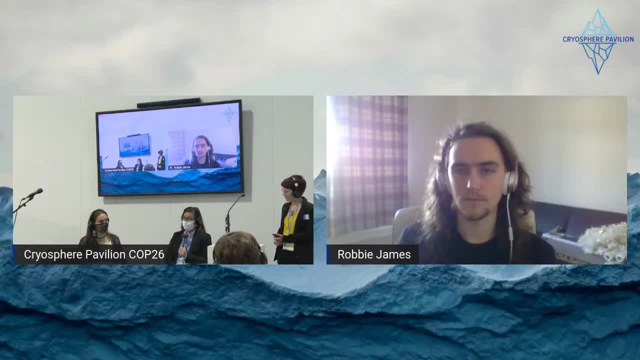 gets overlooked And I don't think that's OK. And I think that scientists can do a much better job working with indigenous people and making sure that their research can benefit somebody, that it can be used in policy to get the tools and resources necessary to indigenous people, to go to policy to really 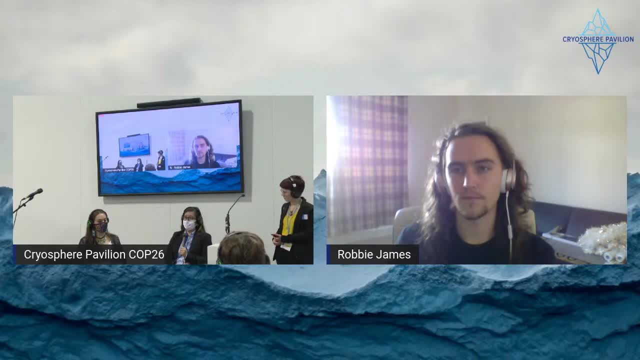 implement change. It doesn't have to be at the international scale, In fact, it probably shouldn't. It should be at the local scale. There's food insecurity, There's infrastructure insecurity, There's a lack of resources across many different venues that are in a community. 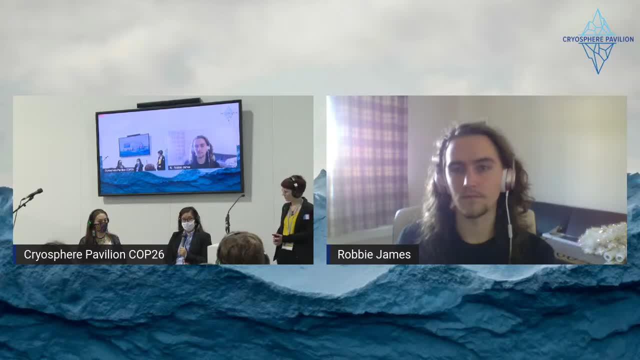 So I just think that researchers and policymakers need to do better with interacting with people, And it requires humility, and it requires a lot of being uncomfortable and being comfortable with being uncomfortable, Absolutely. So so well said, Yeah, Being humble enough to learn from us. 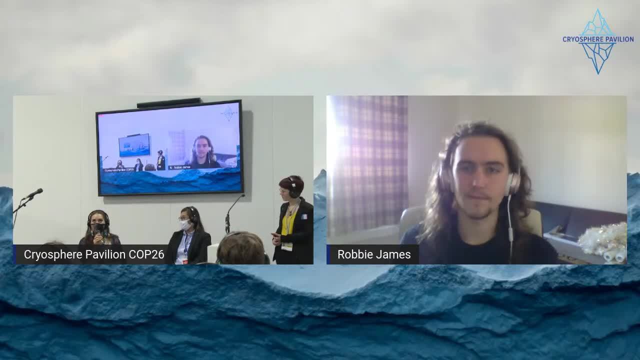 And I think, if I told you know, each of you, or you know the research community, the Western Science community, that that, for instance, our community members, our elders, had been keeping record books of atmospheric pressure, of temperatures, of fish counts, that 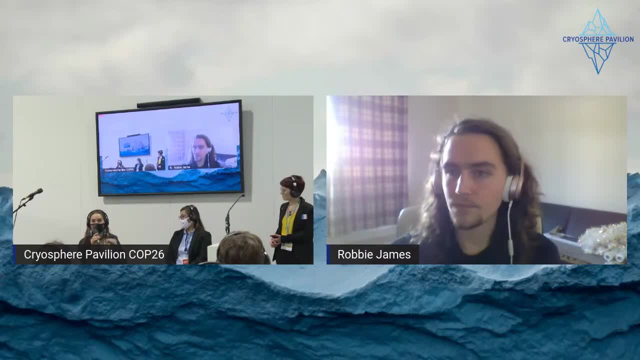 we had data from every month of every year for 10,000 years, that we had biological data and geophysical data, that we we're taking, you know, observation and we were measuring this and that and had written it down, put it in a book, had 10,000 plus years of daily data. The research community would say this is 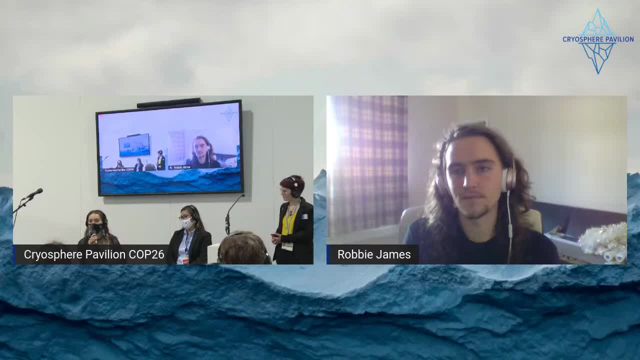 the richest data set in the world. We're so grateful to have it. Look at how much we can learn If I told you that all of that encyclopedic knowledge, that rich data set, was ingrained in our oral histories, our creation stories, our languages. suddenly it becomes invalidated. 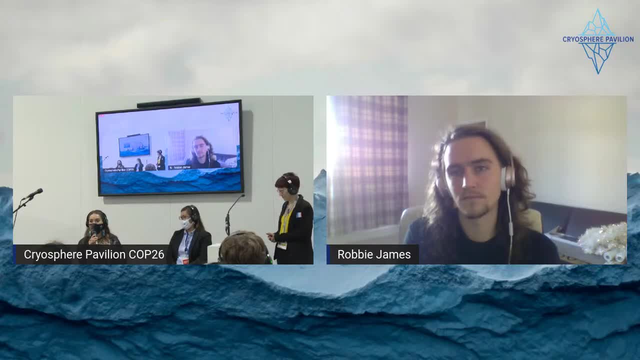 and not valued. We are the world's first climate scientists because we still, to this day, live dependent on our changing climate. Our subsistence communities notice first when our ice flows change, when our salmon counts change, when the places where our berries and edible plants and 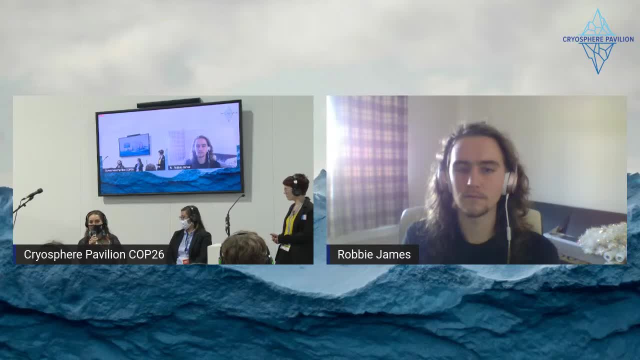 medicinal plants grow- We are the world's first climate scientists, We are the world's first- are growing in different places. when those change- Permafrostas in particular- we are the first to know and we have been recording these changes in our stories, passing them through generations for. 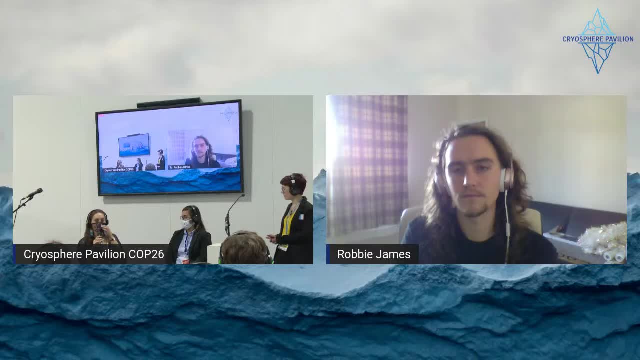 tens of thousands of years. And so I would say: learn that language, validate that science, because we have rich bodies of scientific knowledge. It is just not Western science, which is relatively young, And so by working with Indigenous communities and validating Indigenous knowledge as participatory to climate research, we would see a massive decentralization of Western frames of thinking and would also have the opportunity to learn about how to mobilize and replicate Indigenous ways of being, Indigenous technologies. learning from our first sources, our elders, 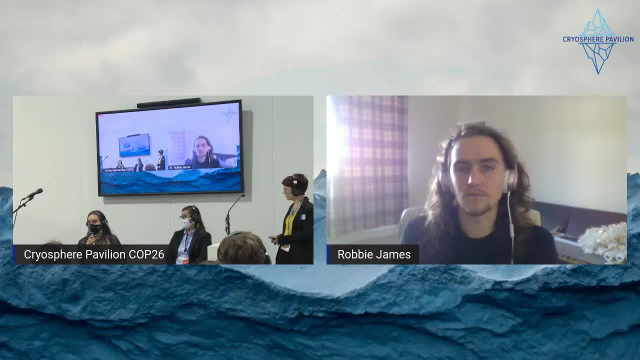 So we already have Indigenous innovations and engineers who are active in our communities, thinking about how to live best with the lands as they change. It is time that you know the Western science research community came to that body of knowledge. Thank you so much And I would love to. I think probably all of us would love to carry on this conversation for so much longer, but I'm a little bit conscious of time. 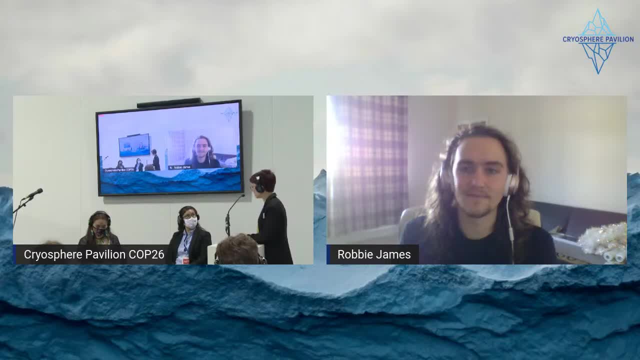 And so I wonder if, perhaps, as a finalist, As a final question, I could ask each of you what is the message that you would most like to be able to share with the policy community here at COP or, failing that, any other last remarks you would like to make? 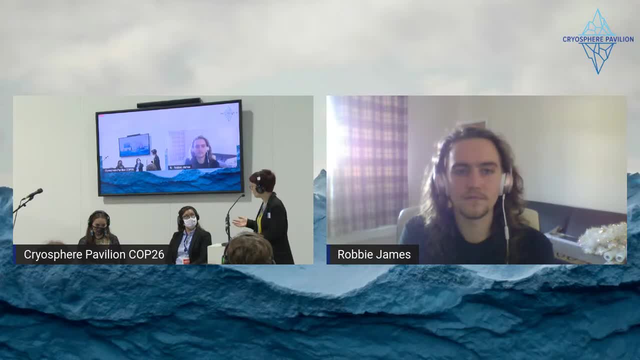 And also if you could add where we can go to follow each of your work and find out more in the future. that would be really helpful as well. There is no way forward for any question, There is no way forward for any question about climate policy- without Indigenous youth engagement, without the engagement of people of color, of frontline communities, local communities, there is no saving anything. 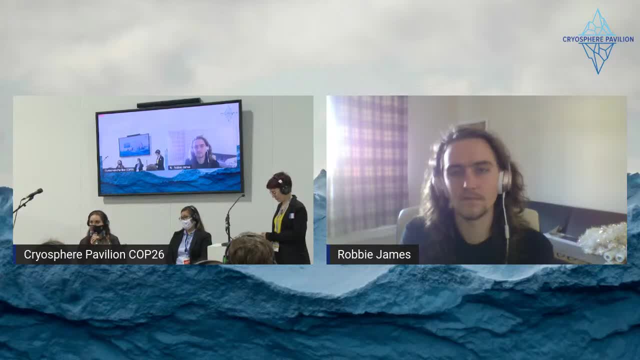 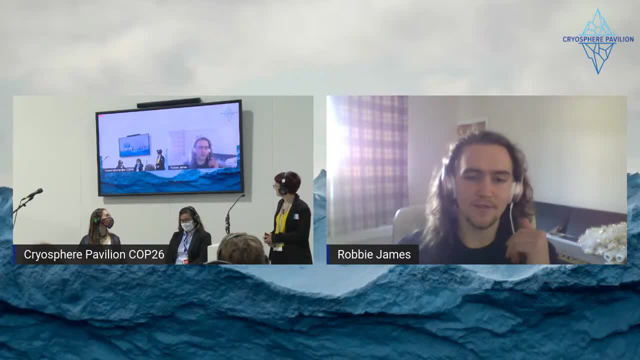 We need a climate recovery to be based in de-colonization. We need a climate recovery to be based in de-colonization. Getting involved with Green New Deal Rising has been a really great opportunity for me to learn, a person coming from a place of, you know, quite extreme privilege. I've been quite 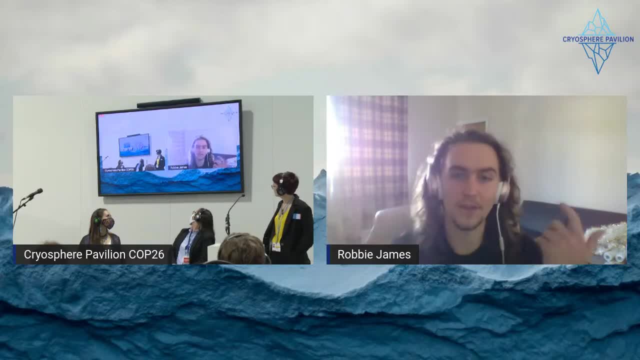 ignorant to these issues a lot, you know growing up, whilst I've been involved and learning about climate change. so I think, like the Green New Deal movement is really good at tying those two things into in together and I'm learning, you know, I'm learning a lot and you know everything. 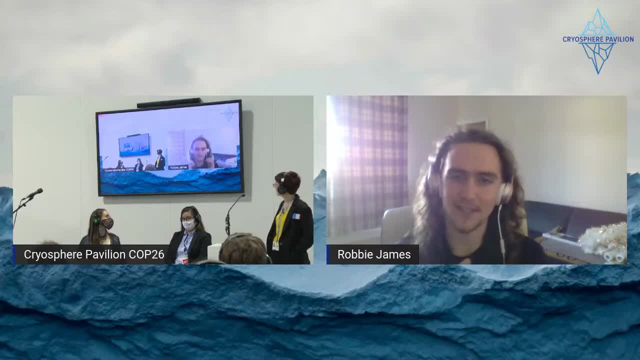 everything that you're saying is like it's so important and I'm really looking forward to learning more about it and getting involved with it as well. Amazing. thank you so much, and I wonder if we perhaps have time for just perhaps one or two quick questions from the floor, and, of course, I'd like to first check if we have any questions online. 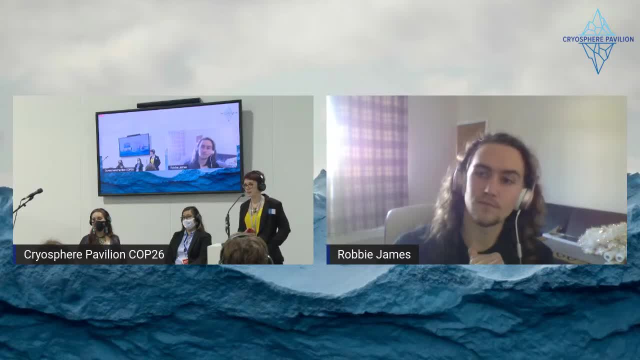 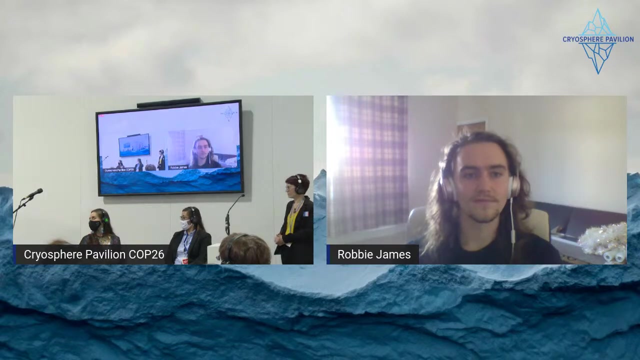 and no, okay, that's fantastic. Does anybody here with us in Glasgow would you like to ask a question? Would you like to come up and speak into the microphone? Thank you for being allowed to ask a question, and I would first like to thank you all for the great 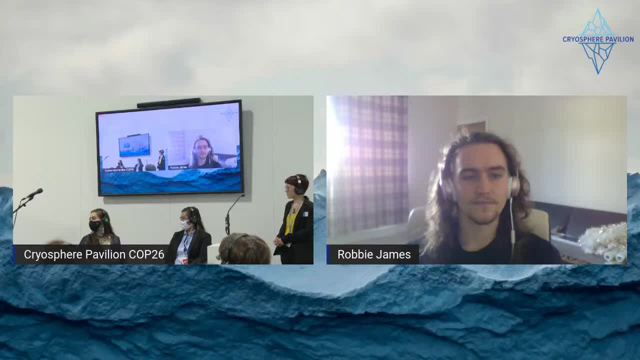 debate we just listened into. My name is Rolf Reven. I'm from the Arctic Monitoring Assessment Programme, one of the Arctic or one of the working groups of the Arctic Council and, as you might know, the Arctic Council. they have both representatives from the Arctic States as well as from permanent. 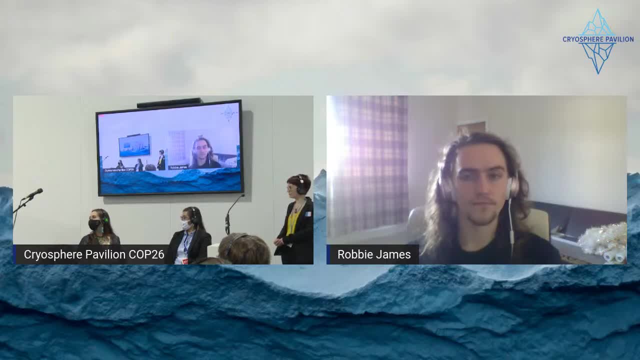 participants or indigenous groups. I'm a member of the Arctic Council and, as you might know, the Arctic Council, they have both representatives from the Arctic States as well as from permanent participants or indigenous groups, And so we do at the working group level with inviting indigenous representatives to our work. 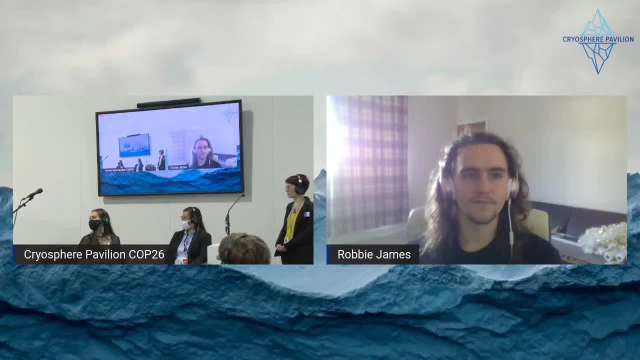 and scientific work. It may not be a question, but more like an encouragement, seen from my side- and I'm both leading the secretariat and being a Sami myself, so I have one foot in both camps. but co-production of knowledge is not only about you know, giving your knowledge to somebody, but it's 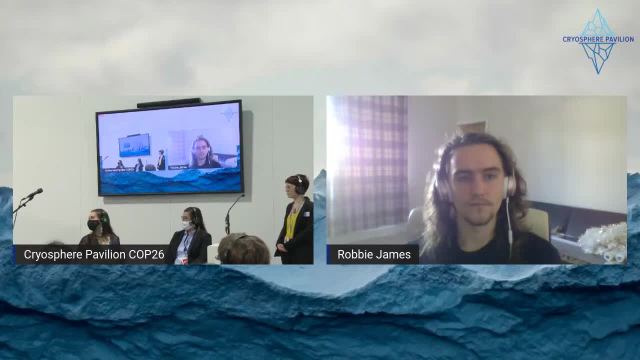 also about developing the process, on how to do so, how to incorporate it into the work that we do. So it's more like an encouragement for you to incorporate those, those knowledges, and making making it to more than just one plus one. So so my encouragement for you is more like: or what we find challenging is also to try to identify. 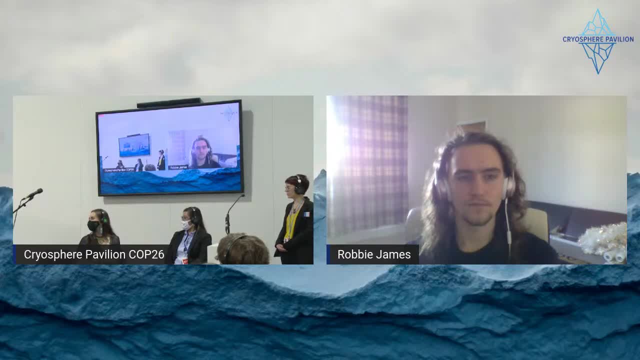 the good knowledge holders, to try to identify the right level of engagement and how to to approach those. So so it's also more like an encouragement from from our side for to invite you to reach out to us, to the scientific um, scientific society And and also, like we would like to, we would like to take part in this. we would like to take part in. 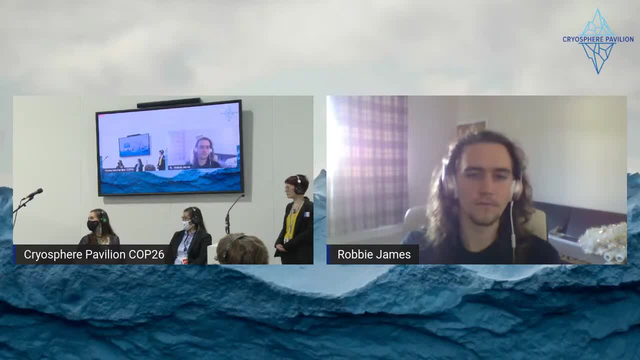 your next climate report. This is what we can bring into this and this is how we can work together so and and in that way, try to also help develop the, the learning process, in particular now when we see a, a system like an arctic system, um, where we kind of move into our, towards the boundaries of what 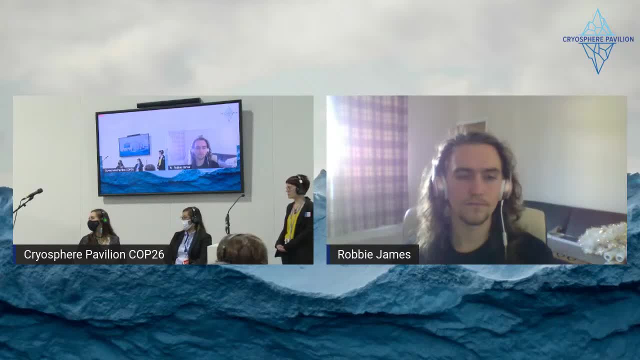 we know We're, we're about to move into the unknown of processes and, and I think it's even more valuable then to to try to combine those knowledges and understand what's actually going on on both on the regional scale, but also on the local scale, as you you say here. so thanks a lot again. 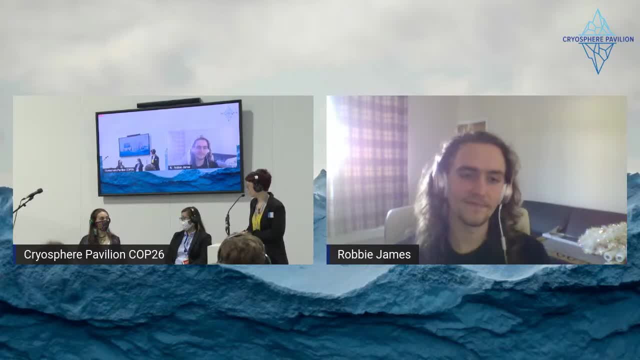 Um, would either of you uh like to respond or are we happy to? I'm happy to make time for other questions. we definitely. we do work closely with Arctic Council on indigenous people And one of the real points of entry is the creation of permanent youth participants to the Arctic Council through the Secretariat. 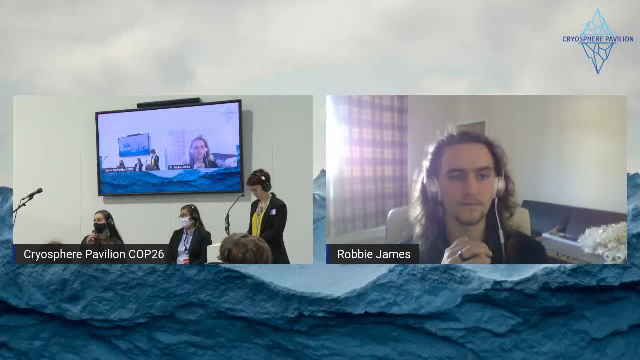 And further expanding those opportunities for engagement is so important. However, the Arctic Council is a distinct body from the United Nations processes and even the definitions of who belongs in the term Arctic shift between these two parties. And so by complicating this, by bringing in more communities, by expanding opportunities for engagement and by publicizing them, it's not only putting the labor on indigenous peoples to come find you and to come contribute to you. 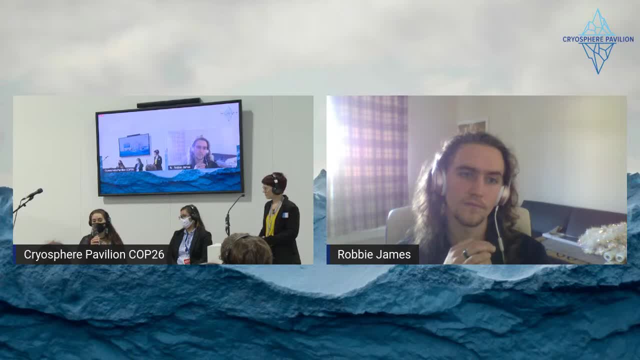 It is by cultivating deep relationship. Thank you so much. Do we possibly have one super quick? Yes, OK, Hi, I'm Tenzin Shiki. I'm senior researcher at Tibet Watch and I was really, really pleased to hear such critical voices that have been pushing for justice as language that the Tibetans themselves have really struggled to push at international platform. 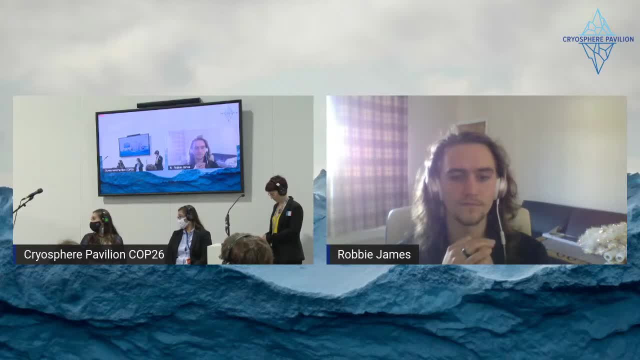 but have been an increasingly isolating experience, because you know the fact that Tibet was colonized by China. When Tibetan delegations come and speak about, everyone is just shying away from discussing the fact, about colonization and the fact that now manufacturing industries are just, you know, dominated by China. 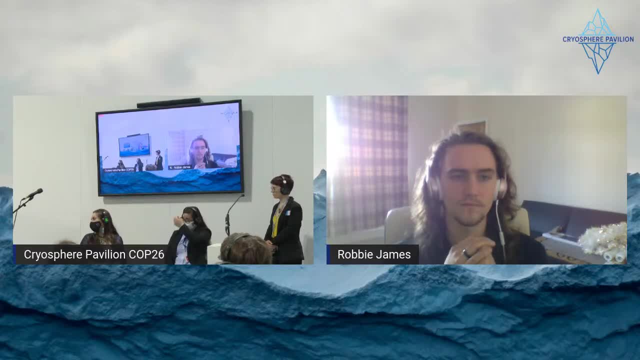 So, as you were saying about you know really facing difficult questions about colonization, capitalism and scientists who are also trying to publish, researchers have to really include frontline communities at every level of political decision making and checking the with indigenous communities and local communities and oppressed people how they can really build research towards an empathetic understanding of justice. 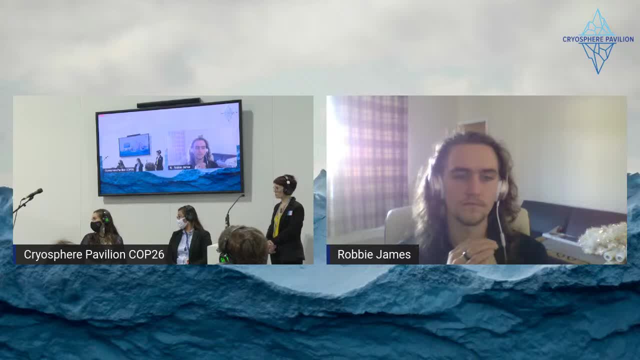 And one of the things I thought to share is just again in terms of, you know, permafrost. So I think there is a lack of understanding about the scale of the Tibetan plateau, which is two point five million square kilometers and about two percent of the land surface area. 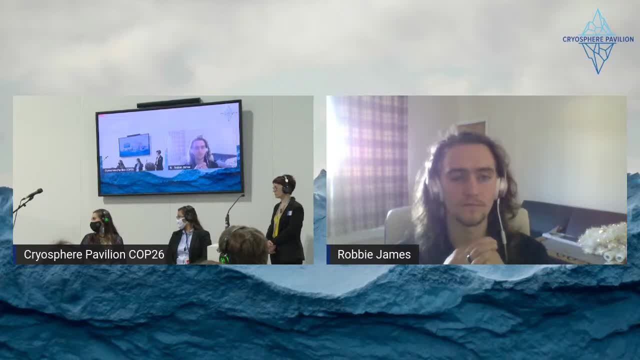 And just as the The previous scientists spoke about how difficult it is to understand what's going on under the ground, and also you know what's going to. it's a complete flux of change. But you know, as I'm really always happy, when we speak our own language, to embed our knowledge in just one word. 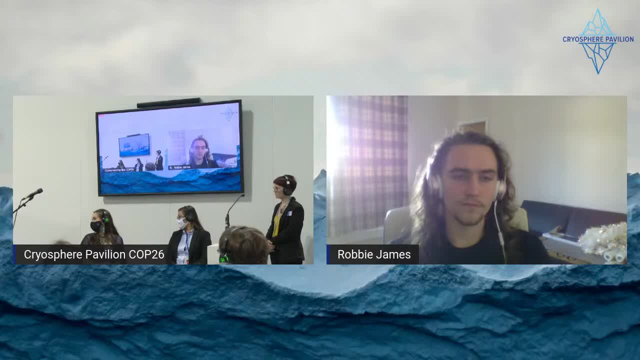 And you know Tibetans have this word, Kawa, which is like domain of ice, or, And then you see that they are poets, So also call themselves like like there's one poet can get to wake up, which means snow born to wake up and the people identify themselves with the land and that land is degrading. 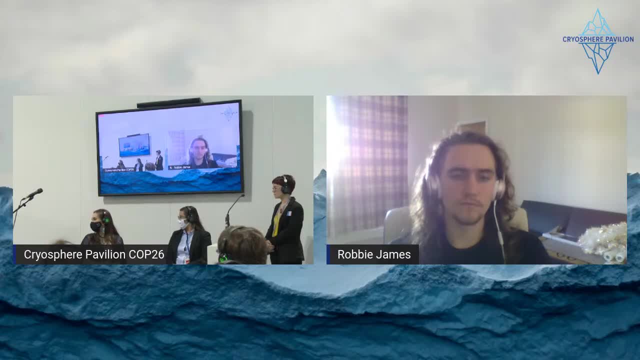 And then as a senior researcher at Tibet Watch, we monitor facts of human human rights violations inside Tibet, And now we have received information that in Ushua, Tibet Autonomous Prefecture, now people have been confiscated of their grassland use certificates, Previously being guaranteed as 50 years. 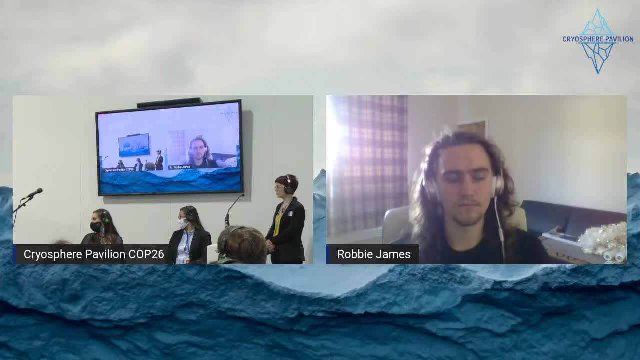 But then now they have just confiscated And now these people who we cannot name are saying that you know they feel like the state is really trying to centralize them and keep them under check, And I think that you know we need these critical discussions and we're really happy that we are here to shift that in a way of framework where you know discussions of, you know power of who's. 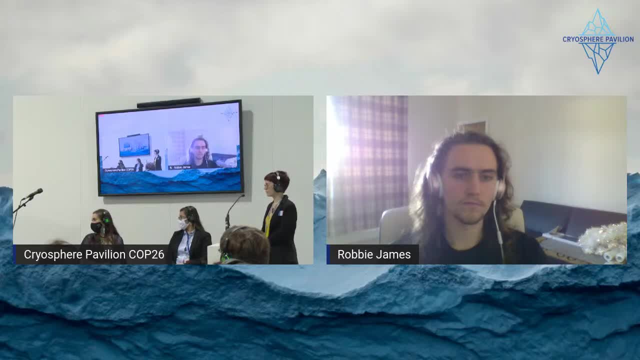 Gets to speak about what science is? who gets to speak up? the politics are really addressed and, yeah, I'm really happy to speak afterwards. Thank you, I wish we had a third chair. I feel like you should be up here with us. 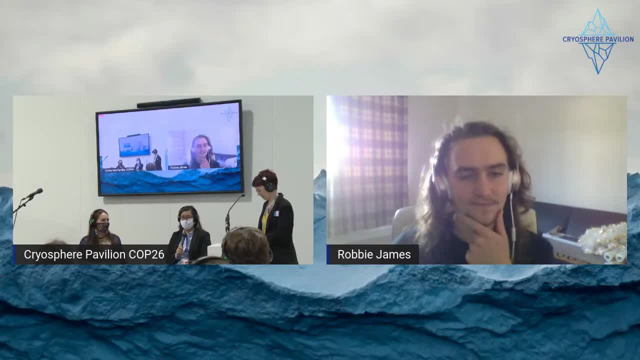 Yeah, Thank you so much for your comment. Yeah, I, I would love to speak after as well. Thank you, Thank you All of you. I think we we should probably wrap up, because our next event will be starting in five minutes and that one is focused on fire and permafrost.